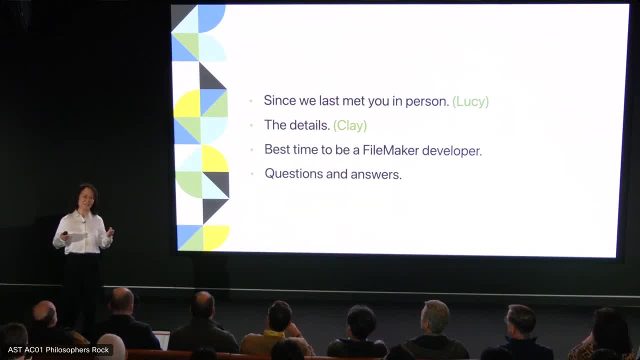 What you do as FileMaker developer is amazing. As problem solvers, you transform ideas, use your imagination to bring FileMaker to new heights. We want to help you to go even further. So we are delivering the best, the most powerful FileMaker we have ever built. It is the best. 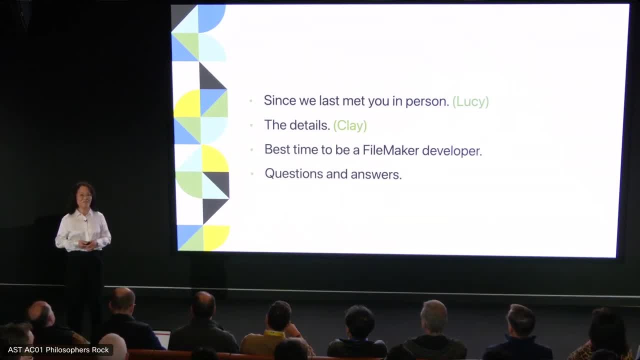 time to be a FileMaker developer. And finally we'll have some Q&A time, also from FileMaker engineering team for this conference. Thank you is Connor Brock, FileMaker Team. Scrum Master Clay is not here. He's at the booth duty. 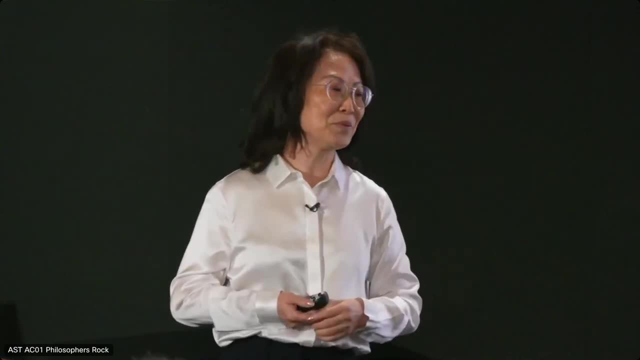 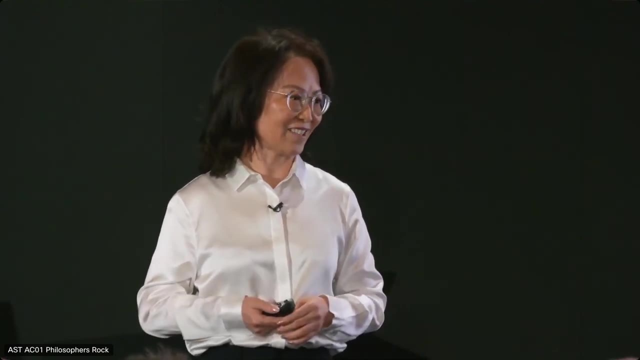 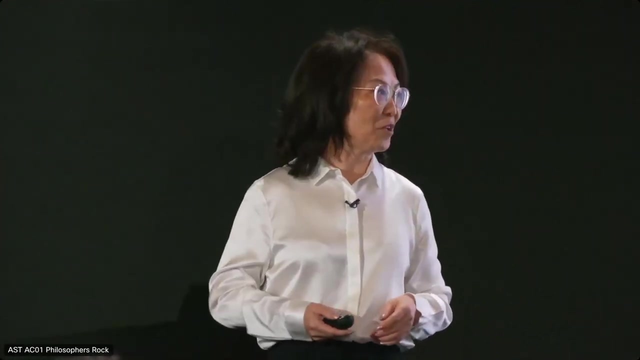 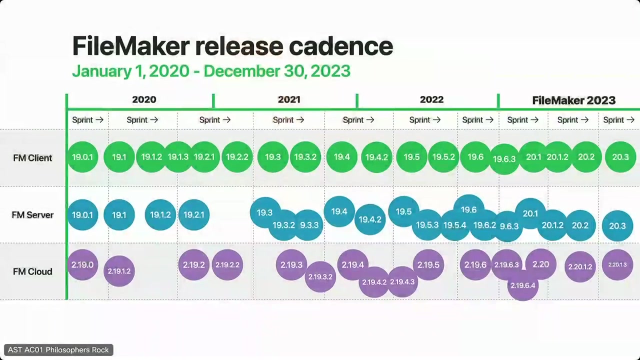 Wade is not here. He's at the booth duty. He's the FileMaker Senior Server Dev Manager and Architect, And we also have PM Rip here. All right, Let's start with FileMaker updates. This is the FileMaker release cadence since we last met in person. 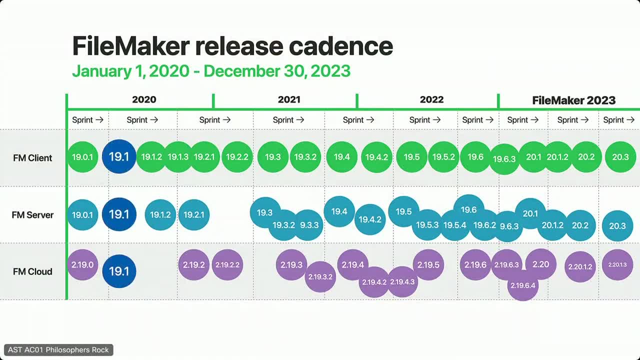 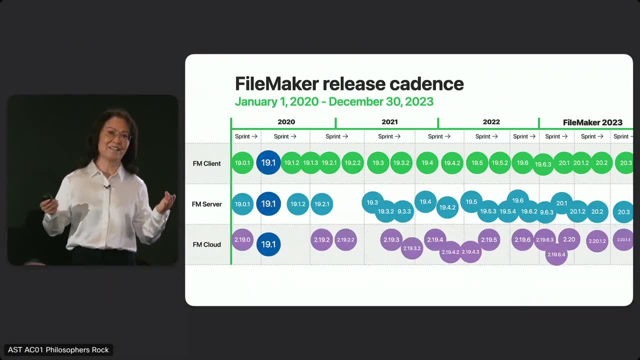 From 19.1, we transformed into Agile, releasing features, bug fixes as they are ready, regardless of major or minor versions. After 19.6, we advanced to 20.1 and named it FileMaker. Now ETS of FileMaker 2024 is available. 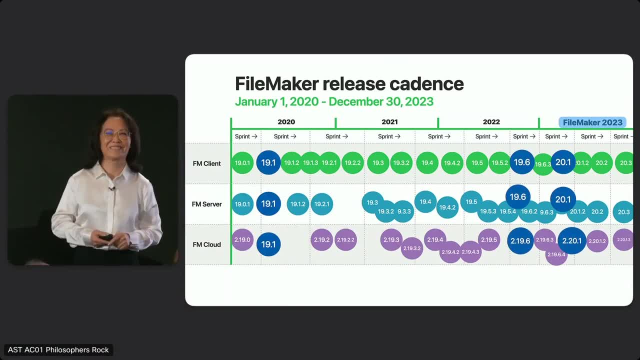 Rick pushed the button yesterday, So we invite you to join the ETS program because we love your feedback, We want your feedback And we really listen to your feedback And we support your feedback, Thank you. Thank you for taking the time to spend time, digest it and categorize it and transform into engineering actionable items. 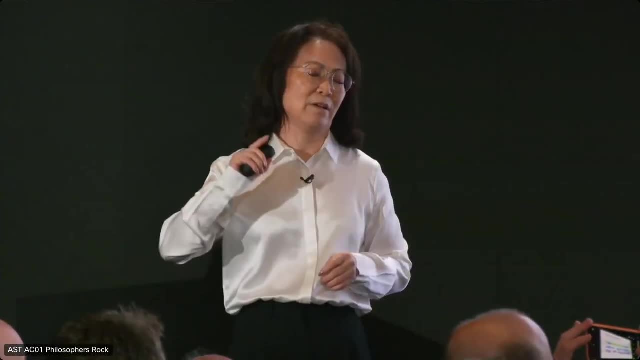 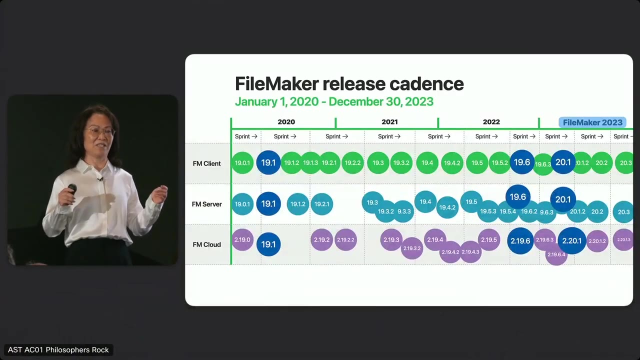 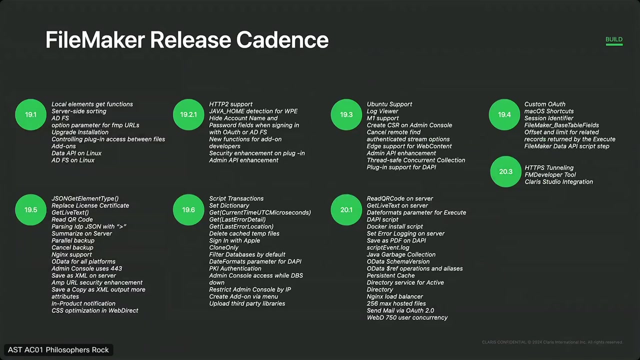 One bug at a time, One feature at a time, One enhancement at a time. I am delighted to say we figured out a customer feedback loop to do what matters to you the most, And here they are. Thank you for your tremendous support for the feature list that you asked. 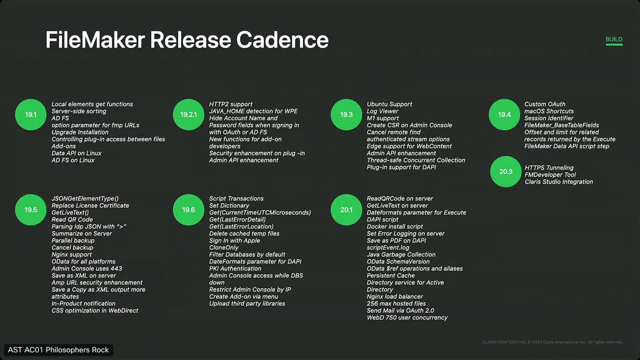 I know Klaus asked a lot, Vince asked. thank you, I encourage you to ask for it- And then the validation of several thousands of bug fixes through these process. Thank you very much. These bug fixes are the secret sauce for your smooth operation. 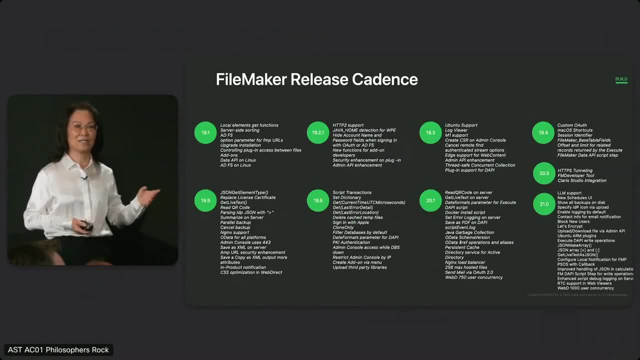 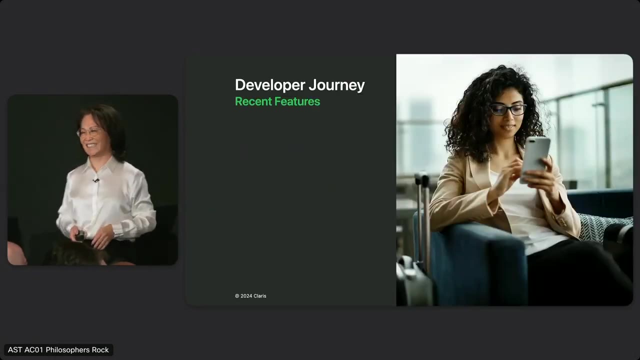 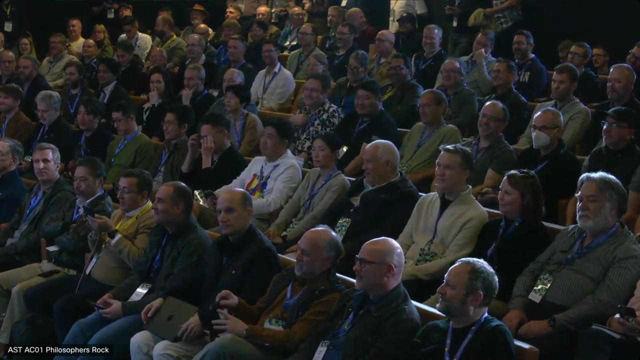 Now the ETS for the next release: List of features and preview of LLM support. That's all in the ETS. Take a look, All right. So let me take you through the ETS. Let me take you through a developer journey and discuss some of the recent features and enhancement. 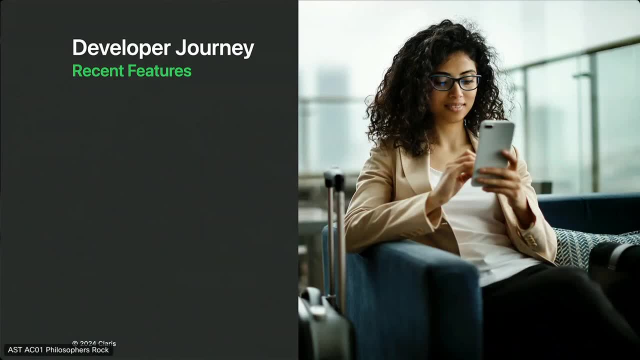 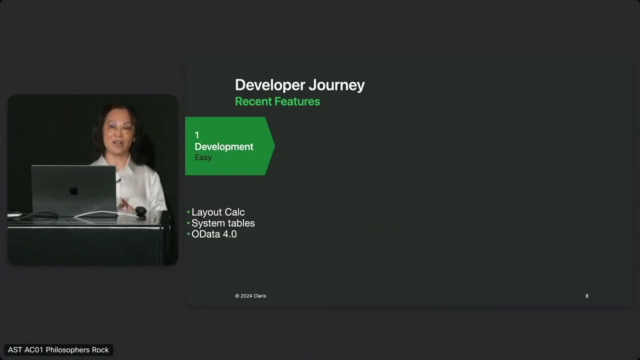 Paula is an experienced FileMaker developer. She works on FileMaker CRM solution for a high-end bike shop. The shop depends on FileMaker solutions to stay connected with customers and streamline internal processes and improve profitability. The bike shop's employees dashboard needs to be dynamic and informative. 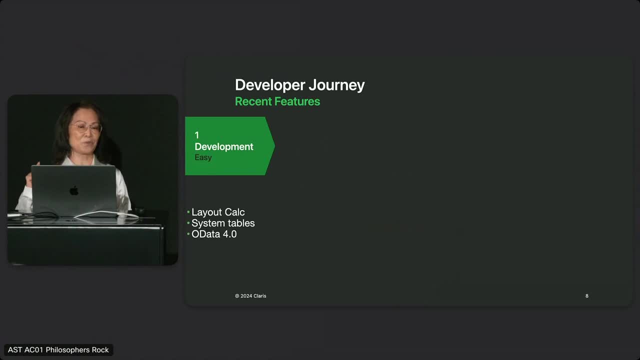 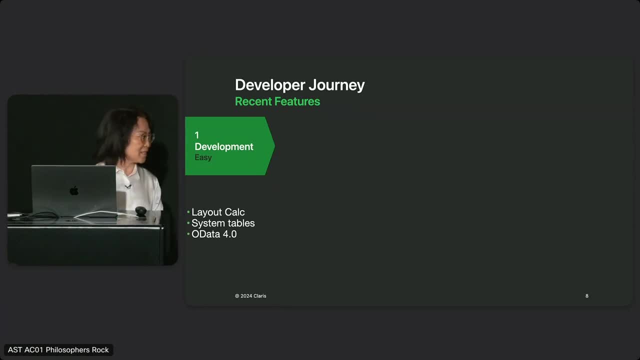 Let's get started. So Paula shortens the development time and use system tables to get schema information of the FileMaker solution and use OData 4.0 to modify record relationships. How about data integrity? Customer information, their bikes and the service details span multiple tables. 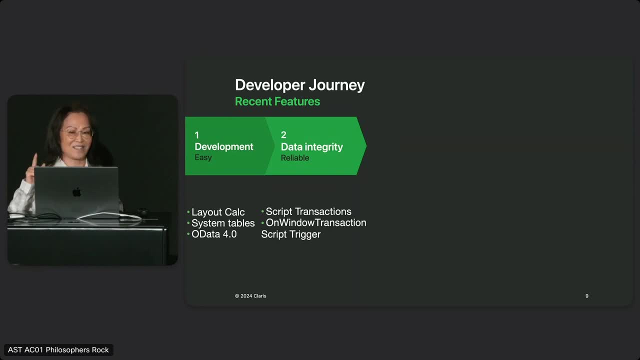 Paula uses script transaction To ensure data entry meets the quality standard, and if she needs to track down who changed a record, all she has to do is look at the audit log that she configured with on-window transaction script trigger. The feature script transaction allows developers to group multiple changes according to business rules. 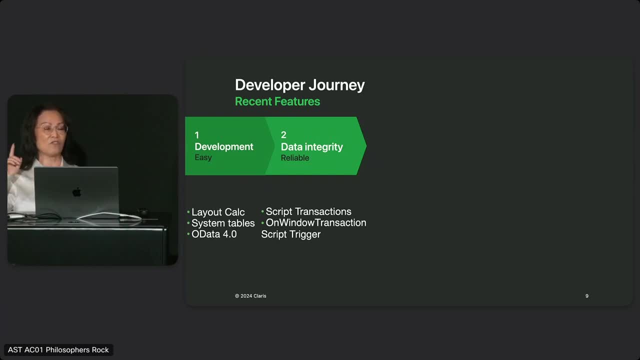 Ada should only use data entry based data, like an empty box of decor and pigmentized machines, Data entry Ads, Data entry. Data entry, Data entry and reliability. Here is what Paula did for integration. She made it simple for bike shop. 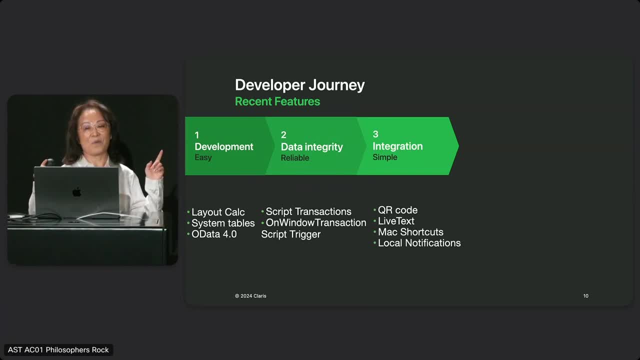 staff to use FileMaker solution with diverse job responsibilities in mind. Their service staff can scan bike parts with QR code. It is simple and accurate. Live text is used to generate reports on converted text for repair documents. Inventory manager can approve orders through iOS and macOS shortcuts. We integrated live text on macOS and iOS and QR code for Mac Windows. 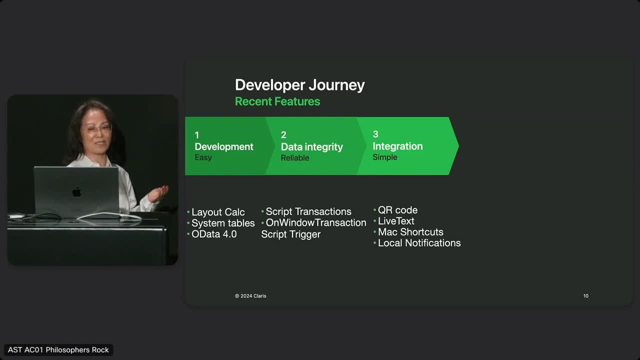 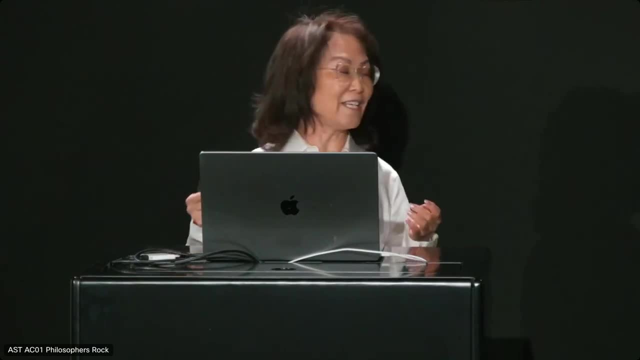 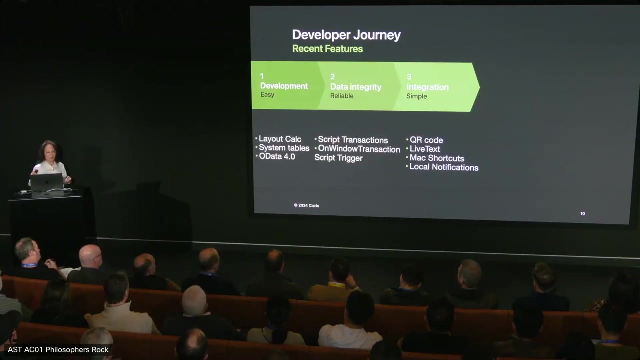 and Ubuntu. macOS and iOS shortcut can open existing exciting integration possibilities. So the next release, Paula can leverage local notification on macOS, iOS and Windows. How does Paula use server-side script to debug and troubleshoot? So analyzing data from repair shop is a heavy task. Paula sends those operations to the server asynchronously. 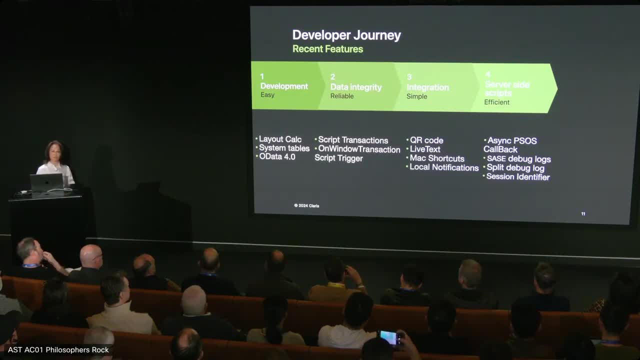 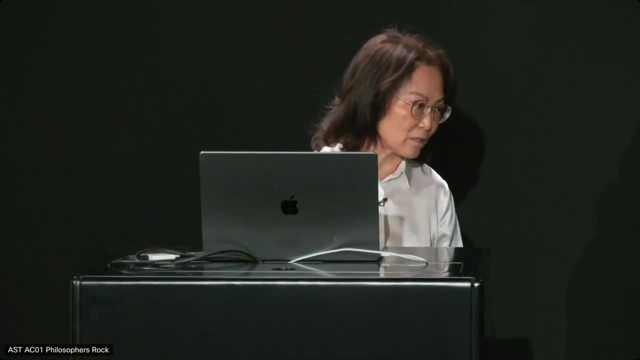 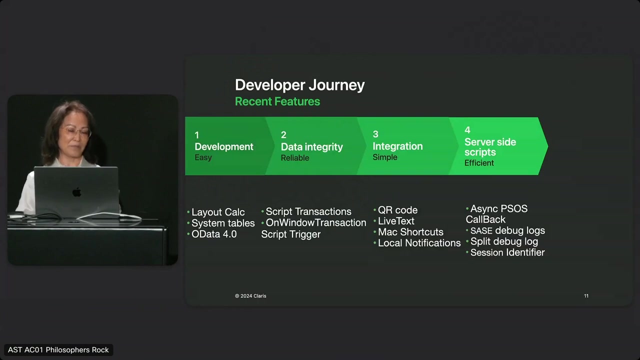 so her users can continue their tasks. P-Source is a popular tool for pro and go to execute scripts on the server. MetaScript Server мож server side script to simplify debugging. It is easy to find the script error because they are split into separate log. 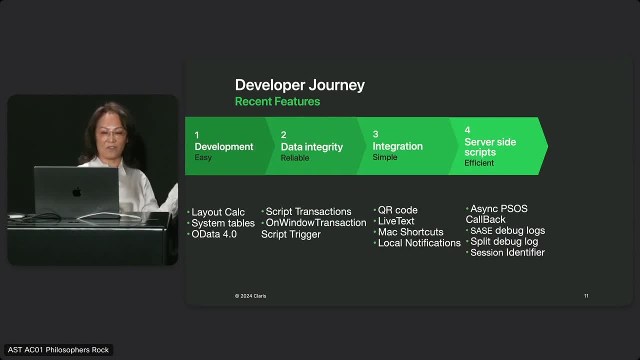 Setting a session identifier for the script, Paula can identify exactly the user who sent the work to the server For deployment. Paula's final touches are to encrypt the file and remove admin access. Thanks to developer tool, Paula can integrate that into her automation flow. 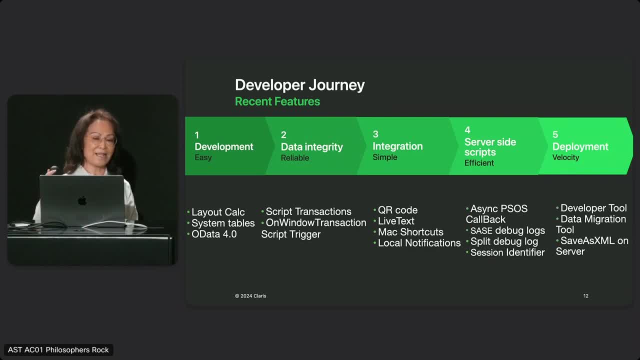 With the data migration tool. she then upgrade the production version of the file After the bike shop begins using the production. using the solution in production, she continues to make enhancements and keep track of development and using the schema as XML after each update. 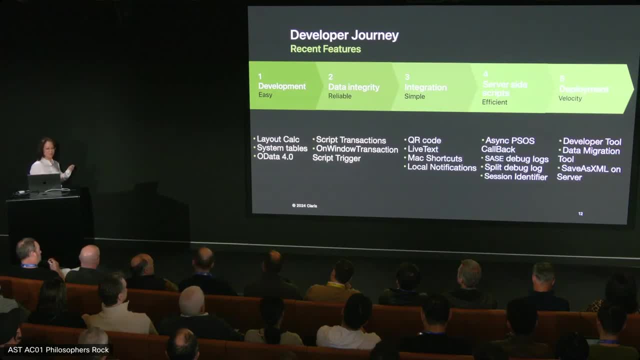 Save a copy, as XML is fast when performed on server For bike shop. it's a big job every week. By automating this, it saves hours a week and many in a year. To Paula, a FileMaker developer, these features made it easy for her. 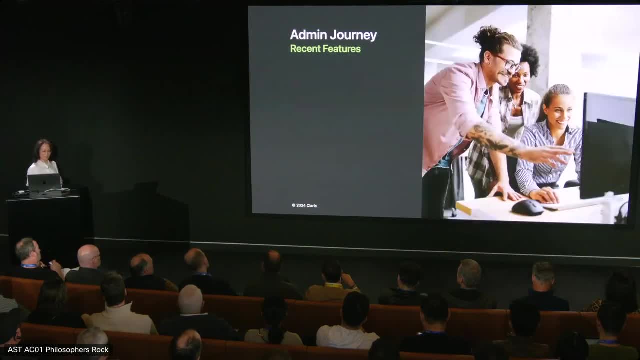 It's time To go into production. Let me take you through a FileMaker admin journey. Our goal is to empower admin to keep FileMaker solutions running well, safe and available to whoever needs them. Alex is an IT manager for the bike shop. 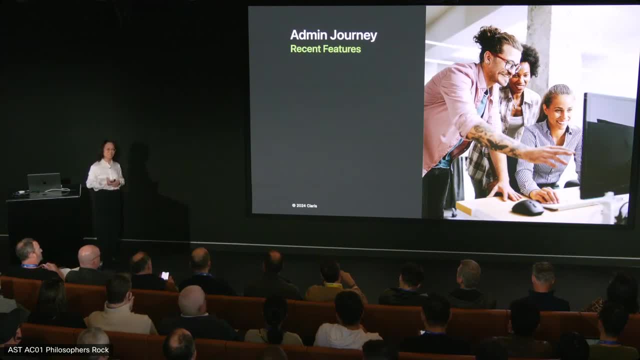 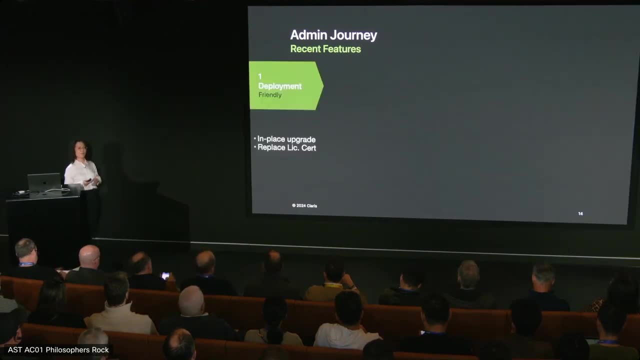 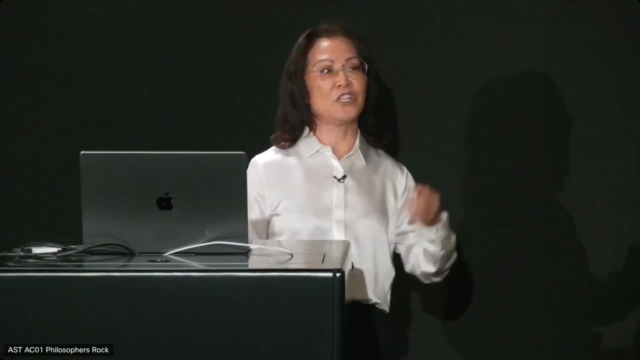 He manages and runs FileMaker production servers. He handles deployment efficiency and security For deployment. Alex can perform in-place upgrade directly from FileMaker server 16 all the way up to FileMaker 19.x, 20.x and even the new version that we will release in the future. 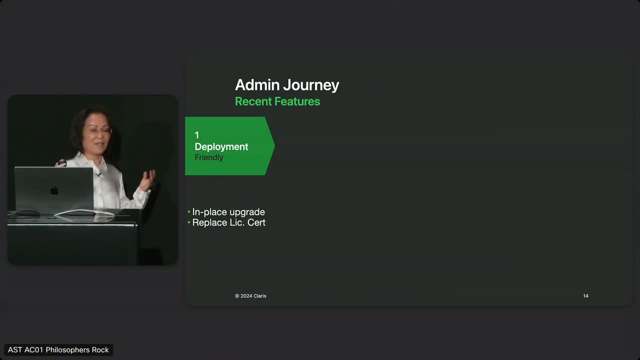 Alex can upgrade. update the new license certificate. view the menu. no longer need to reinstall FileMaker Pro. We continue to improve user experience. for deployment Capacity, FileMaker server can host up 256 files, now up from 125.. Admin role now allows each member accesses their own file. 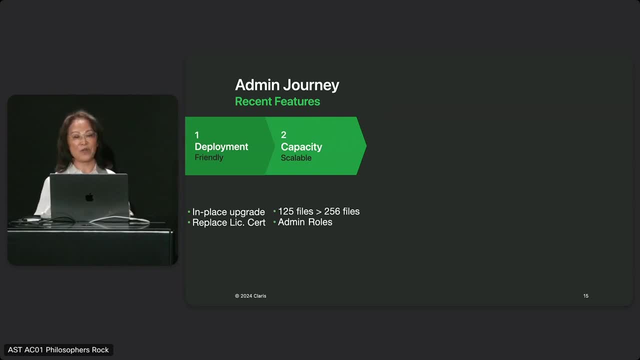 handle file business capacity for action- motives, taste, activity and receptivity of their clients of their own file. handle their own tasks. When you have multiple FileMaker solutions in a single FileMaker server, you can cut cost, simplify management and improve resource allocation. 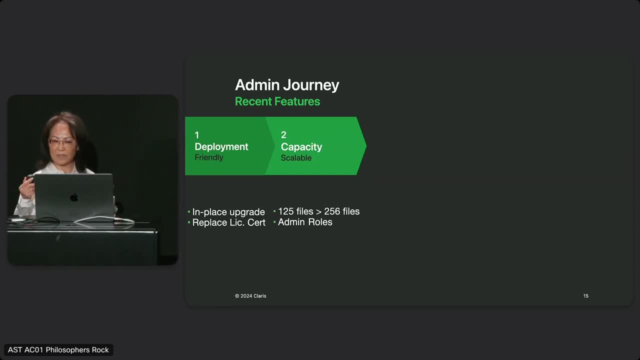 This is very beneficial for solution bundle agreement for our partners who host solutions- multiple solutions- for their customers. For backup, each solution's file set is backed up in its own threads. in parallel backup Alex can set backup schedule to create backup with clone-only option. He can cancel backup cleanly without affecting data integrity. Safeguarding your data is vital to us And backup is more manageable For connectivity. some network admin cannot open port 5003.. They now can use port 443 with HTTPS WebSocket tunneling on Ubuntu 22.. 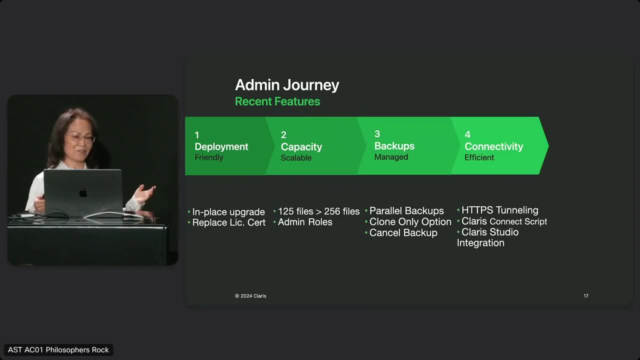 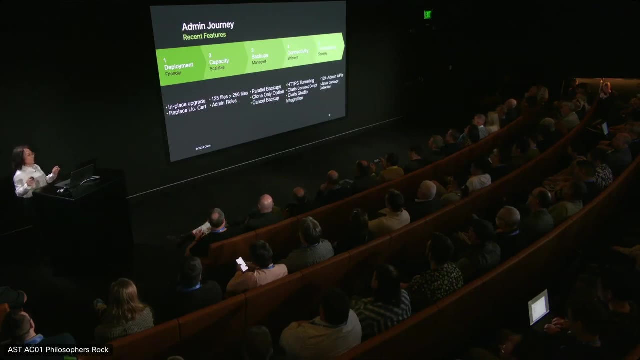 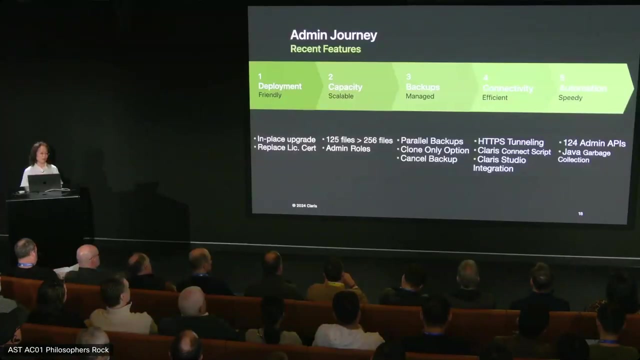 Claris Connect can link FileMaker with other apps. FileMaker is integrated with Claris Studio. FileMaker's environment is more adaptable For automation. Alex can implement speedy automation with 124 admin APIs and more on the way. He can schedule web direct garbage collection to optimize Java memory usage. 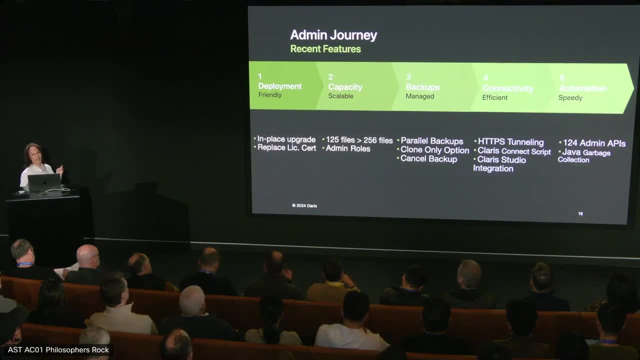 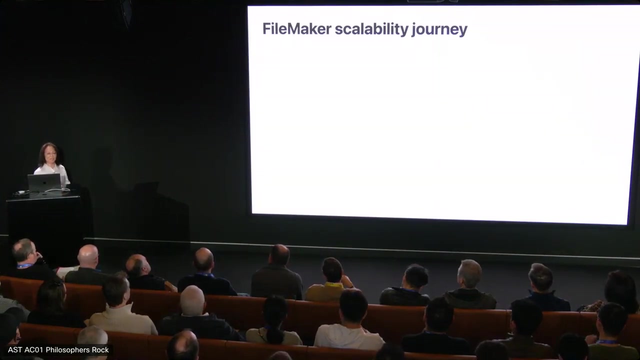 FileMaker allows admin to work smart. We empower admin to keep FileMaker solutions running well, safe for whoever needs them. all right, how about the FileMaker scalability journey? when it comes to scalability, there are two things in mind: scale up and scale out. scale up for FileMaker server means 150 connections, and scale out means adding secondary servers to manage the load. the benefit for scale up is to ensure quality, uninterrupted connections, and the benefit for scale out is to support large number of connections for different kind of company sizes. there we go. this chart is about tested concurrent connections. 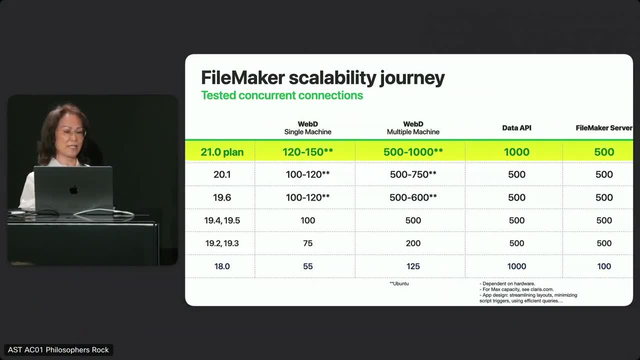 WebDE reached a thousand concurrent connections in the upcoming 2024 release. behind this chart we put extensive, consistent engineering effort to reach to that 21.0 level. we know that every solution is unique. performance and scalability depends on the network hardware and your solution design. 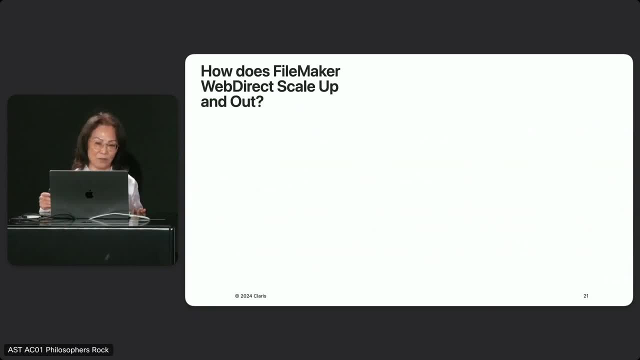 so how does WebDE scale up and out? let me walk through. walk you through the steps. one, you set up a FileMaker primary server. second, you configure secondary servers with three VMs run each to four. each can run three to four docker instances. And then you install NGINX plus. 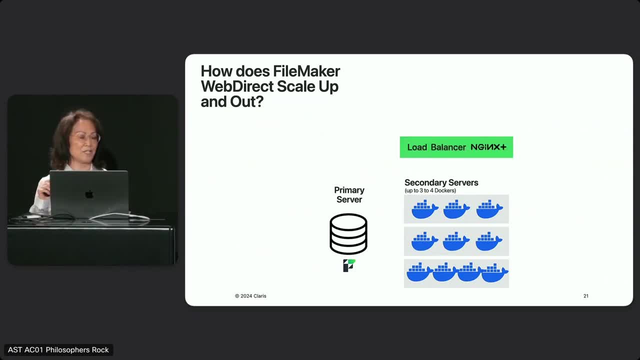 As load balancer in the DMZ zone to distribute the concurrent connections across the 10 secondary servers. Both primary server and secondary servers stay behind the whole framework. we started to build the library to match the configuration of the server, the two firewalls, and we optimize the primary server to only handle database. 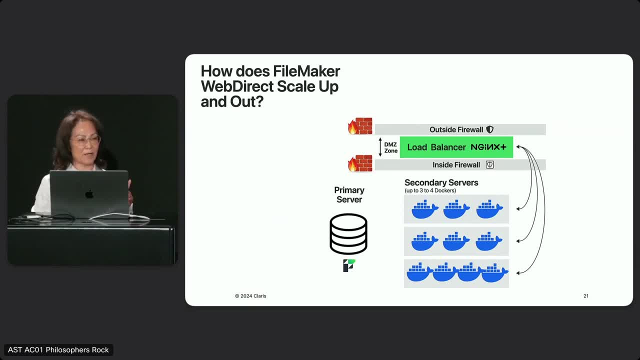 services. it does not handle WebD requests. it does not perform load balancing. this result is to improve performance, simplify management and enhance security. so we enhanced WebD with four layer CS. there we go: four layer CSS layout cache architecture for better performance. we improved threads with non blocking threads between components, so there's no delays. 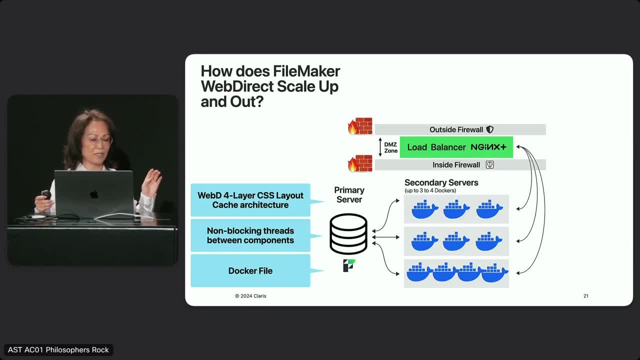 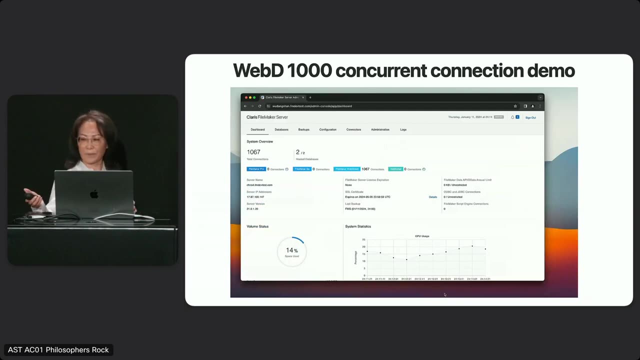 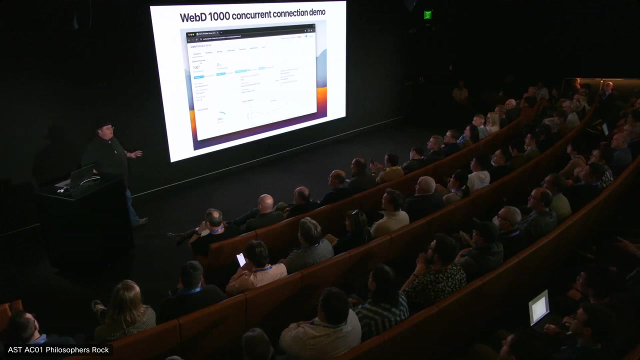 everything can go. at the same time, we provided a docker file to manage those secondary servers. this is how WebD scaled out to a thousand concurrent connections. let me have clay walk you through the demo, howdy. yeah, yeah. this is a demo movie of WebDirect reaching over a thousand concurrent users. with the future version, 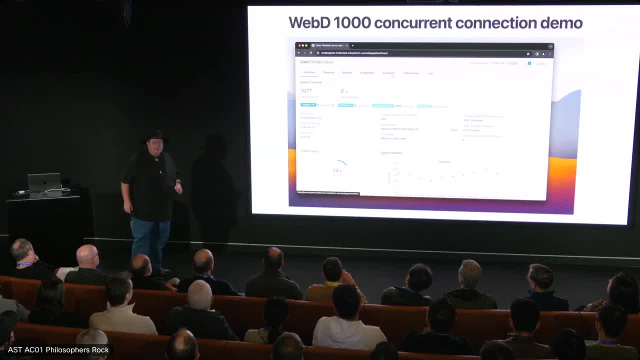 of FileMaker Pro server and this is being tested by our Beijing QA team. the hardware configuration is the primary server, with WebDirect turned off. you can see that the server is now connected to the server and the server is now connected to the server. and the server is now connected to the server. 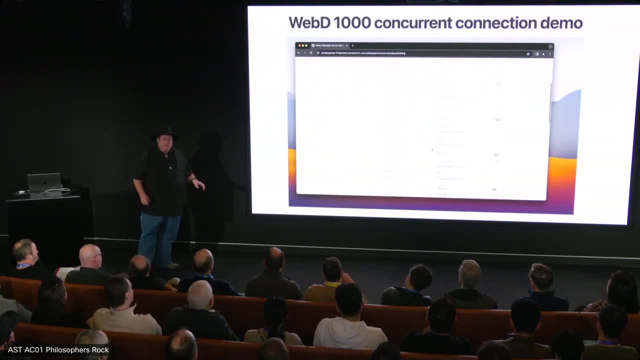 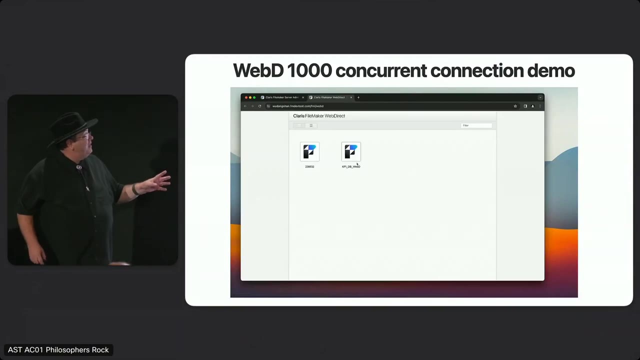 engine X plus the load balancer, 10 configurated running secondary servers- they're right, they're running- are bound to 22 with 8 gigabyte for Intel codes, 8 gigabytes of RAM and currently all the other clients are distributed over these 10 servers running right now. now we're going to have a ad hoc user logging into 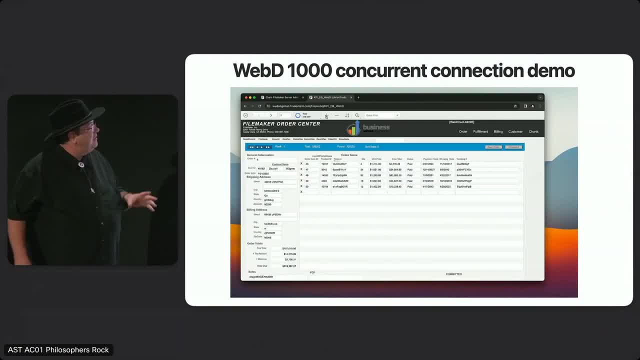 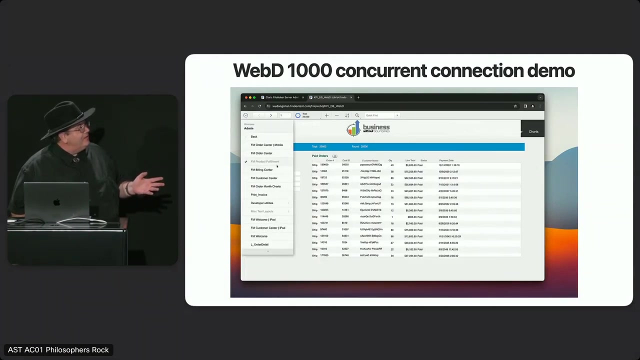 this solution. you'll notice that we have a 15 second idle time, so this user is going through and just doing random operations while all the other clients are doing all these other tasks- they're creating sales orders, doing reports, paying, getting shipping costs, fulfilling orders- and notice that the the user operations of this one ad hoc user going in here is. 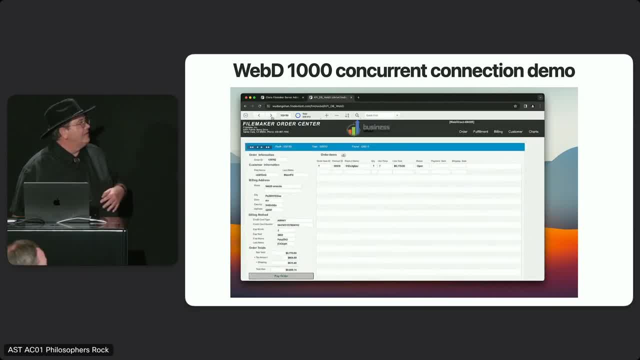 not really being delayed in any way. you see, I'm adding records, deleting records, making changes, and things are working quite well with a thousand- I think it said a thousand sixty seven- ones running during these tests: the operating systems performance metrics and the file maker server metrics like cache hits. 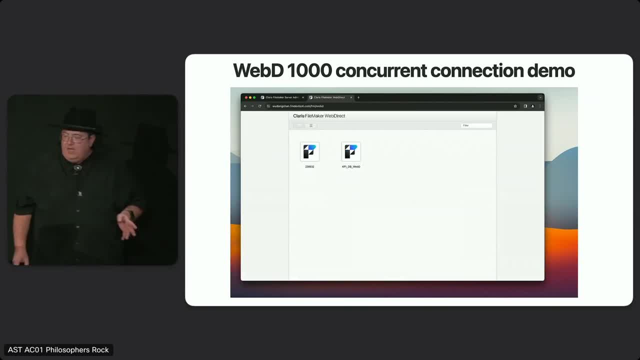 and remote procedure calls are all being recorded and they're used to make a baseline for when we do future versions of file maker server and then we compare them, see whether the changes you made were an improvement or not. so this is one of the ways we're improving file maker performance and I will go back to Lucy. 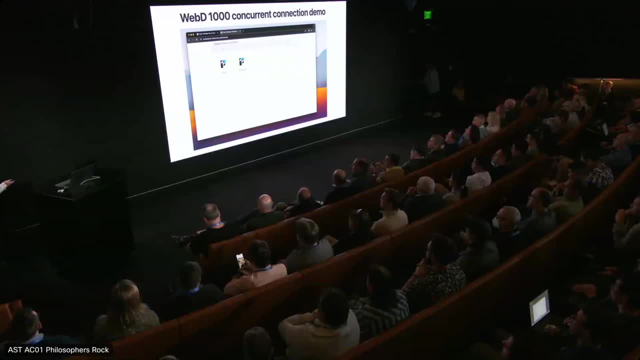 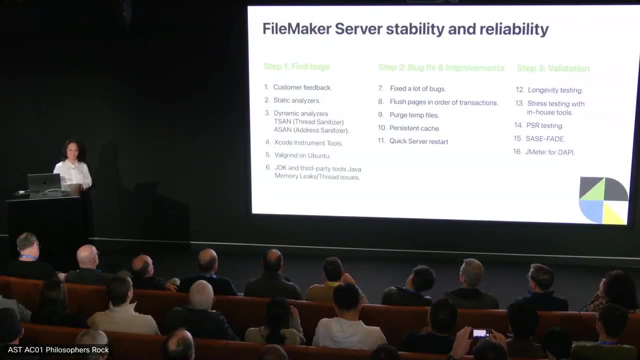 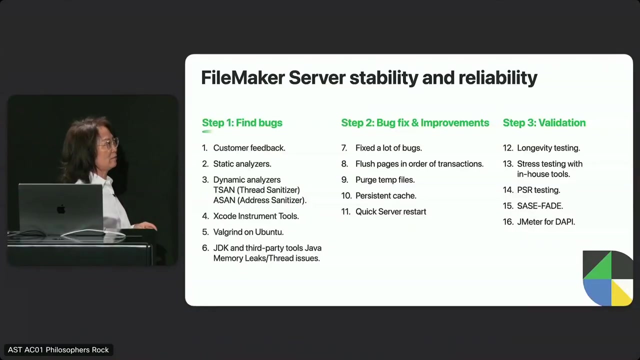 there. thank you, clay, and it's exciting to see a thousand conclusions. and I'm going to go back to Lucy. thank you, clay, and it's exciting to see a thousand conclusions. current connections: how about file maker stability and reliability. this is the three steps in our agile iteration process. number one: find bugs. how do we? 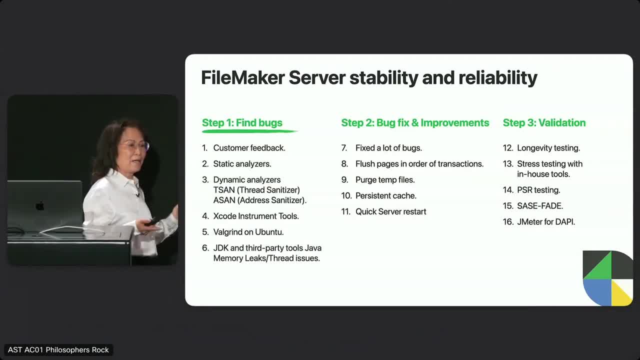 find the bugs. customer feedback. we want your feedback. send us the bugs, it's very important. we want to hear from you then. internally, we run static analyzer and dynamic analyzer with tools like t-san, a-san to do stress test to find bugs. t-san is threat sanitizer, a-san is. 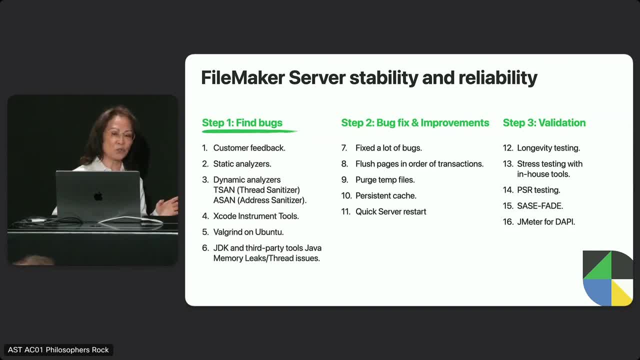 address sanitizer. we use Xcode tool instrument to find slowdowns and memory leaks on Mac and well-ground on Ubuntu. for WebD, we use Java, uh developer kit and third-party tools to find Java memory leaks and threats issues, finding and reproducing these bugs. I want to tell you in scalability. 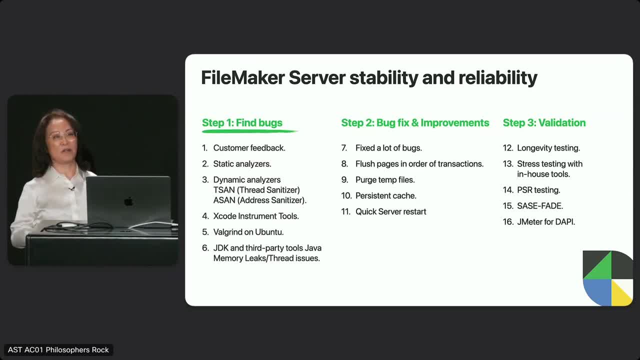 reliability takes a huge amount of effort and time, so we leverage these analyzers and tools to find bugs. of course, a lot of your health and your help as well. then number two, what we do is to fix bug and make the improvement. clay is going to the detail about features I want to talk about highlight. persistent cache. persistent cache protects your file maker files from corrupting. it minimizes the transaction loss in situations like abnormal, normal server termination or force kill. Your solution: stay in a consistent stage with persistent cache. then admin server can restart the server again with very little loss, minimum downtime. 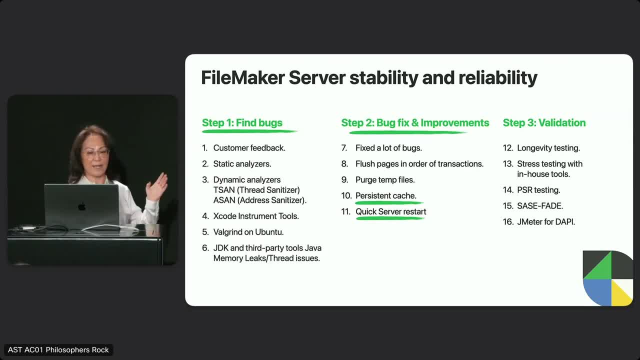 We regress these bug fixes and go back to step one if we need to before we hit step three. Step three for validation. we've set the server longevity testing criteria to two weeks. street Server must run consistently for two weeks, no exceptions, for every certification. 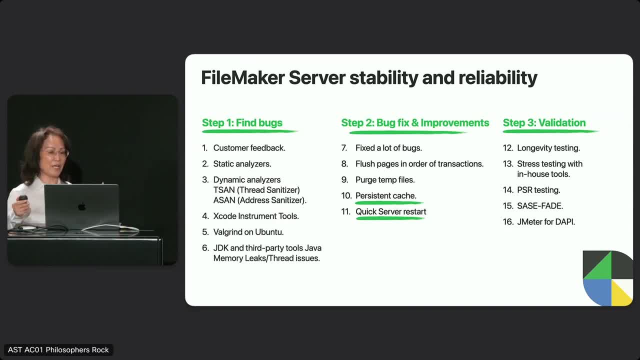 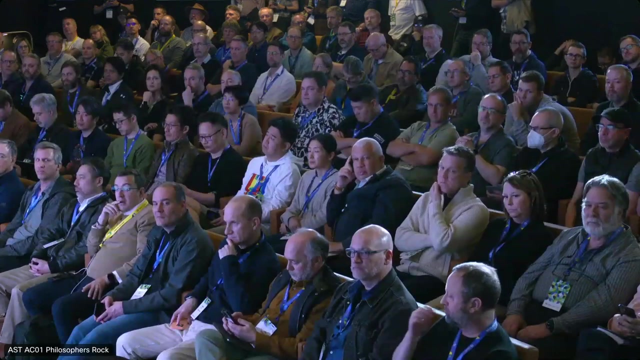 We run stress test with in-house tools: benchmark PSR testing against the previous releases, safety performance tests with Sassy Fade, Apache JMeter test for data API. We work with a core group of customers. I see Vincent Klaus there today. 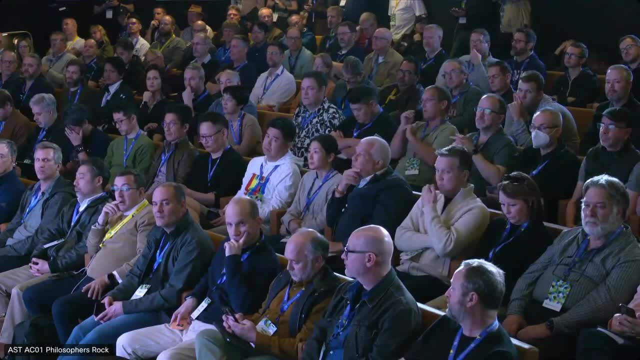 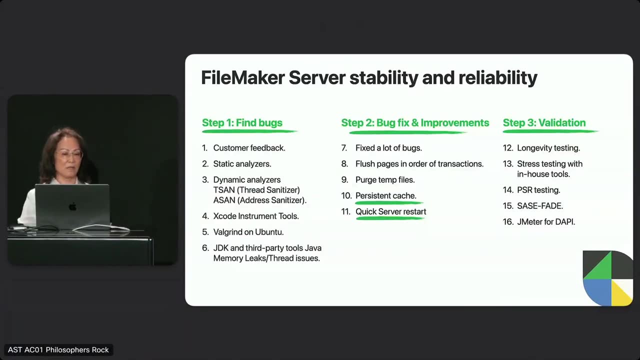 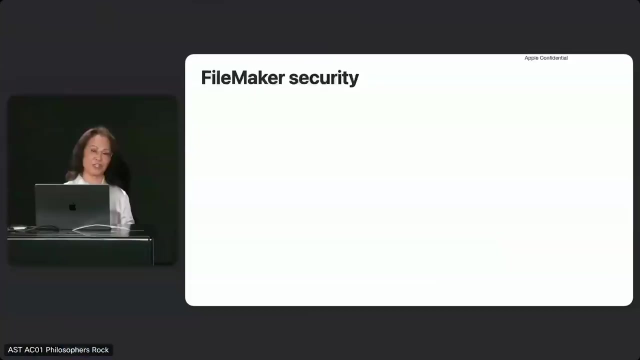 So we also work with a lot of other folks very closely. We call them ring zero customers. Together we made FileMaker safer and more reliable. So thank you, ring zero customers For security. FileMaker is more secure with hundreds of safety measures and bug fixes. 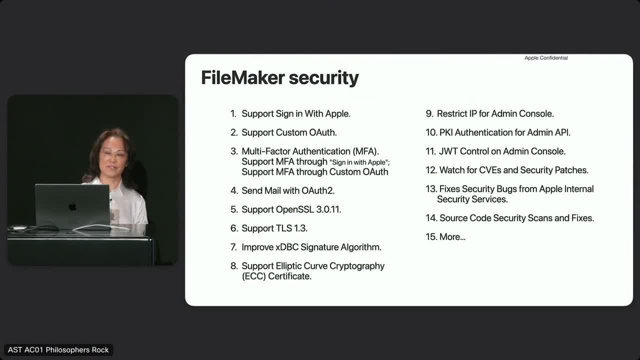 I have examples. First, FileMaker solution can use custom OAuth or sign in with Apple and you can use it to create a new system. Second, you can use multi-factor authentication through these sign-in services. Please enable MFA whenever possible. 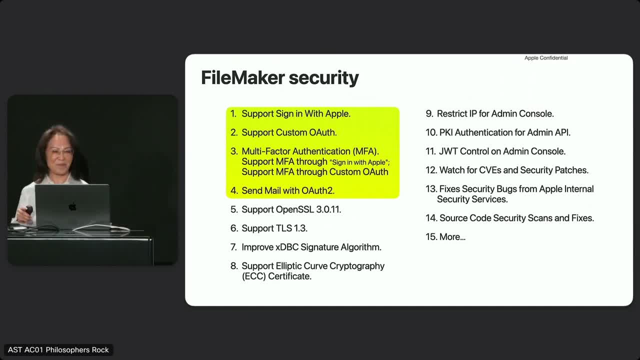 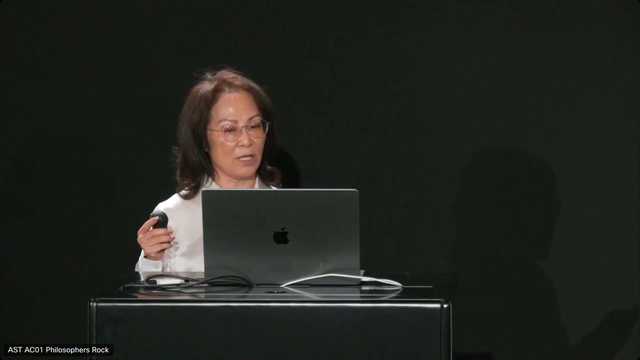 We implemented thank you. we implemented SendMail with OAuth 2 for Office 365 and Gmail. We made signing in more convenient by adding login services for you. Next, we upgraded FileMaker. Next, we upgraded FileMaker. Next, we upgraded FileMaker to open SSL 3.0.11 for Mac, Windows, Ubuntu, to improve security and better performance. 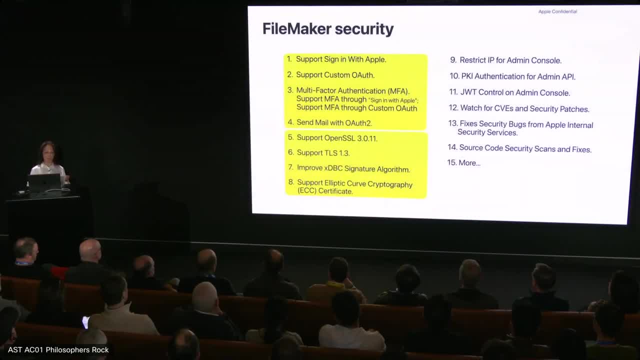 TLS 1.3 boosts security and better performance for a speedy connection And let me know if you need FIPS 140 compliant, We can talk after this session. for XTBC, We upgraded X509 signature algorithm to SHA256 from MD5.. 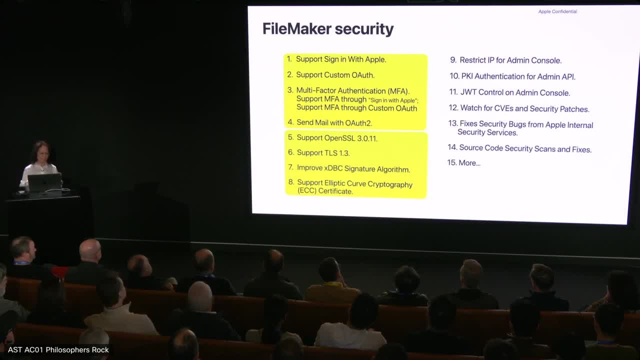 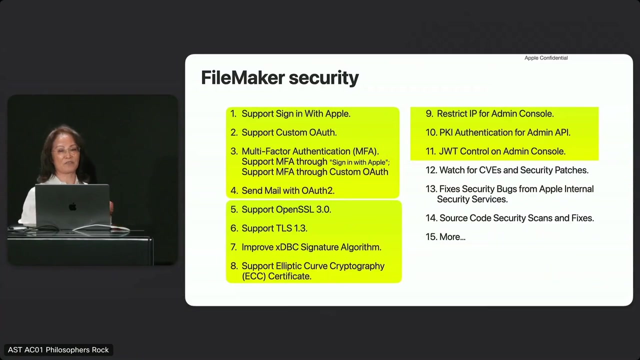 We support ECC certificate for a higher encryption strength, such as P384.. SEC is considered very secure against attacks. ECC is considered very secure against attacks. access to specific IP addresses. We added PKI authentication for Admin API. PKI stands for Public Key Infrastructure. 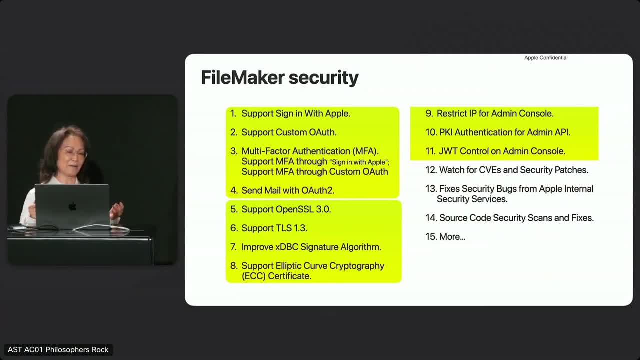 for Online Information Security. No need to share Admin password for running Admin API. Admin can control JSON Web Token JWT on Admin Console. It is secure, compact and fast. Finally, when we triage bugs, we treat security as high priority at all time. 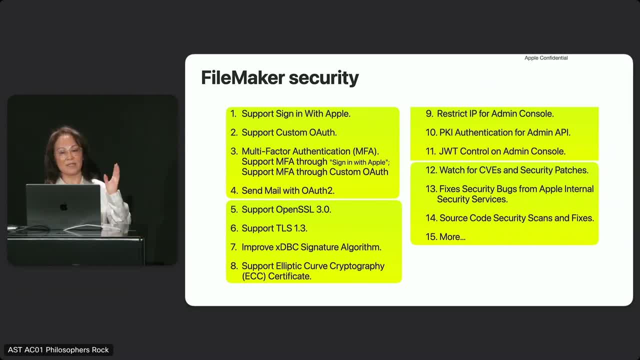 We always watch for common CVEs and security patches. Claris is an Apple company. We follow Apple high security standard. We do security code, We do source code security scan for our product and fix vulnerabilities whenever possible from multiple sources, including Apple internal security services. 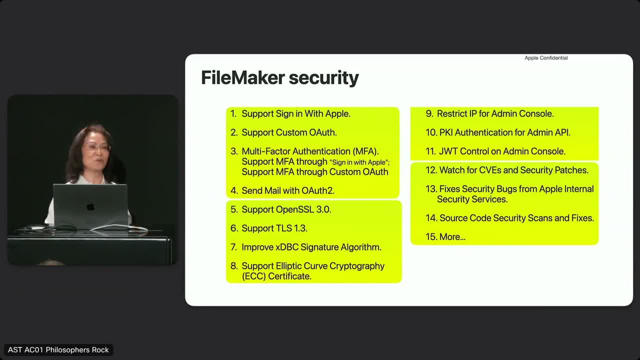 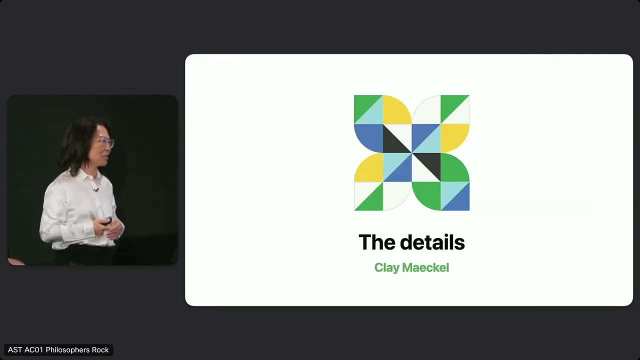 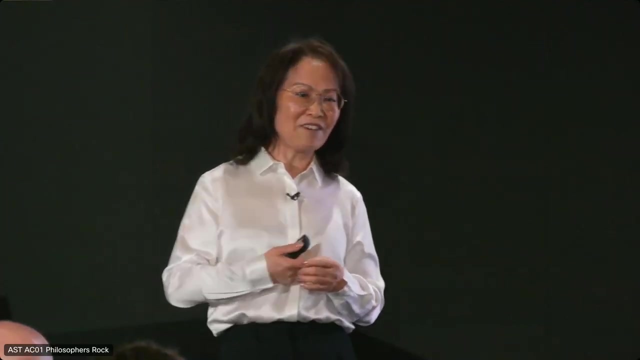 We made FileMaker more secure. It's important for you to upgrade as soon as you can. With all these, we are delivering the most powerful version of FileMaker ever. It's the best time to be a FileMaker developer And I want to invite Clay, the guru of FileMaker everything. 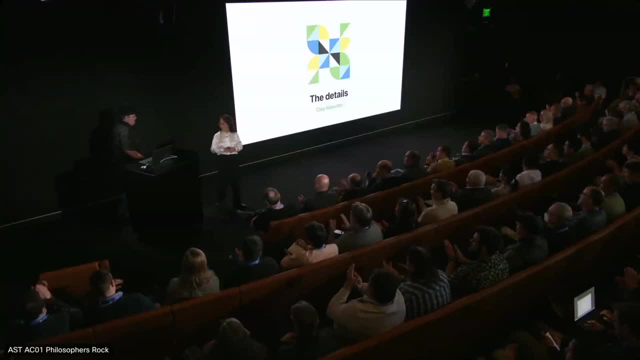 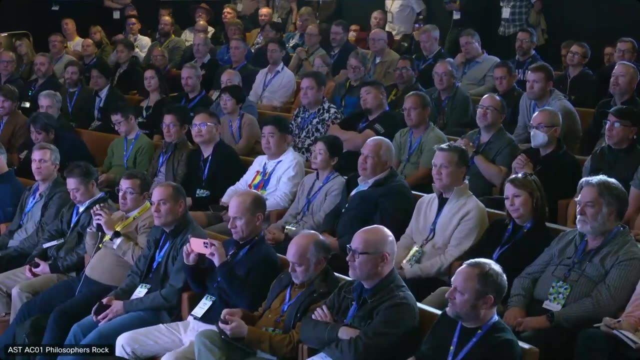 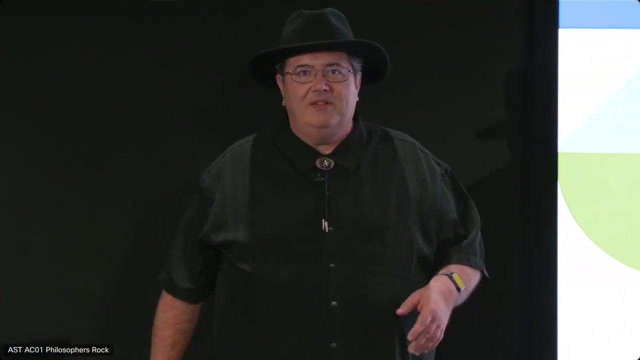 The one and only Clay. so there we go. So thanks, Lucy, but I'm gonna start talking about the FileMaker Clients Pro and Go first, then do some server stuff and other sections like this. Now, this is gonna be a mixture of 2023 features and 2024 features that are 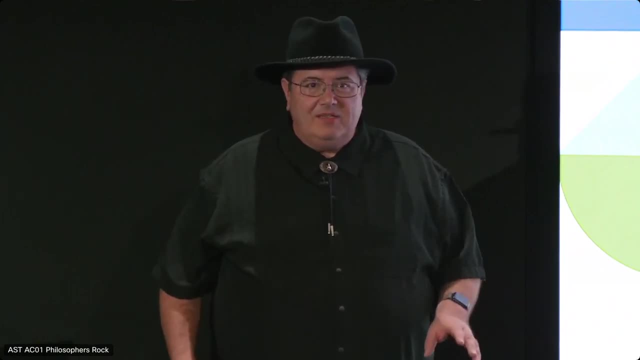 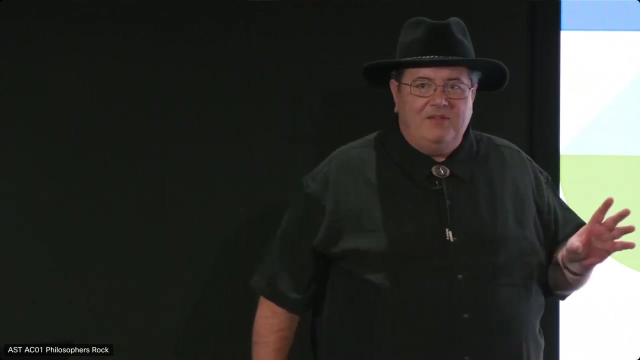 upcoming and what the differences are, and some of the under the hood stuff as I go across all of them Now, the stuff that you see that I'm gonna be talking about 2024 may not be in the first release or in this first ETS release, but most of it is all expected to be out by the end of this year. Much like we had three releases of 20, maybe we'll have three or four releases of 24.. Or we'll have three or four releases of 24.. 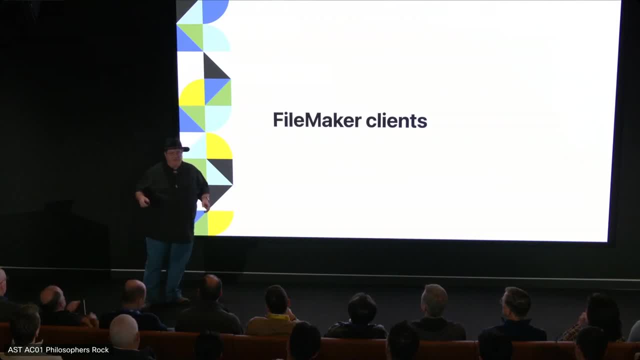 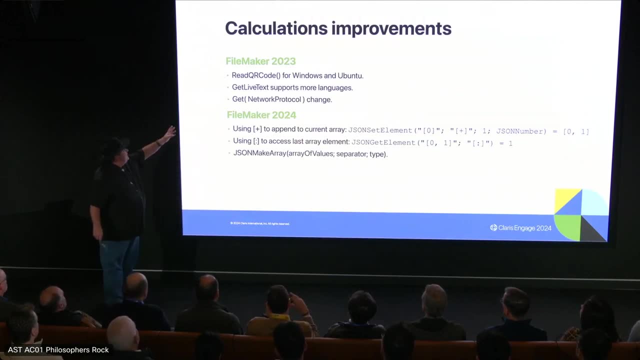 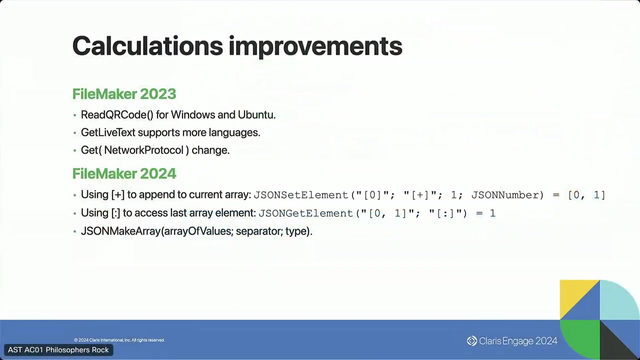 Which internally is gonna be called version 21, just to make things even more confusing. So calculation improvements In FileMaker 2023, there is read QR code. We've brought it to Windows and Ubuntu Now. this is a kind of an ongoing theme in general in these releases and 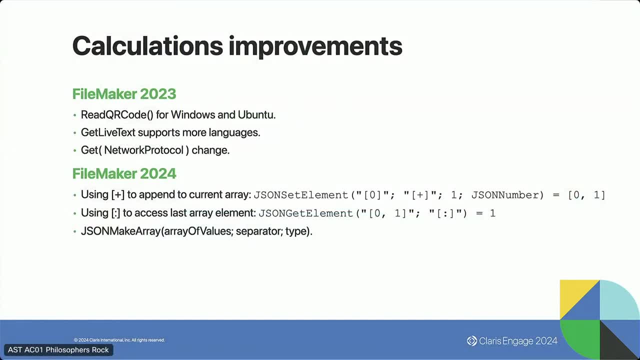 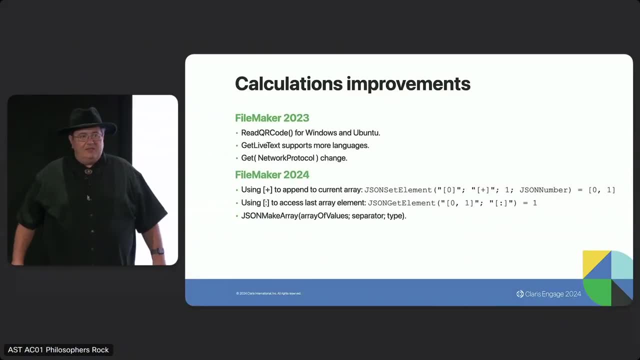 upcoming releases is that we're bringing technologies that were only specific on certain platforms and bringing them over to the other platforms, Or even stuff that was on iOS only and bringing it to other sections, And stuff that was on Netflix And stuff that was on Mac and wasn't on Ubuntu and stuff like that. 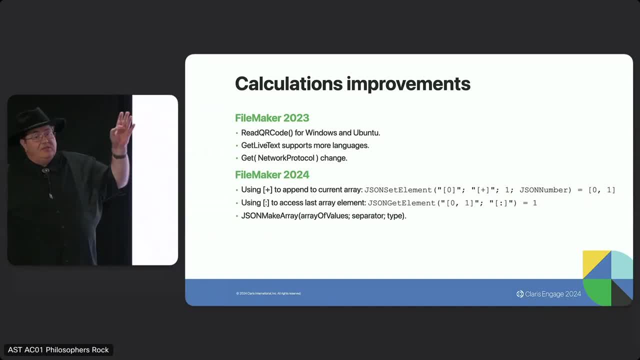 GetLiveText supports more languages, and this is another one where we're working in the future to actually improve GetLiveText- You probably won't see it in the first version of 2024, but to actually work on platforms other than Apple platforms. 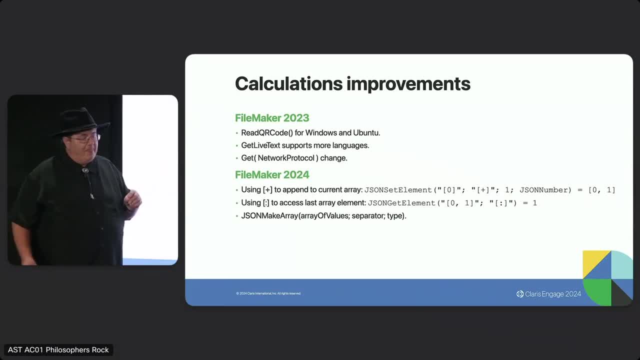 And also to support other multiple other data types and other than images, So like PDFs or maybe Word documents and stuff like that. Well, this is really being kind of driven by the AI work, Because we wanna be able to feed all your documents into and 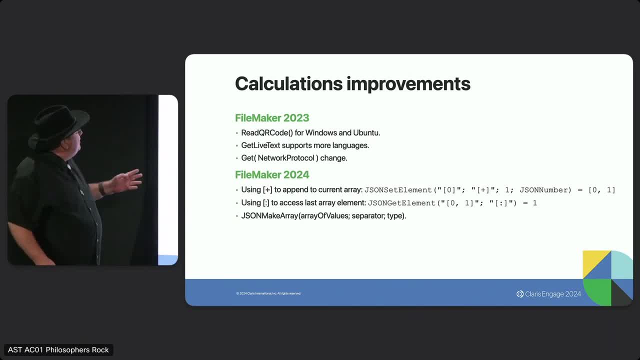 spread em out so more things can be hallucinated on. We have GetNetwork Protocol. okay, This is something I rather like, Cuz I wrote a whole bunch of different protocols and reports for like Apple Talks, IPX, Net Payess. 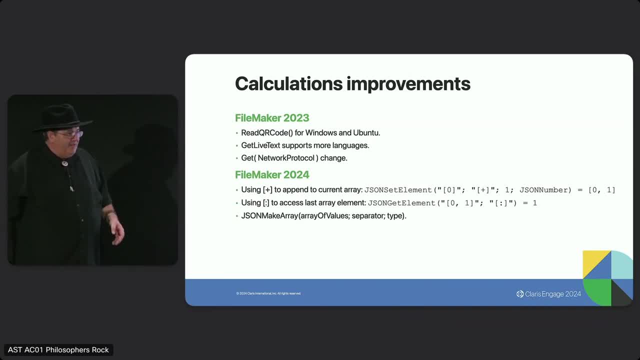 So this function used to return a whole bunch of different values and then eventually TCP I PC, one which didn't actually exist in the first version of FileMaker. So that took over and so it's been returning that for like the last 20, some odd years, or something like that. 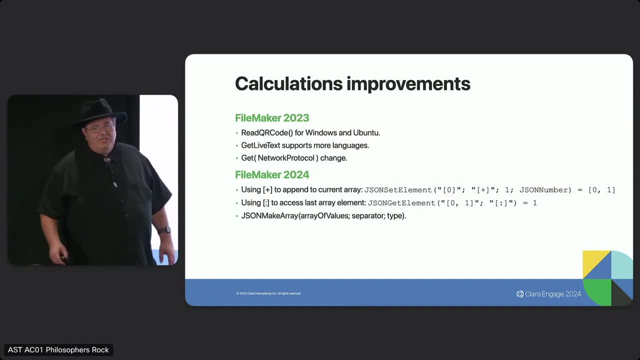 But now it actually gets to return something else. When you turn on HTTPS tunneling, it will now return HTTPS. So there actually is a use for this function now. FileMaker 2024, we're doing JSON improvements. This first one was brought up on. 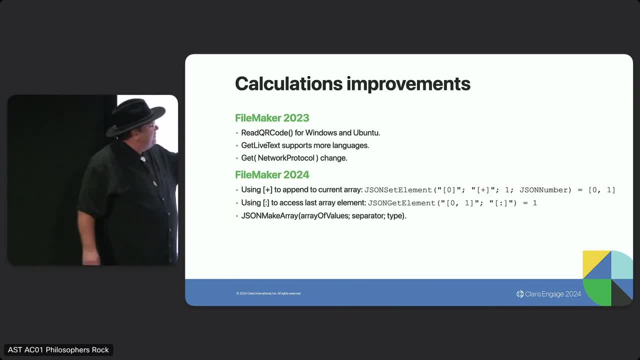 the community forums and had a lot of discussion how to work for it and stuff like that. But basically you can just, instead of going through looping and finding out how many elements in the array, you can say: I just want to tack something onto the end of the JSON array. 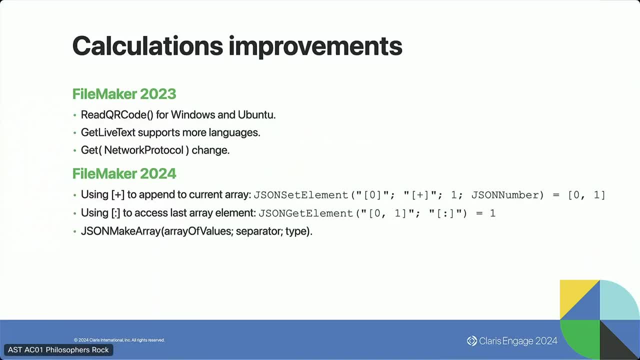 So you can use the plus operator. When I was in Antwerp we were discussing this and people were. they were actually already mocking it up and seeing how it would work and stuff like that. They say, well, when I append something to the end, 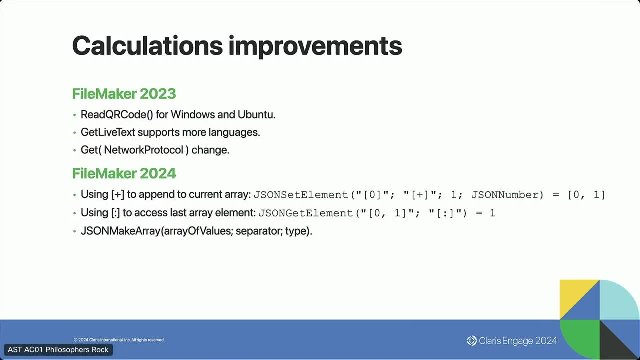 when does it want to reference something at the end? So we had like a three-hour discussion trying to determine what the character is going to be and I implemented it in about 40 minutes. So that's how things usually work. But so now the colon character is going to be last element. 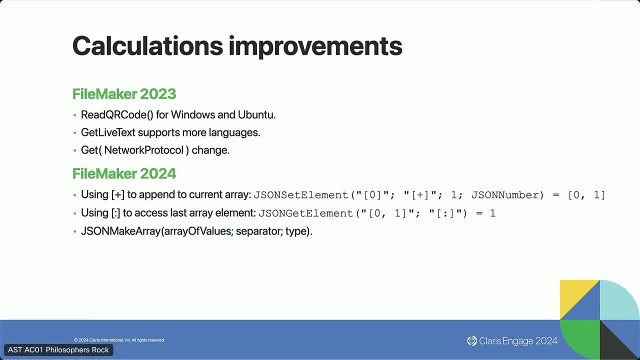 So it's nice. You can use the appender to put a JSON object at the end and then use the colon operator to set specific fields inside that object that you added. It makes things pretty nice. Another thing we're adding is a new function. 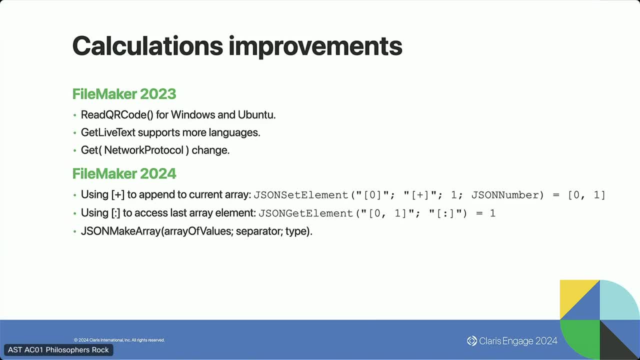 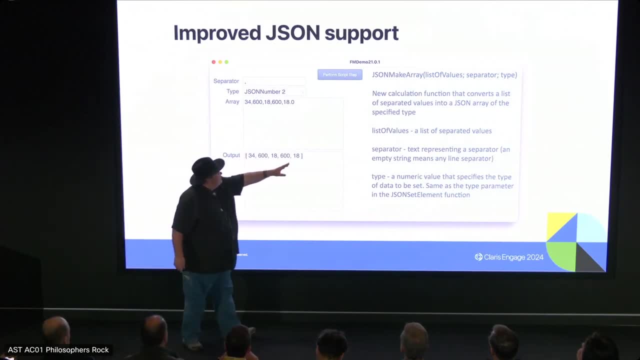 Everyone seems to be wanting to use arrays now, but a way to make an array a little bit easier. So there's the definition of the function up there. There's three parameters. The first one does you give the list, you give the chunk of text that has. 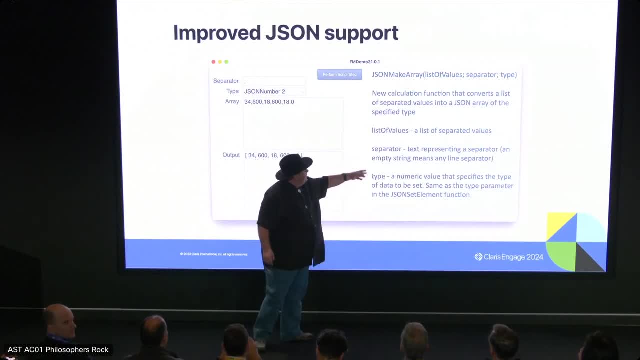 the elements you want to add to the array, The separator. you can determine whether you're using commas separated, tab separated or carriage return. We'll go to the next slide to see that And you determine the number, type or the type that you want all the elements in the array to be. 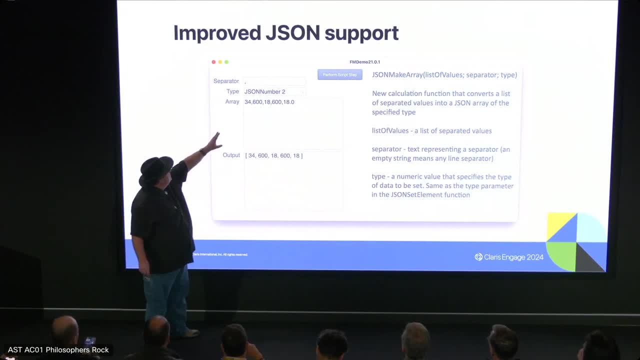 And in here I'm using comma. I want JSON numbers. There's the input and then you just get an array of numbers. In this version, I want strings. I want to have red, green, blue be part of the array strings. 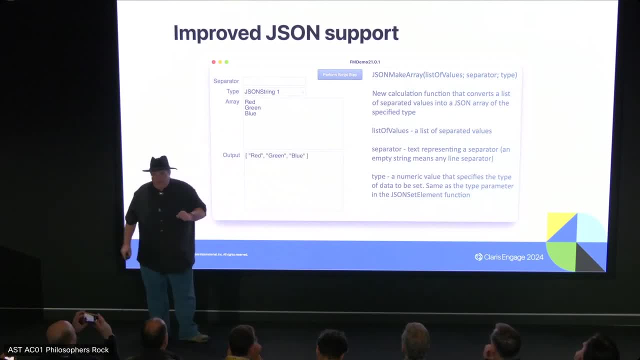 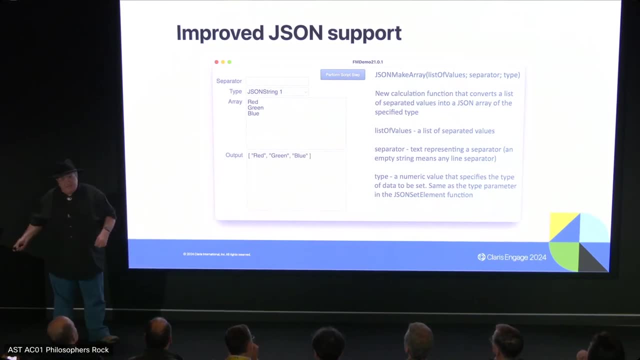 And notice that the separator field is empty. When the separator field is empty, it'll treat that the default is basically look for carriage returns line feeds, carriage return line feeds or the multitude of you know. 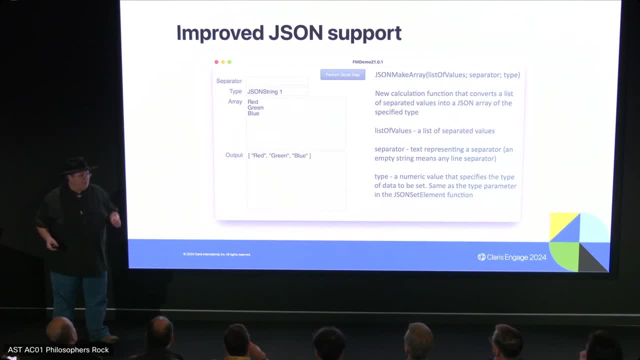 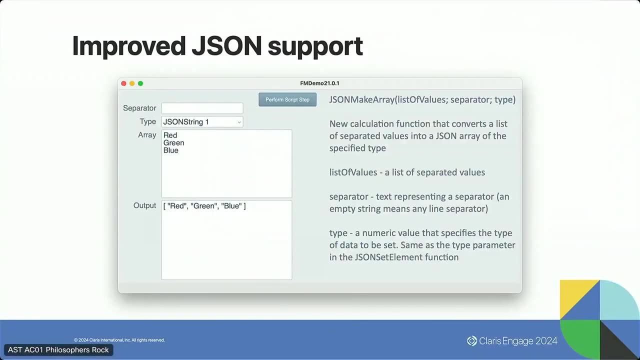 code, characters that represent paragraph in locations and stuff like that. So when it's blank it's actually scanning for a lot more different things. to find the with a line with the array terminator is: And in the last place- here I'm using the sharp character. 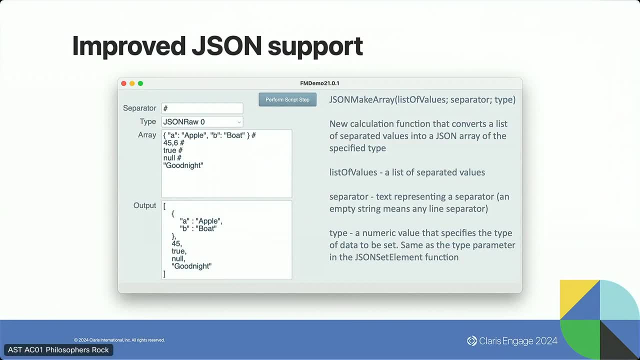 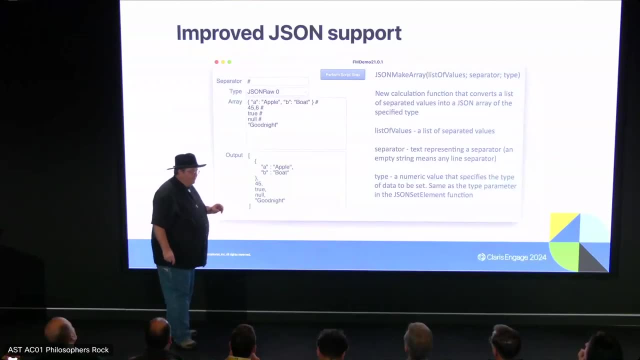 and using JSONRaw. I don't know how many people of you know actually what JSONRaw is doing, but what JSONRaw does is, once we grab the text, we give it to the JSON interpreter and then it tells us what type of what type it thinks it is. 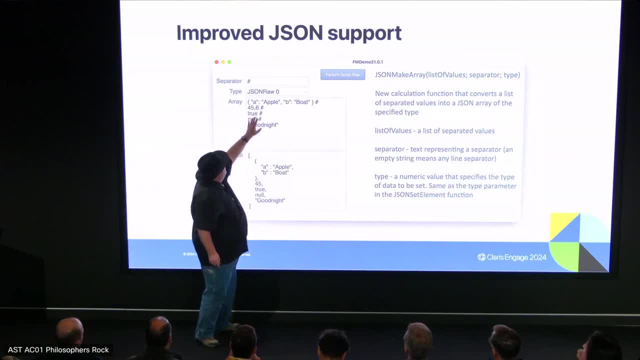 So if it sees a JSON object or numbers or Boolean or null, we'll just output that as those types. If it sees a string, or if it can't parse it, if it can't recognize it, it doesn't know if it's JSON or. 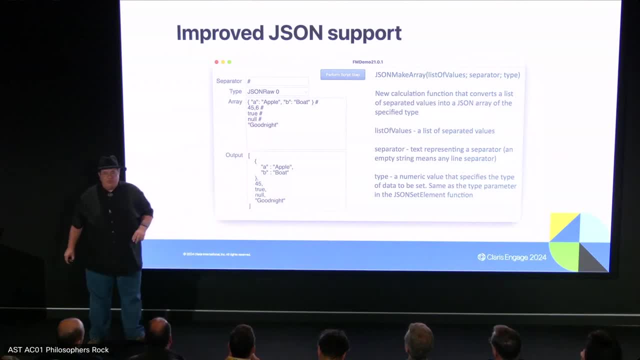 not JSON. it'll just put it in a string So it'll quote it and dump it down in there, So JSON is actually. there's some interesting uses that you use with JSON raw if you're doing mixed operations and you don't know the data type. 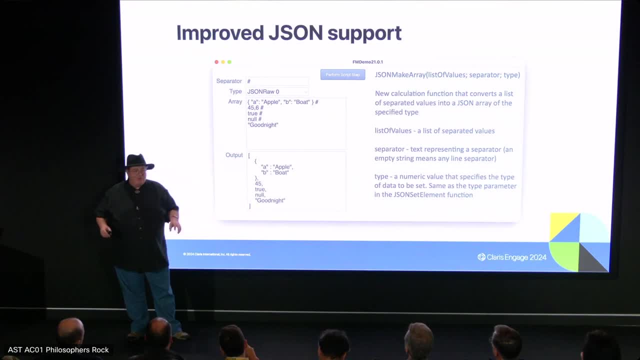 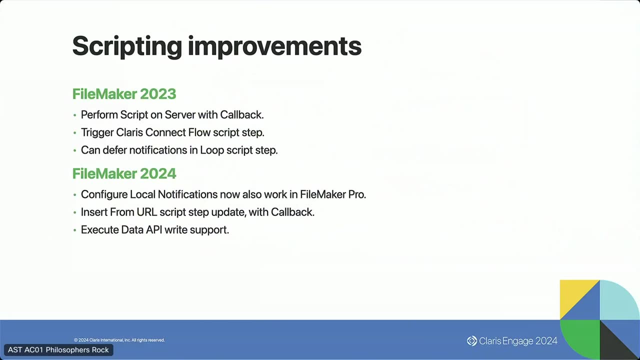 But it's not the guarantee that it won't fix your JSON or stuff like that, but it interprets the data coming in. Now we go on to scripting improvements. We have the perform script on server with callback, which has been mentioned, Triggering Claris Flows and Claris Connect Flows script step. 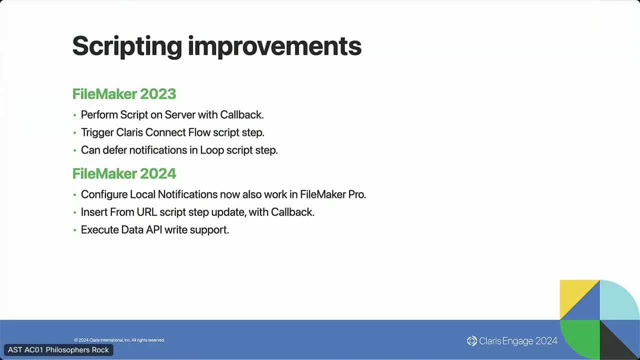 This then the first step, the first version. you had to copy and paste the URL And then, in another version you had to. you got a pop-up of the flows that were available to you if you logged in with your Claris ID inside FileMaker. 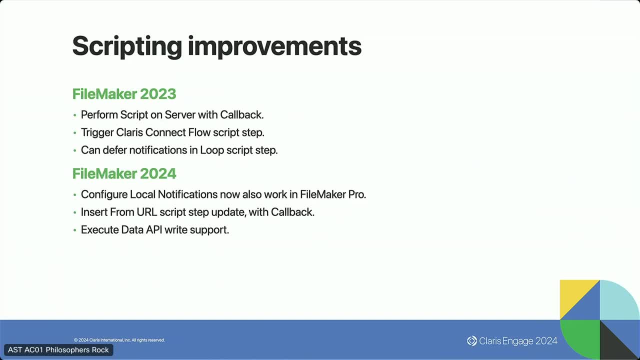 That's another change with. the thing is, yeah, FileMaker 20 is. now you can always log into Claris ID. Before it was determined on the type of license you had- whether you had a license that was dependent on the that you could connect to cloud. 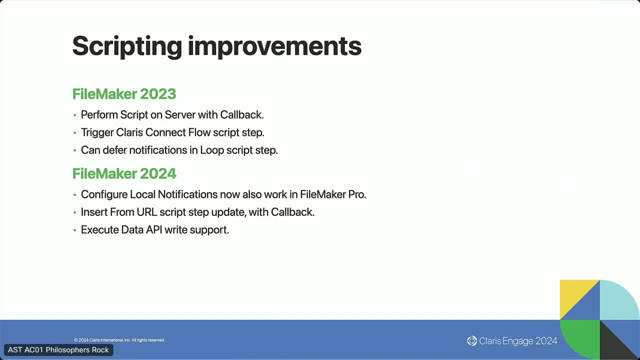 But now it's always available there because we're using that Claris ID to log to access the file. So it's just connect studio and cloud. There's the can defer notification and loop script step. I notice that there's been a couple sessions already talking about this. 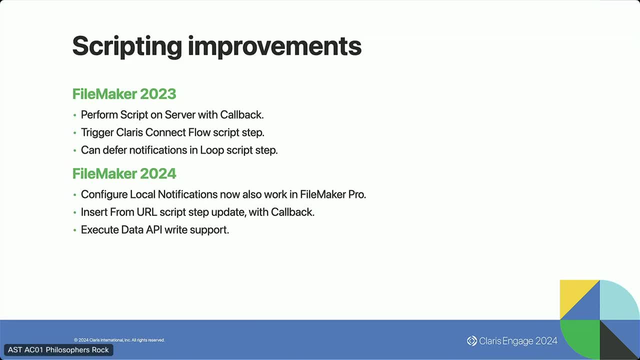 but- and we have a blog talking about when you would want to use it and the different behaviors when you, with the three different options, The short thing- I mean the CliffsNotes version of it- is if you're doing anything relational inside the loop or 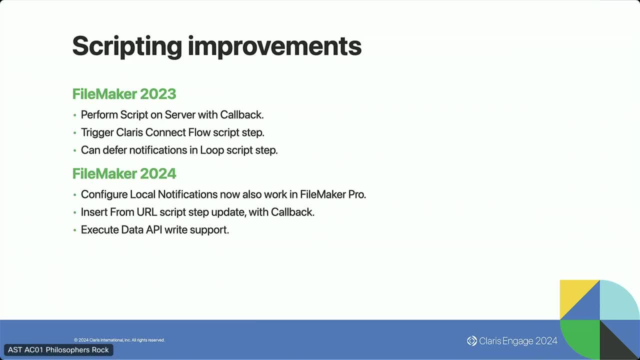 you want the UI to refresh while you're inside the loop, leave it the way it is, You don't. you do not want to defer it. If you're doing neither of those things, then you can just go ahead and defer notifications. 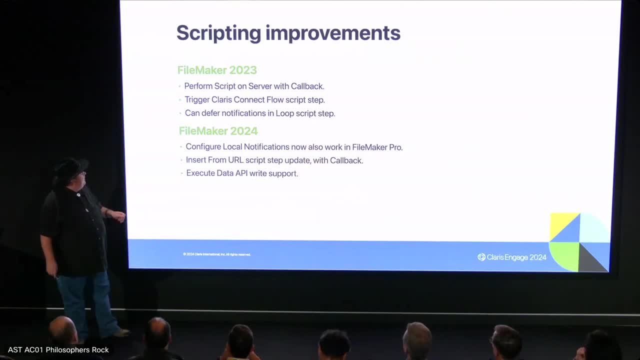 and the loop will go quicker. Well coming up in the future. this is the configure local. local notifications will now work in FileMaker Pro. Lucy mentioned that This is still other operations that we're bringing to multiple platforms. This was a iOS only feature and now you can bring it up there. 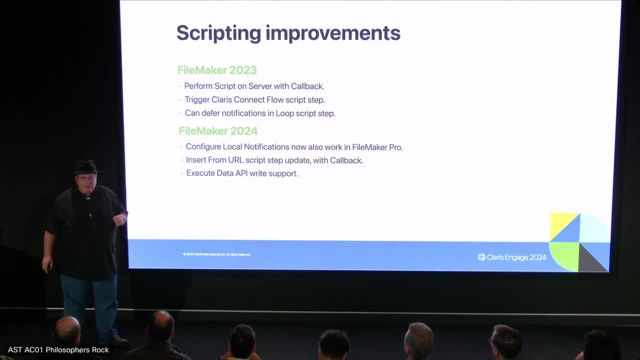 And we do have a prototype of it. We're working in Web Direct. I'm not quite sure whether they'll make it out in the first release or not, But we're working to try to bring that also to that platform. Some of them are coming up. 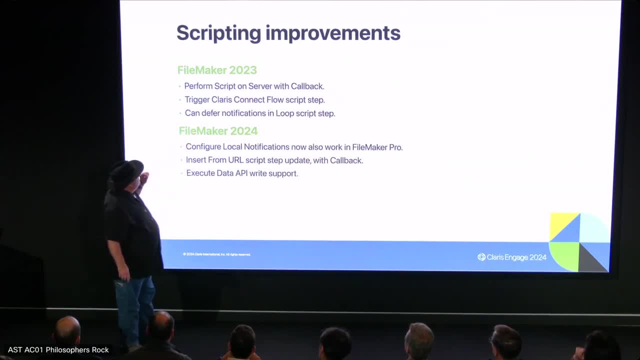 Notice that we've been starting to do more things with callback. This is kind of our. I guess people have been wanting to do like I want to run multiple scripts at the same time. We want to have more asynchronous operations and stuff like that. 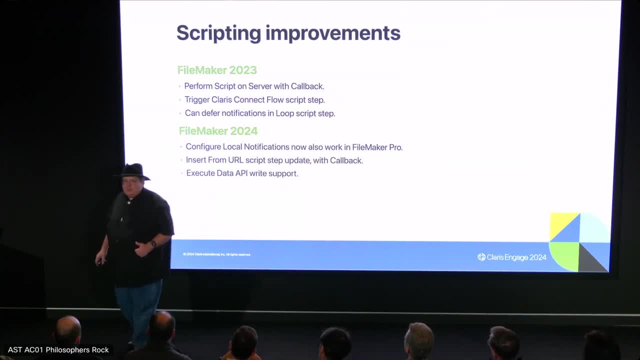 FileMaker being a very context-sensitive, I think it depends on which file window record you have selected and where the insert cursor is located inside the field for all this stuff, Trying to do multi-threaded operations when there's the context of just how. 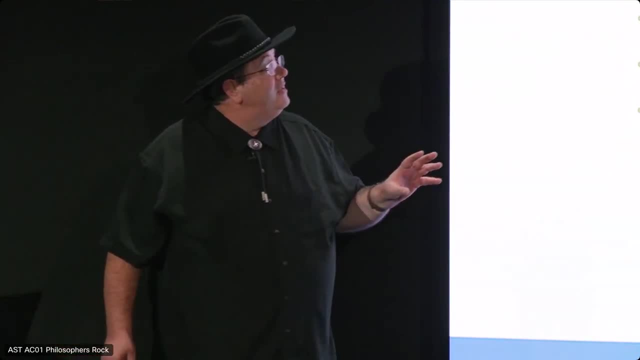 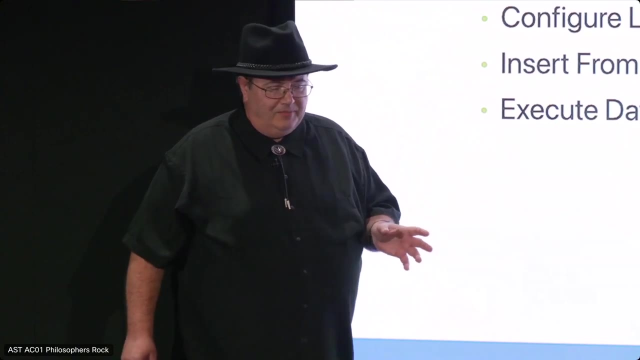 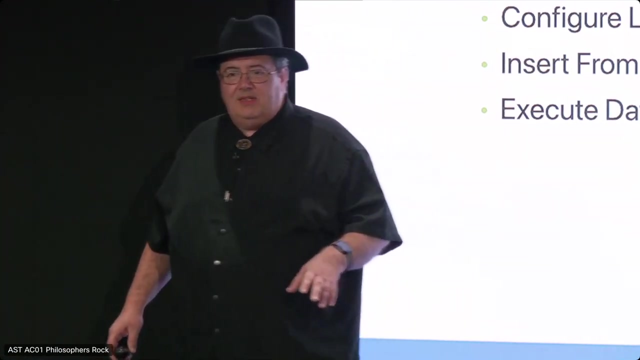 the machine is setting. there is very tough to do, So we're gonna stick with this callback model where it actually the first version of it was: on the install on timer script step. That actually is basically an early version of the callback, because after the timer triggers, it would then schedule the script to be executed at the next. 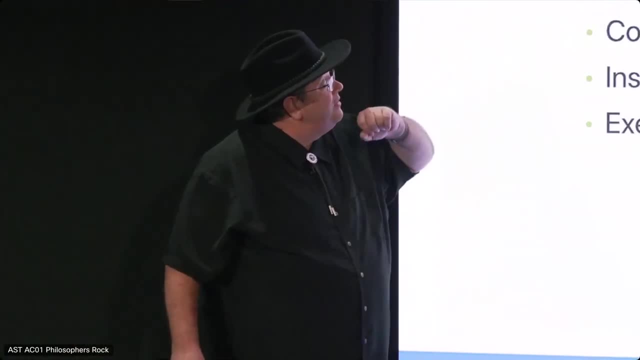 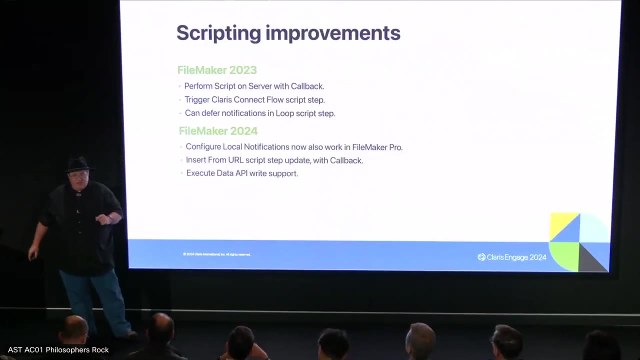 possible moment- And that's the same mechanism that performs script on server with callback- is gonna be using and what we're gonna be bringing to insert from URL. Now we're gonna probably be leaving insert URL the way it is, that current script step. 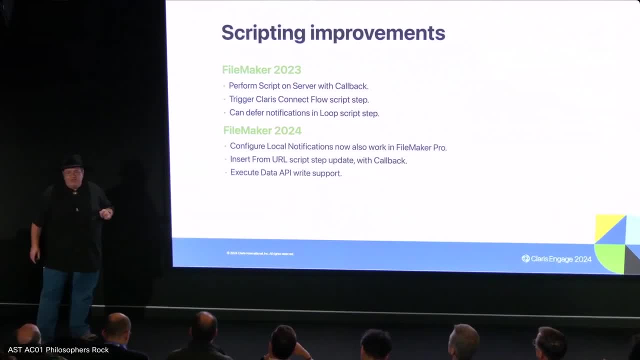 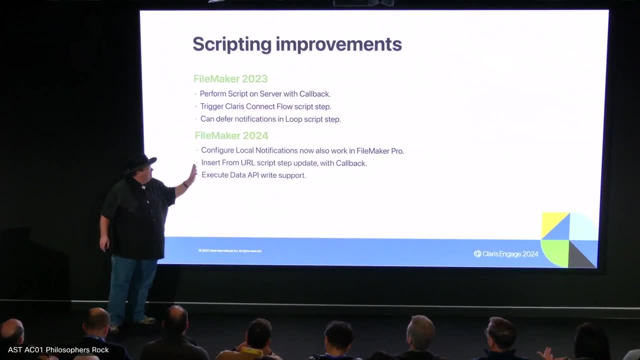 And it's gonna be a newer version that's gonna be more microservice oriented and won't be dependent on where the cursor position is. We're gonna be removing, basically, the cuz insert. all the insert scripts behave the same way. They depend on what field is selected, actually whether all the text is selected. 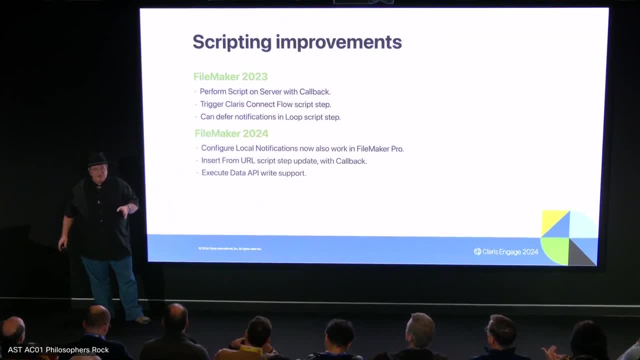 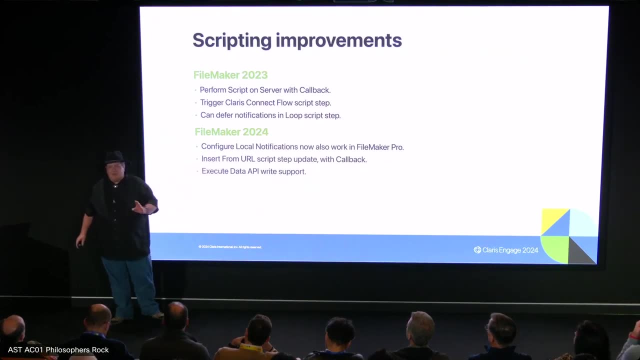 or whether the cursor is blinking in a particular location. It's really more. anything starting with UI is really more UI oriented. But insert from URL is being used for a lot of other purposes in doing. I don't know how many people are actually using it for UI purposes. 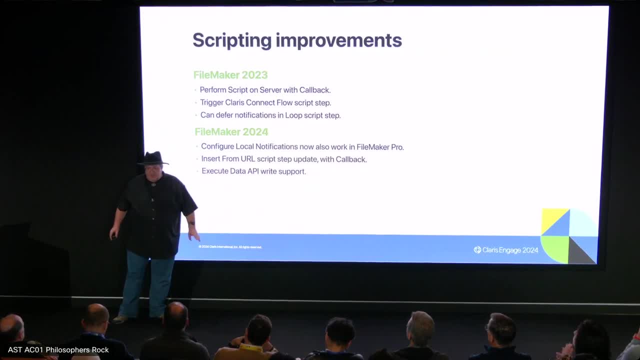 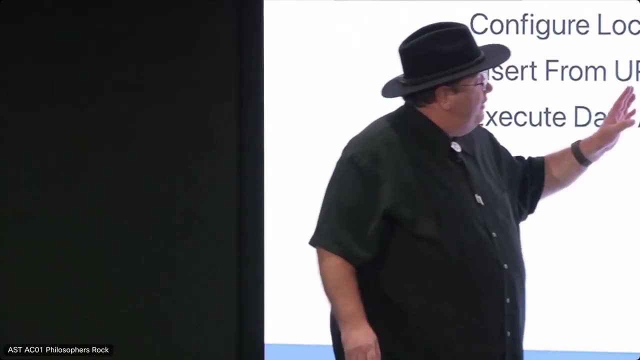 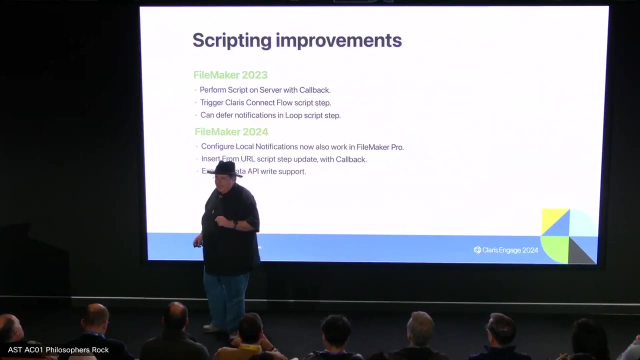 But we'll have a new version that's with the GUI and the options that are more relevant for doing microservice calls, And you could start a download and then, when the download completes, a script will be called telling you the download completed, And we'll probably- I don't know whether it's gonna be the parameter or- 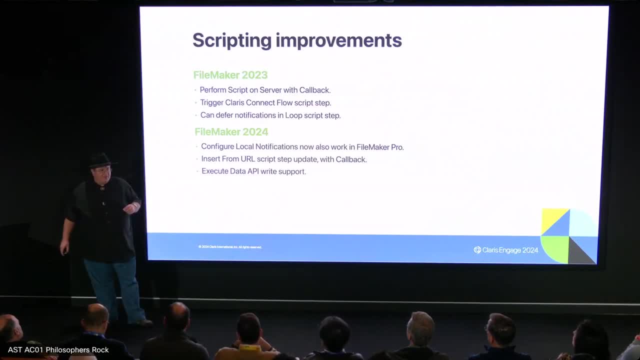 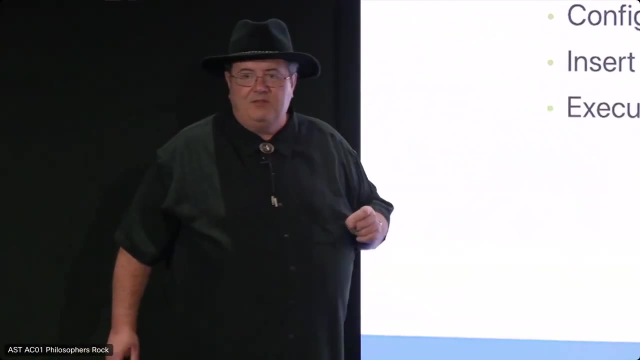 there'll be some mechanism to get the results of what you asked for. They'll probably be the parameter of the script that's called. The other change is the execute data API now has write support. Previously you could get the metadata or do read operations on data using that script step. 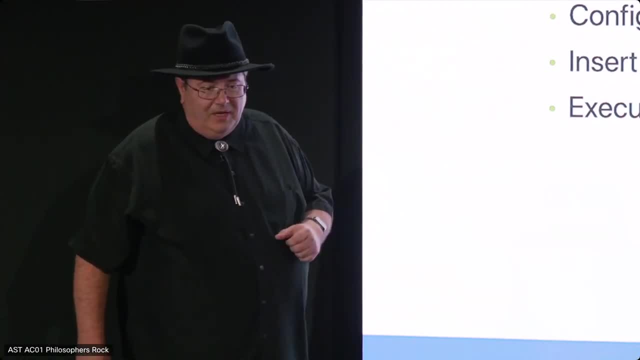 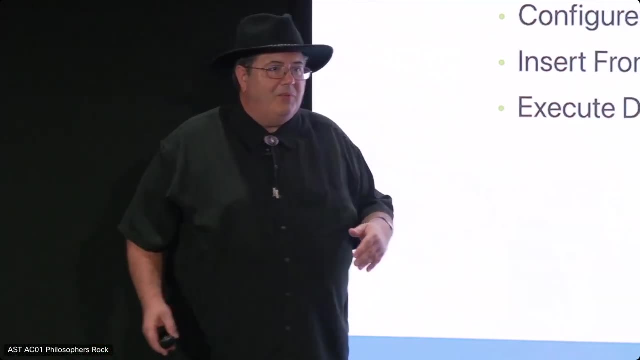 One thing that we noticed if we went back to the on window transaction trigger. You have a when you want to. if you're doing auditing and you want to write the same file that you're in, you have to worry about recursion because you don't want the on window transaction to trigger for. 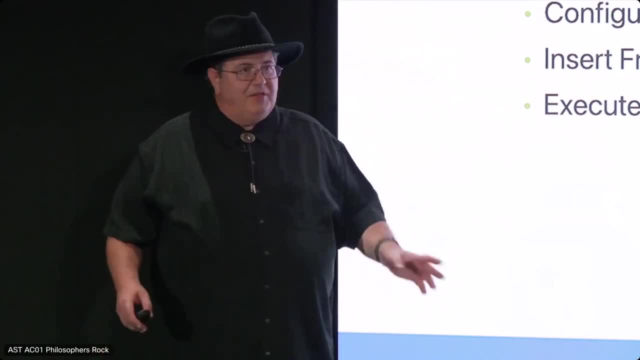 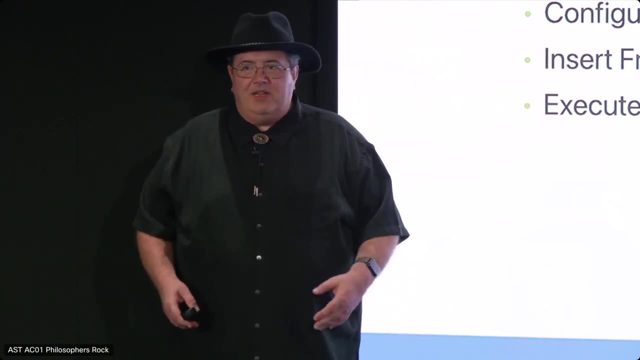 your audit records. But- and there's different tricks- You can open another window, but then returning the state back to where you were can be complex sometimes. Or the best thing is like, I think, the demo we have writes it out to a file. 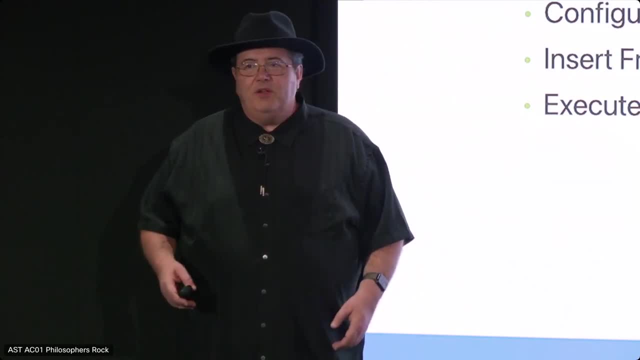 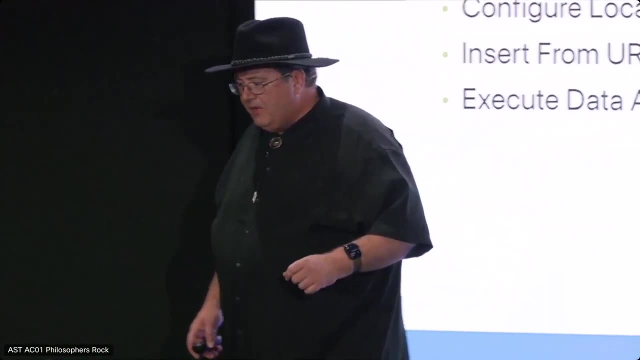 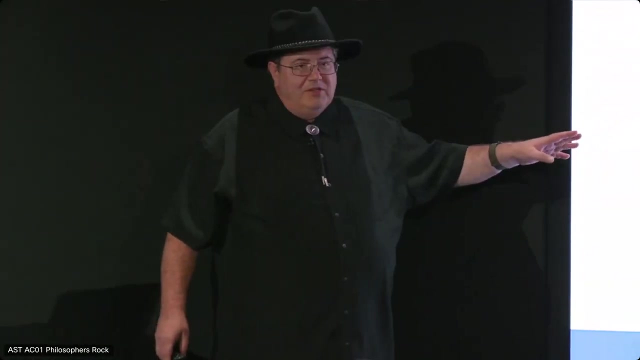 Or To like a text file in JSON format, Or you can just write it to another file that doesn't have this trigger on. But now with execute data API, write support. the FileMaker data API doesn't trigger the on window transaction, So you could just do write operations directly to wherever you want. 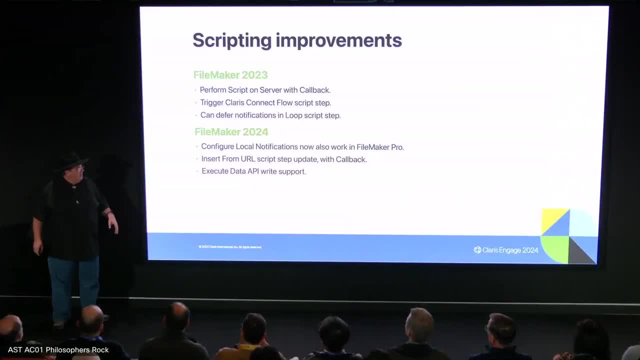 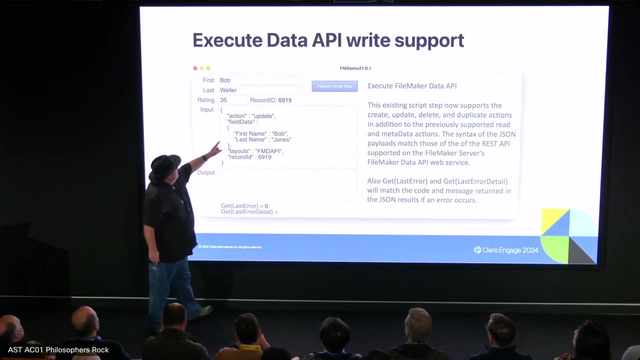 For your auditing information or make your sync statements, And there's probably gonna be a whole bunch of other purposes why you want to do write operations internally at some point. that's not dependent on the client Context of anything else, And so this is what it looks like, that the key change. 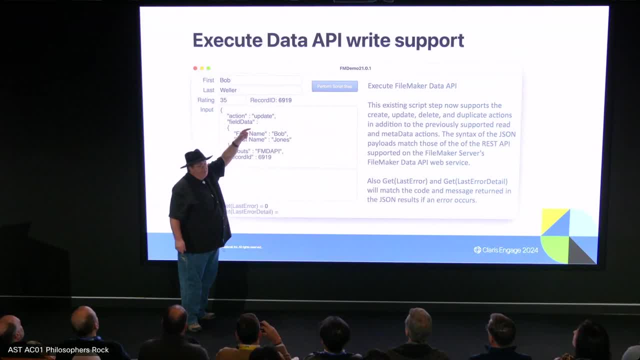 Key change is that the action tag here now has more things other than just read and metadata. So in this record we have Bob Weller with Iranian 35. His record ID is 6919.. You notice, this is your standard FileMaker data API request. 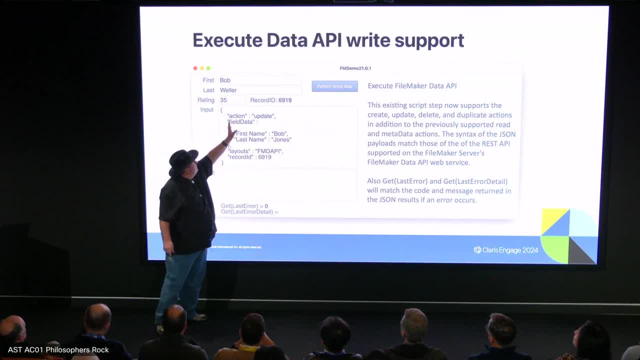 It's a little bit different than what you do over the network, because over the network you're doing, you're determining the action by whether you're doing puts or deletes or patches. In this version that's all determined basically by the action tag. But here we want to update this thing to Bob Jones with this record ID. 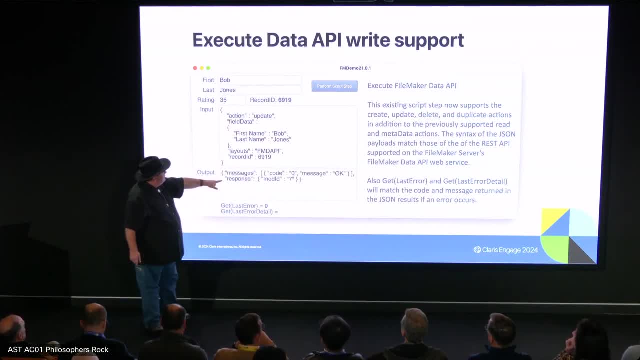 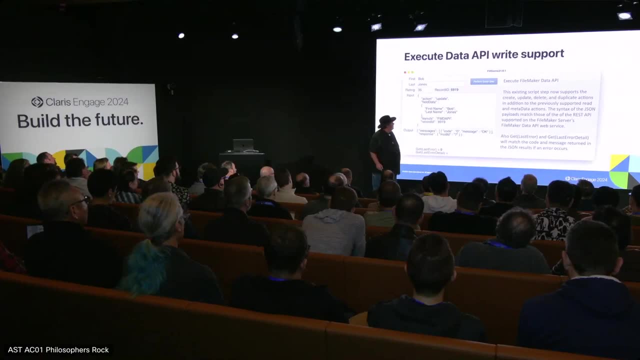 So here we execute it, it changes the name and we get the standard response back saying that there was no error in what the modification ID of that modification count, basically of that record. Now here we're gonna do Robert Scarver with a rating of 3, and we want to change his rating. 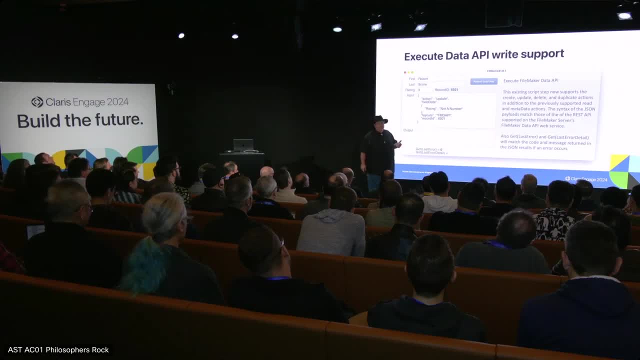 Now, rating is a number, Rating is a number field marked to be number only. And here I'm, you know, passing in a payload of saying that, oh, I'm trying to shove some text into this number field, So this should be an error. 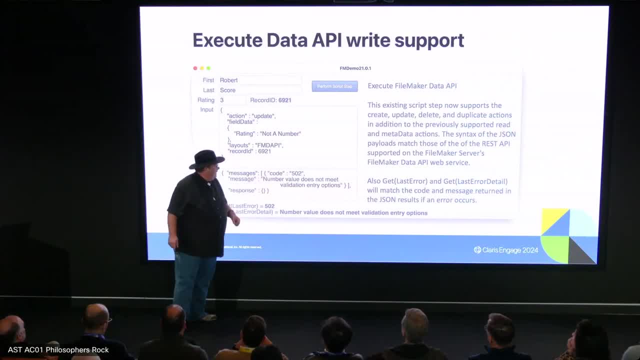 And, of course, when you execute it, you do get the error here And the string for it. A new enhancement for execute FileMaker data API 2 now is that we're gonna parse the JSON response coming back from that and set: get last error. 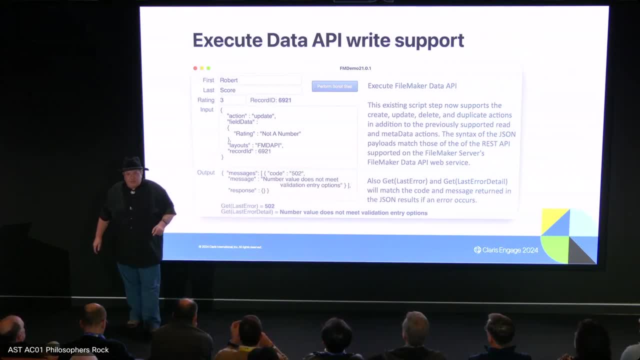 and get last error details with those values there. So when you make these calls you'll no longer have to parse the JSON result. For doing simple operations, all you do is expecting an error code or the error result coming back. You'll still have to parse it if you're asking for record data and stuff like that. 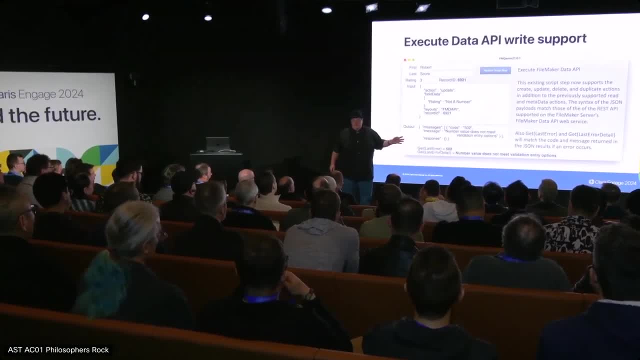 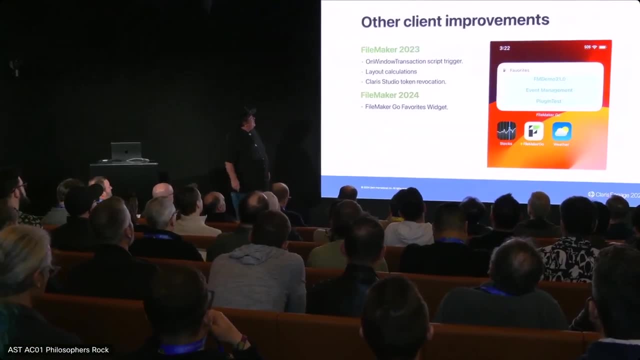 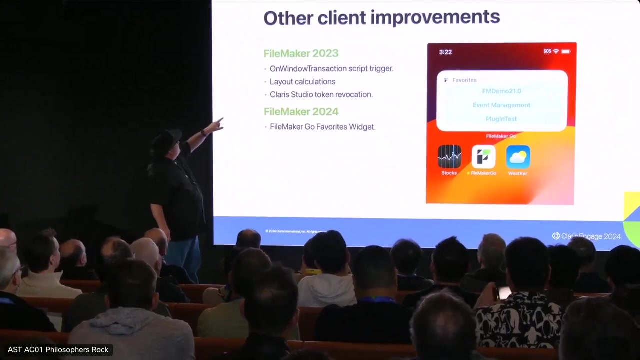 But a lot of these new calls. when you delete a lot of these newer ones, you're just looking for the error code and, whether it succeeded or failed, Some other client improvements- Don't look at the picture on the right. yet The on-window transaction script trigger that came in. 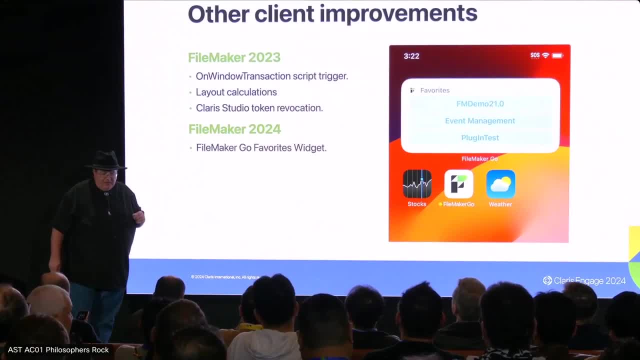 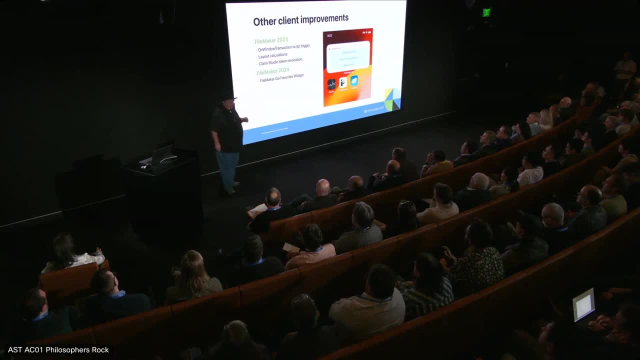 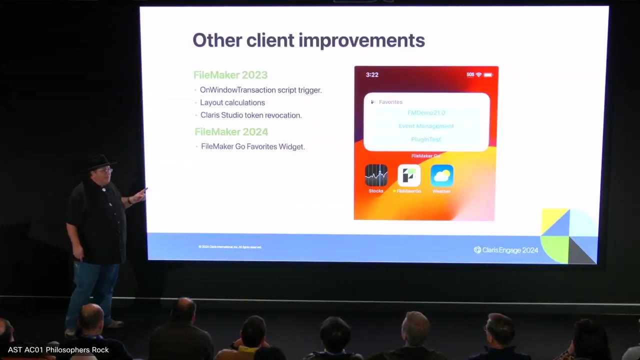 I've discussed that already. There's layout calculations, The first iteration of this. yeah, this actually caught our marketing department by surprise. They didn't realize everyone was going to be so excited about it. But you have to remember the first implementation of this. right now you have to treat it as the evaluate calculation function. 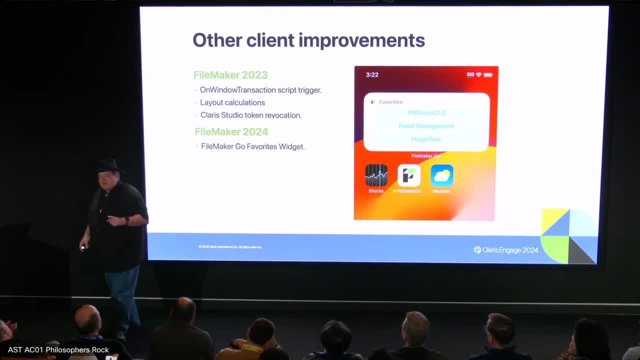 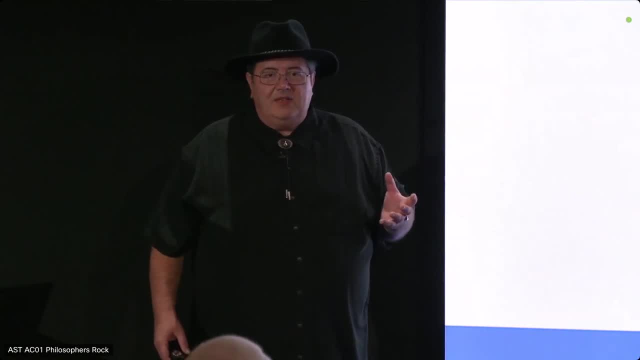 So all the limitations of the evaluate calculation functions apply to this text that you're doing there. So if you wanted to be able to work over multiple locales, the calculation actually has to be in English, Because if you try to run it on server, it doesn't know about. you know server, you can't set it to like Korean and stuff like that. 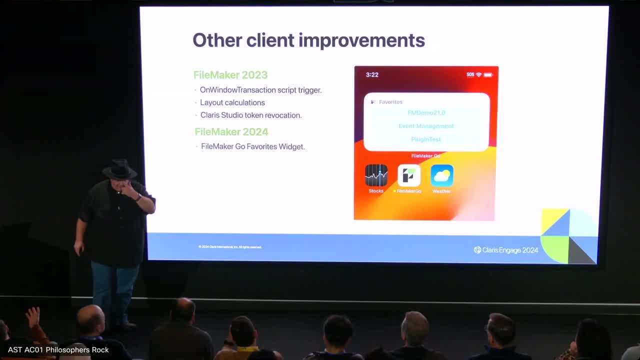 So it probably failed over there. The other thing that the evaluate calculation does: since you're only passing in the text of the calculation, It makes it fragile if you're going through changing field names, table names and stuff like that. So, but what you have to think is when you think of layout calculations, you really have to think, oh, this is really actually an evaluate calc. that's on my layout. 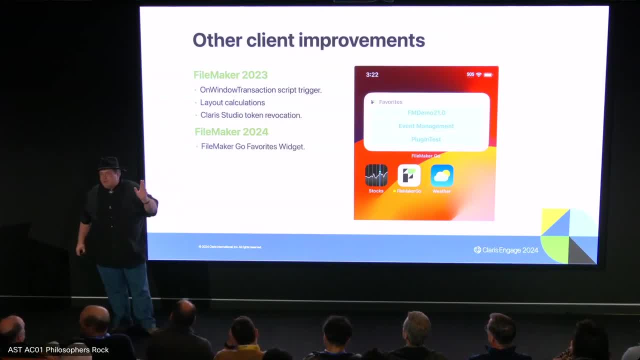 We do have plans to start back, doing a back store of this with the actual calculation definition, with the actual parse, the reverse Polish notation binary version of the calculation and put that in there. That will also allow us. I know Vince is complaining. 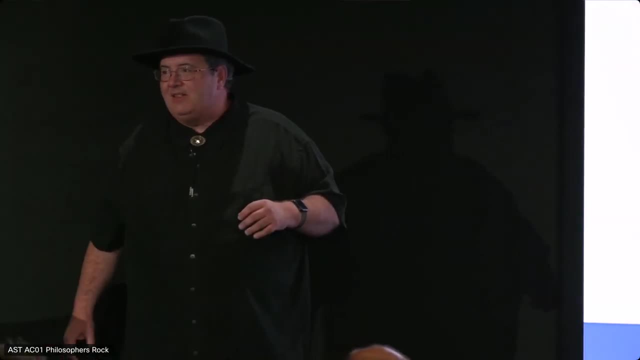 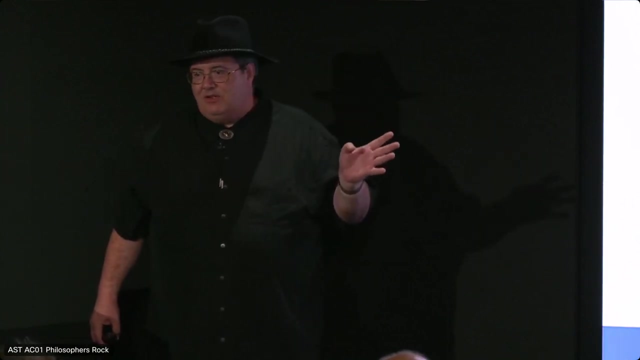 That he can't get the chunks of the calc from the XML definitions of these things. and once we back at store with that format- because it'll be backward compatible If only the text is there- we'll just use the text and continue using it like the evaluation. 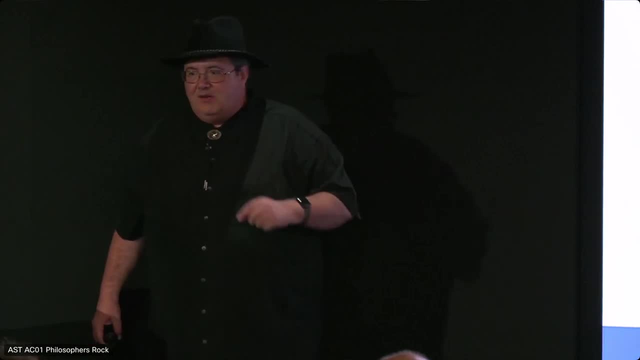 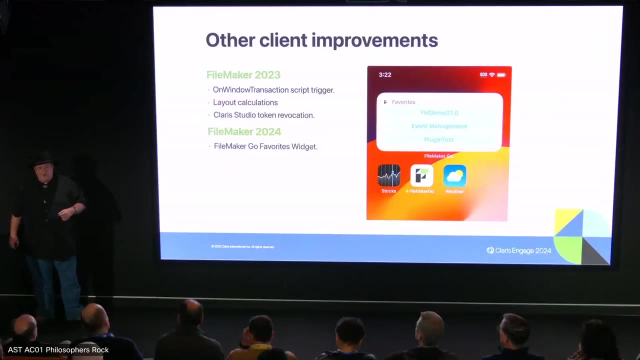 But I don't know if we're gonna try to do automatic update or you'll have to go in there like touch the layout text to force to do to generate the calc backing store for it. That will then then be used for doing evaluations. 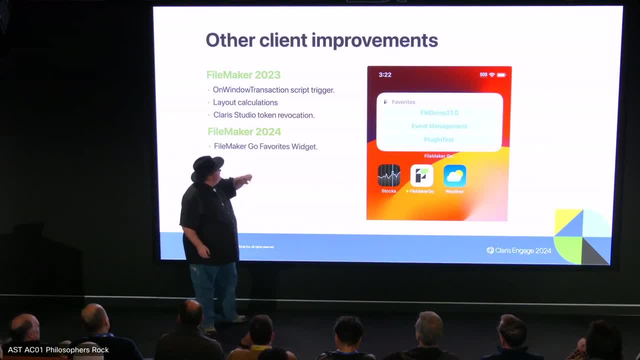 Um and well, I guess we'll talk about the go favorite rigid names, And then we'll talk about the go favorite rigid names, And then we'll talk about the go favorite rigid names. So on go. we've written a widget on there that will show you what the current favorite items. 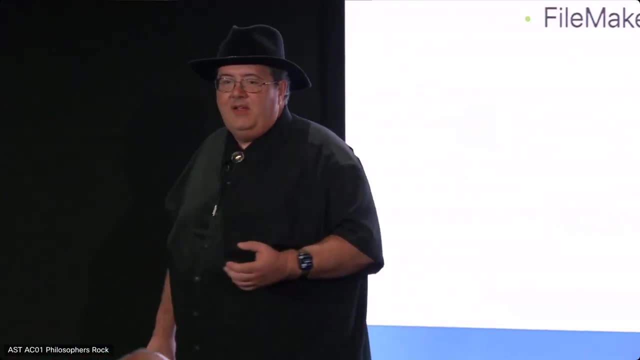 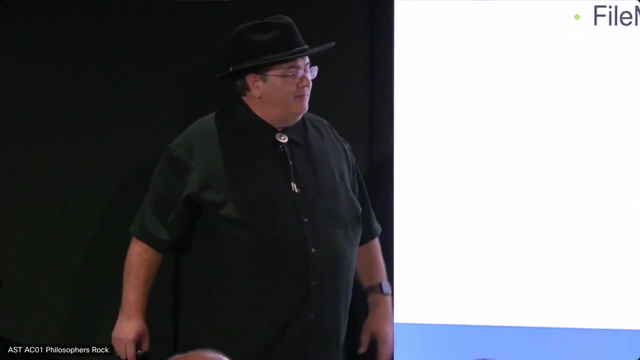 So if you go and you select a couple files and you make them your favorite file, you can now have a widget laying on your- I'm not sure what it's called. it's not the finder, it's a desktop or whatever they call spring bar, spring board, okay. 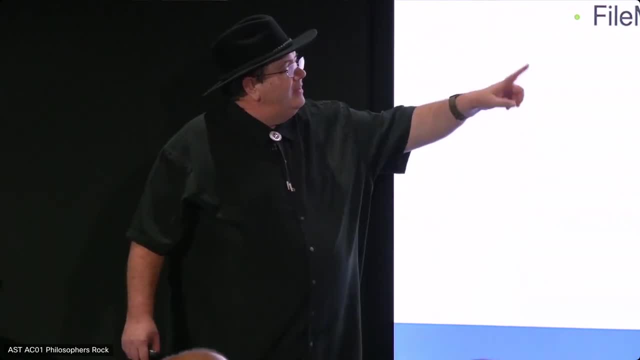 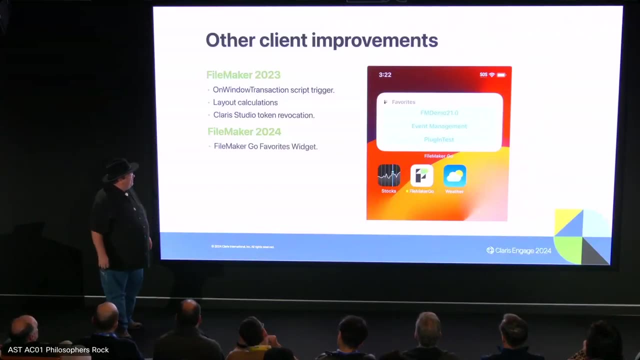 So you can put this widget on your spring board and you click on any of those things and it'll open, it'll launch, go and then take you to that file immediately. So it's a nice little Uh quick, you, you usability thing. We we may bring it to the Mac OS two, but apple keeps changing these widget APIs. It's really a pain right now to keep up with it. right now I can't even use Xcode 15 to compile this widget, because it just doesn't work at that point. 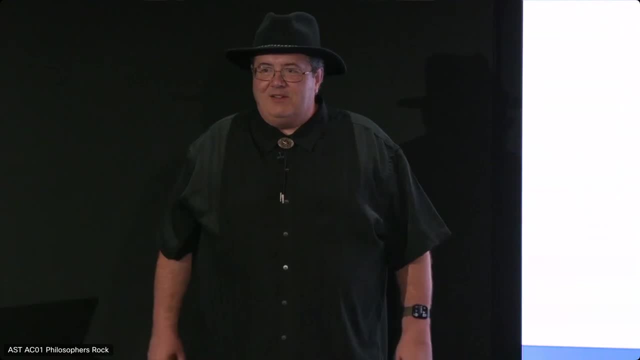 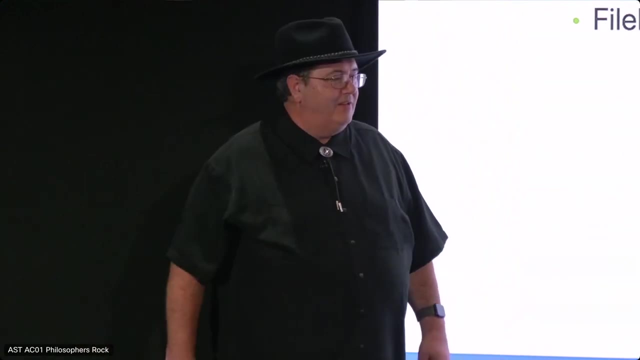 So I have to figure out. you know, all I did was just change compilers, and now it won't run, So, but we'll work that out. So that's a clue. We're still using Xcode 14 for the current version of file maker or this ETS build. So, but we'll work that out. So, but that's a clue, We're still using Xcode 14 for the current version of file maker or this ETS build, So, but we'll work that out. So, but we'll work that out. 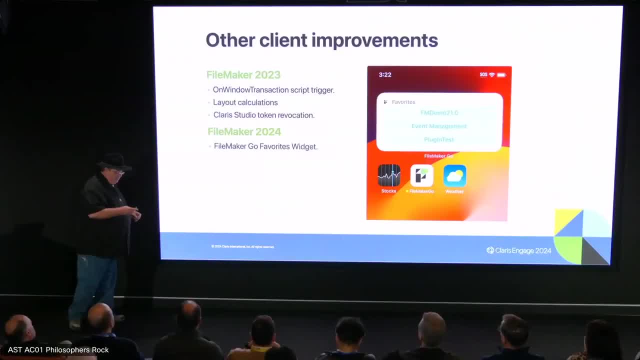 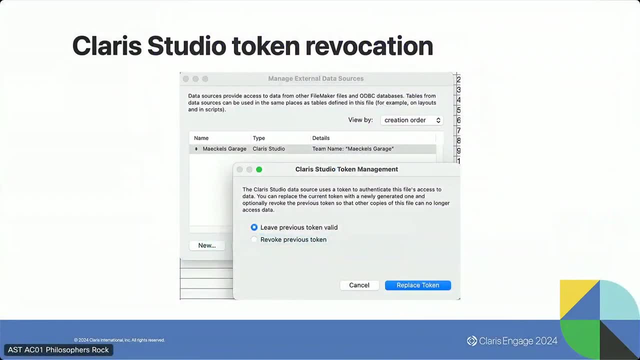 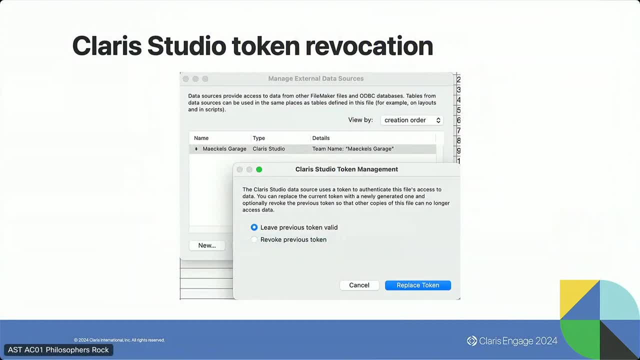 We to talk to. so we have to get into the details of how we talk to the Claris Studio product. So we we make a connection And you have to have a Claris ID where you're a team manager on it. 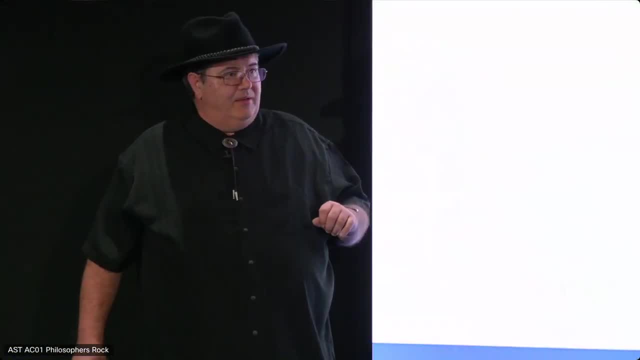 And once you have a team manager and when you go into the join graph and you add a new table reference- like how you do ESS and stuff like that- what you're actually doing is that it's using your team management credentials to get a token to access all those tables in that organization. 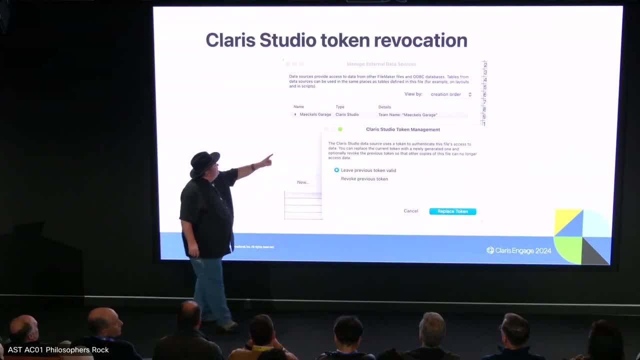 And that or that token is then stored And you can see this. if you go to manage external data sources after you've made a connection to that organization, If you go to manage external data sources after you've made a connection to studio, you'll see a type Clara studio type of external data source now in Clara's pro, if you double click on this thing. you did nothing at all once the token was created. you couldn't delete it, you couldn't revoke it. people would have access forever if they had that copy of that file. so that was a bit of a whole. 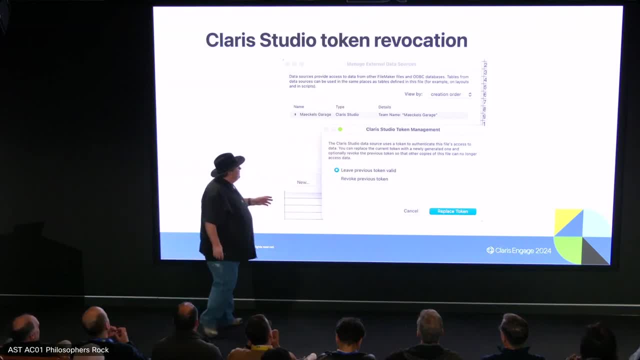 So, starting with the filmmaker 2023, now if you double click on it, you can at least revoke the previous token and get a new token to replace, to use it, or leave the old token alone, because you've given clones of this file to other people, that you want them to continue using that token, and then you want new people using your file using the newer token, and stuff like that. now, this is still not really optimal, but the studios 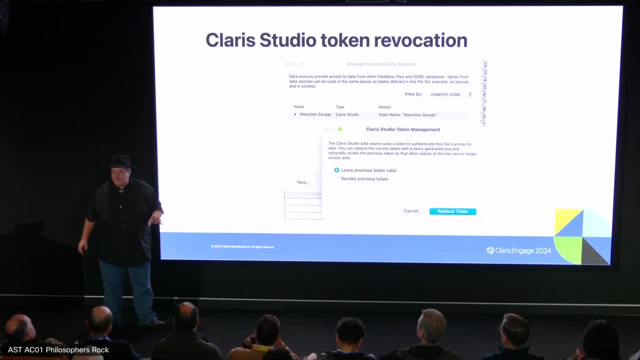 User Management and user permissions is still in flux right now and they're gonna have to be doing token management, to Which there will be some. you I should probably see which tokens and eventually when you, when you connect to Clara studio paving, you'll probably be asked: you know which token that you created you want to use for this connection, so you can do a little bit better management when you're creating solutions connected to studio. 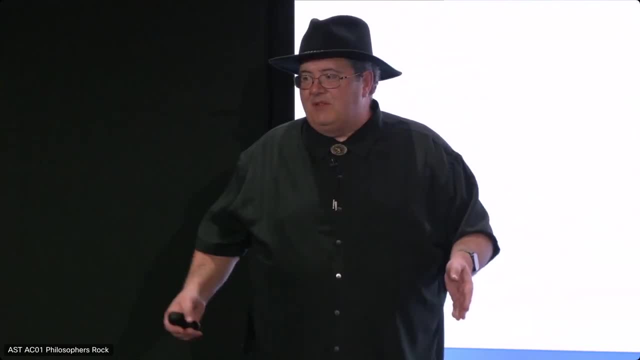 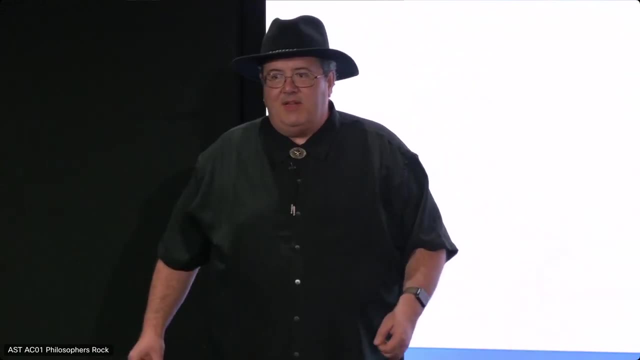 But that's more. you ought to go to the studio team to say when that stuff is ready, because we're just waiting for the api's to be there For us to be able to hook this stuff up. we know what we want to do. we're just waiting for the api's to be available for us to actually do that- the hooking it up to it. 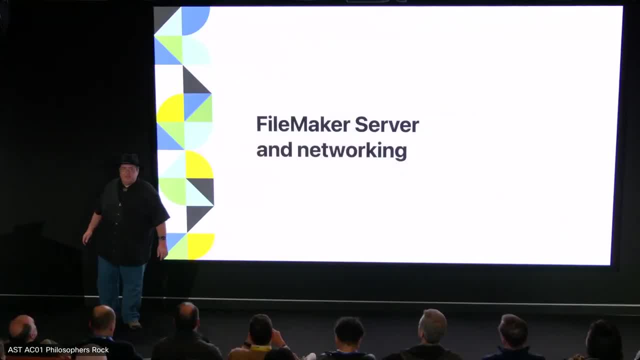 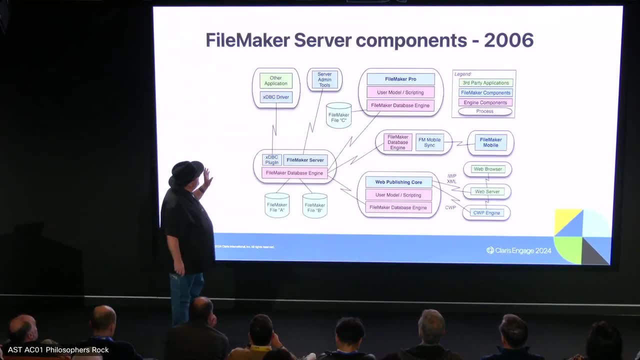 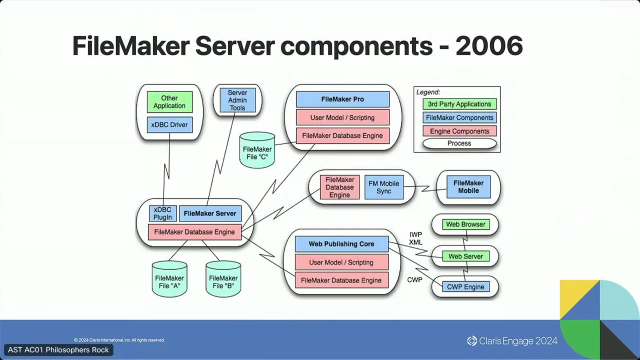 So now we go on to the filmmaker server and networking issues. first a little quick history of older slides of mine. so in 2006, this is basically the file maker, what the file maker server was all doing. we had one, They see, very monolithic file maker server. it loaded plugins which made it kind of fragile of a plugin cable. 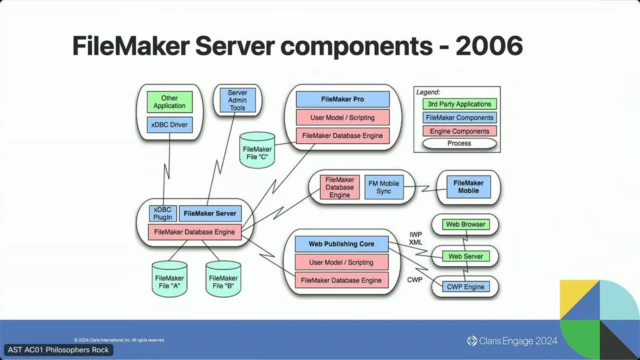 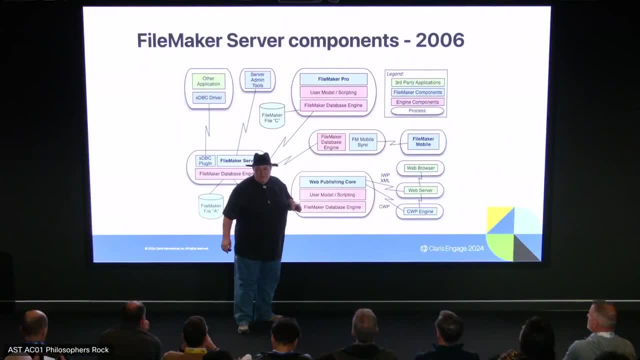 It was a problem. xdbc was actually implemented as a plugin and not a separate process we were using. oh yeah, we actually supported palm devices and newtons at that point, if you guys remember, And we had the web publishing core. this is when we were doing a instant web publishing. this was even before web direct. 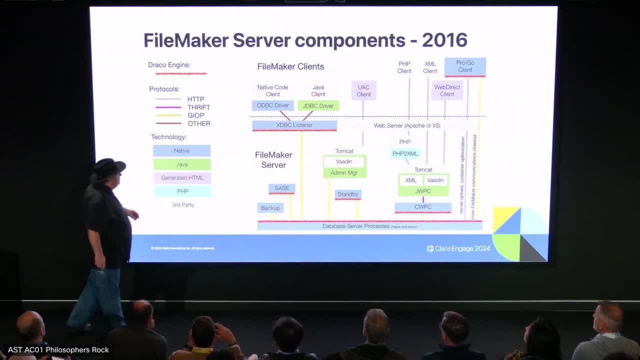 Ten years later you're getting a little bit more modern. We tried to move more things out of The database server process, like backups and sassy and the standby logic. the xdbc listener was outside there- these little two brown lines up here. lucy mentioned about how we improved the security of of the xdbc. these little brown lines, which is this custom protocol, is what we improved. it was using md5 before and that's a known security risk at this point, so those lines are updated. 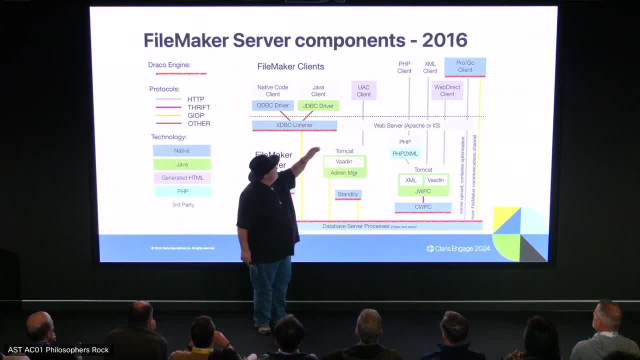 We were using. So we were using java here pretty heavily. with the uac client we found out that widgets were not very stable between different versions of java's. every time you updated java the uac would break In over. here. We still have the main file maker protocol going back and forth on port five thousand and three, but we were starting to use https to do container downloads if the containers were stored as external files. so we 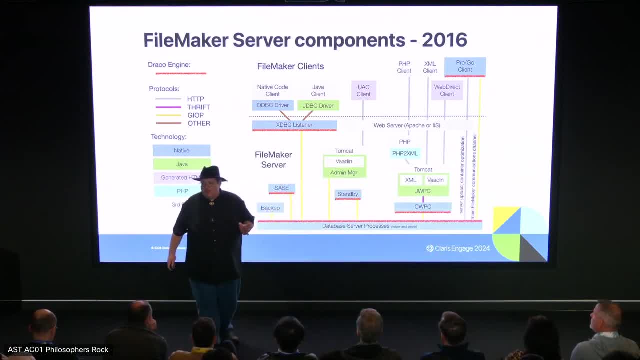 Wouldn't go through the file maker server Process. we could just talk to the web server. the web server would then know where those files were stored on disk, since they weren't inside the file maker database itself, and you could download it directly just using the web server to do the the file. 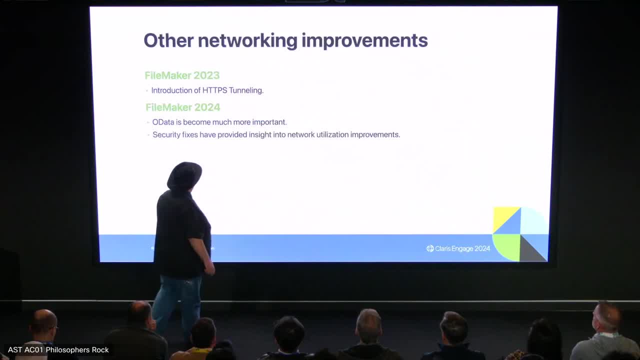 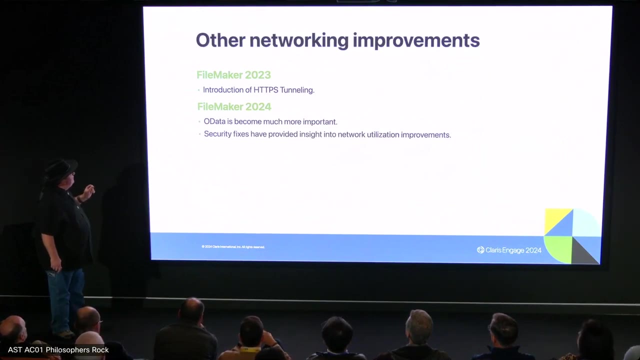 I go. So in file maker twenty twenty three, we introduced https telling it's only on obon to twenty two. right now. I'll talk about those reasons a little bit more later. in twenty twenty four, And actually in twenty twenty Three, We've been starting to move, oh, data to be four, point, oh one compliant. 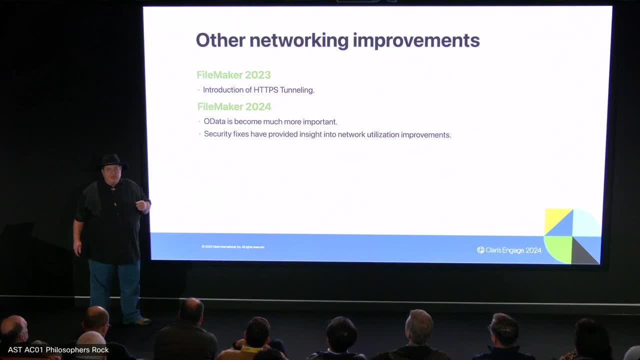 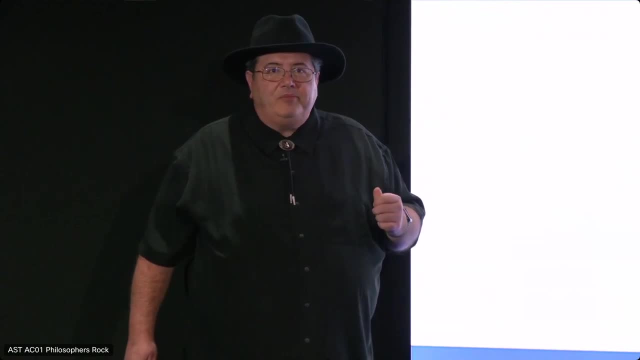 It's not quite all the way there but is our goal to make it fully compliant in the next version Of the first version of twenty twenty four. the We're implementing dollar select and dollar expand in the thing and so this gives you the ability to do things like inner joins and left outer joins to kind of match the same capabilities of the odbc driver has. 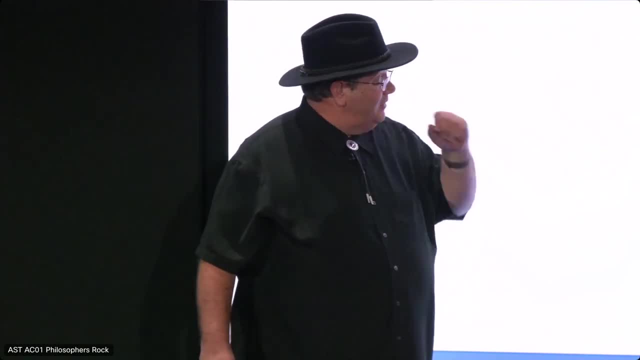 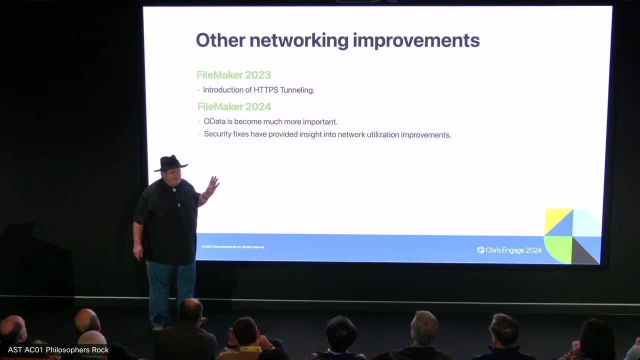 And other things. The security fixes in this apple team that lucy was talking about Fixing the stuff that they've been telling us about- and just then makes us look at what's going on, even finding things where we can optimize the opening and closing process of file maker. 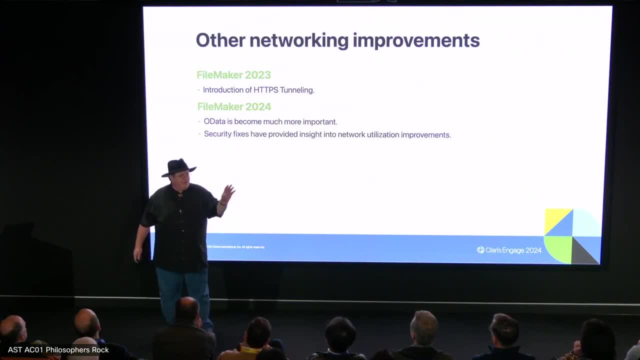 We know. so when you were you were closing down the file, that it was actually starting to log out and start shutting things down, and then something at the end would ask: oh, I need to update that too. so then we download again, updated and uploaded, and you know it's like, oh, that was doing things in wrong order. so 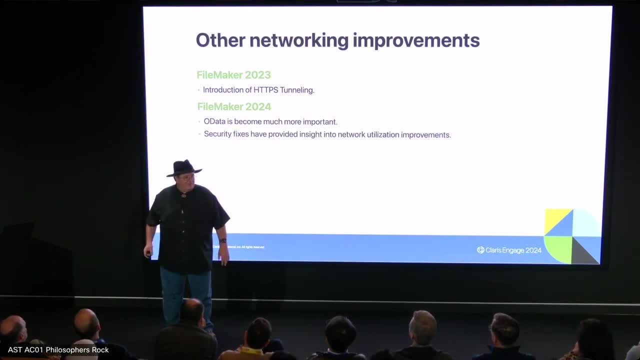 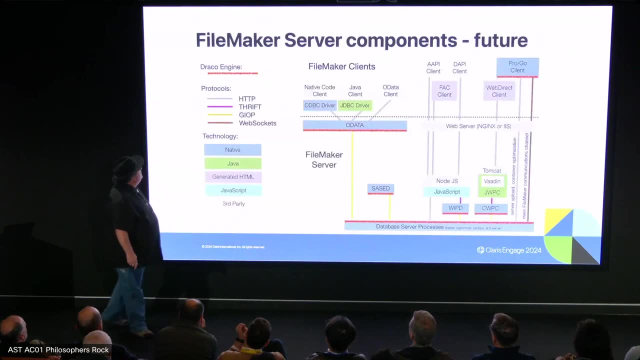 We're rearranging seven. we're Actually looking at what's going on, because over these number of years things have just been getting crafty and I mean it all works. it's just not optimal, So This is not necessarily file maker. Twenty twenty four: 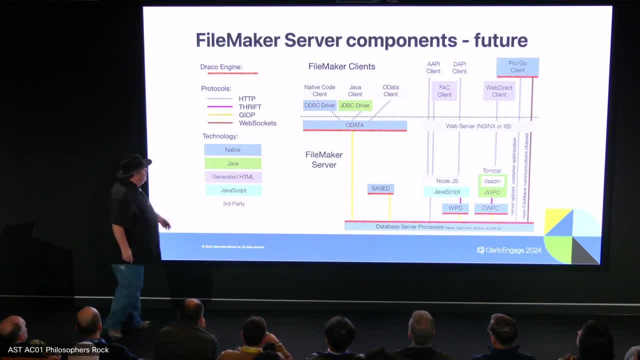 This is kind of like the future that we're shooting for. What we want to do is actually just get rid of the xdbc listener altogether. we want to make oh data as our main data source for things like talking directly with oh data. The. 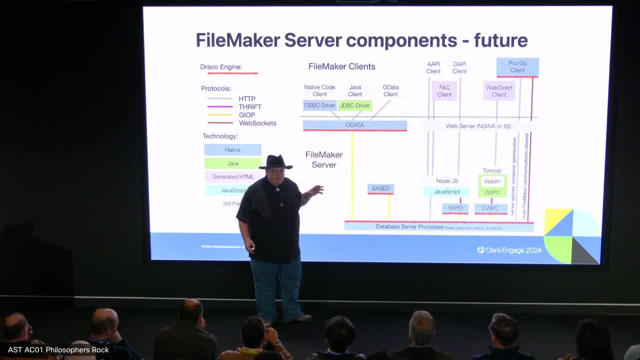 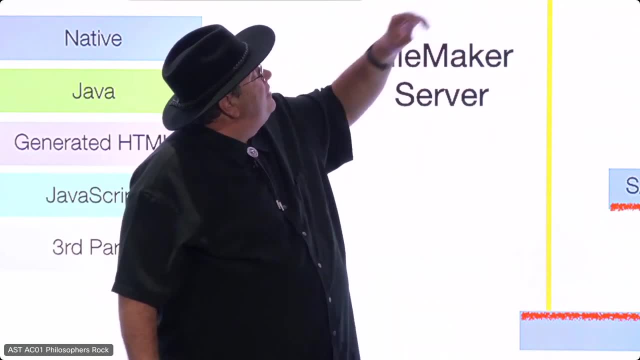 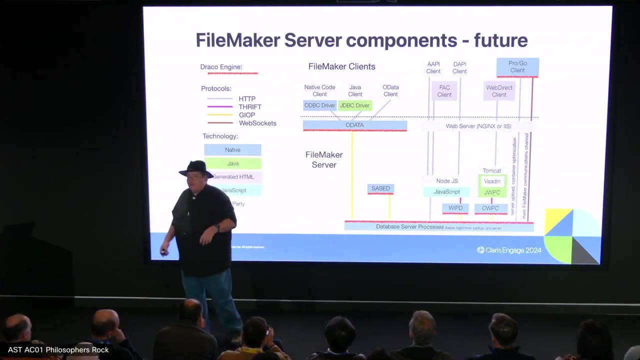 Dbc driver will be one of these drivers that they basically take sequel statements and oh dbc api's and just convert them to oh data directly. same with jdbc. now you can purchase drivers that do that. right now there are drivers out there that do this type operations if you want to talk to oh data and you need to give it an old oh dbc api to it. but ours are going to be, ours will be slightly different because we have, you know, some additional features for accessing container data and stuff like that. that's really nonstandard that we're going to have to do. 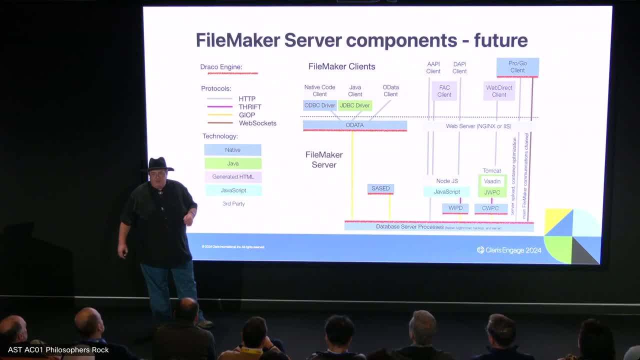 So That these other products out there wouldn't be able to support. they'd be able to support, you know, regular straight table data, but not some of the additions that File maker does. You know, now we're using the, the, the fac that that you, I, which will be showing is now, all you know, react base, all using no js underneath all using javascript. we got rid of java completely. in this state we still are using java to run that and which is kind of the core. 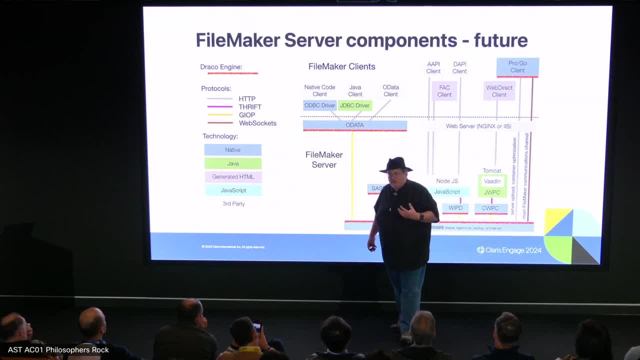 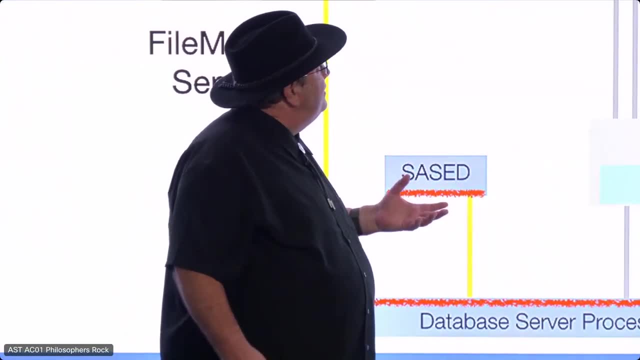 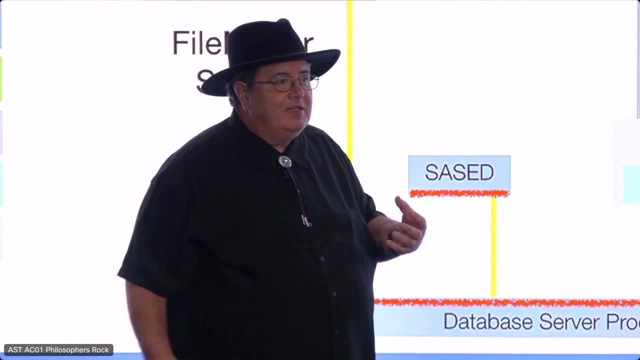 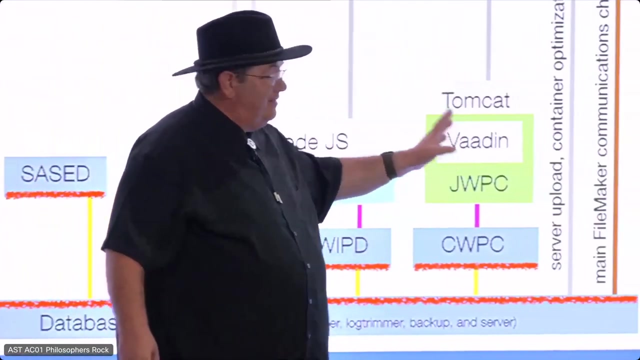 For web Direct for doing that, the user model. inside there is the java process that's generating the html pages that you're viewing. We'd like to get away from that and there is some work. we're taking some of the stuff being learned from a clara studio for how to do pages and stuff like that and and some of the infrastructure from inside there to start working on the eventual replacement. but this is this is going to be a pretty big job. this is not something twenty foot twenty four that's going to change by that point. 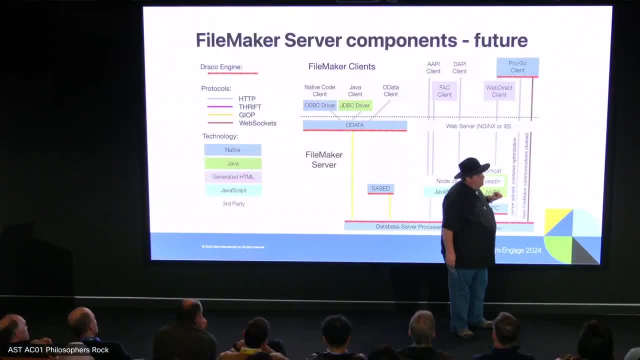 The other thing is that will probably be Trying to move more to the http model, where http telling is actually using web sockets to communicate. it's really not using https as the protocol. Ideally, what I would wanted to do is use http two, which is the new modern standard for doing bidirectional communications between a server and a client. but proxy support for http two is a little bit spotty and there's some out there that work. there's some people really. 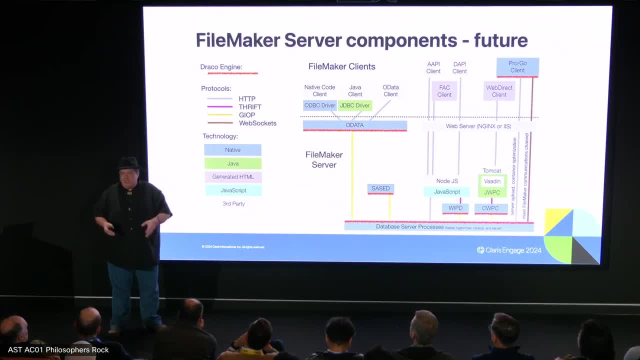 Poo pooing http two Because of how it can't have multiple channels communicating, which web browsers really want to do. we don't need that because we just have one thing that we're going back and forth on, so that problem isn't a problem for us. but if everyone 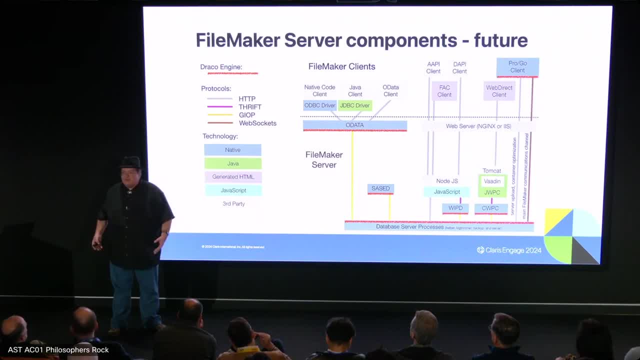 Else doesn't start using http two, then all the tools and all the infrastructure out there won't be there to really support it properly, so we may be stuck with web sockets. but that that's like a direction I want to go in. really want to use the new definitions. 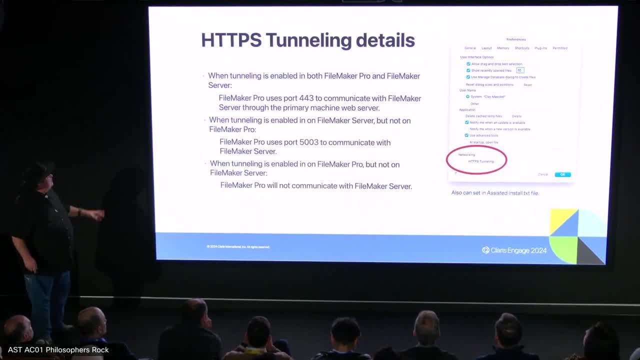 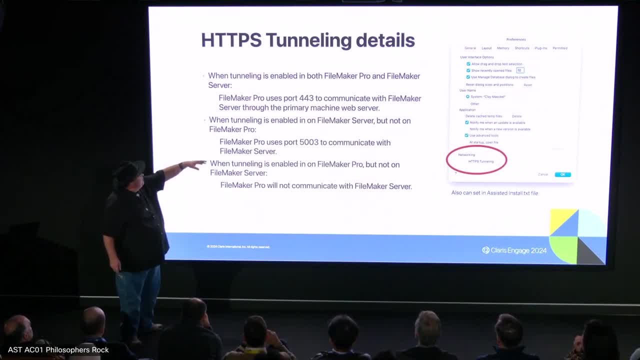 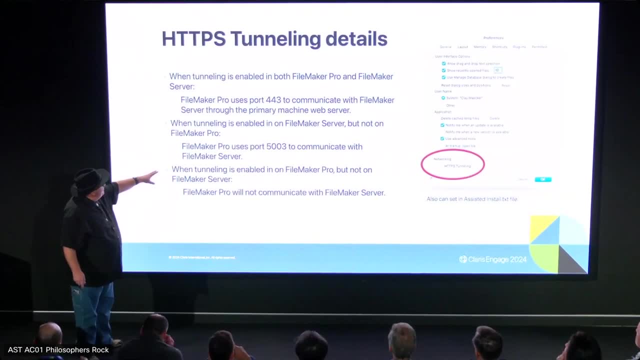 When it's enabled, Filemaker pro uses port 443 to communicate with the server through the primary web server. If you enable it on server but not on pro, Filemaker basically falls back to the old protocol using port 5003 and using the g i o p protocol, basically layered in top of a raw tcp IP stream. 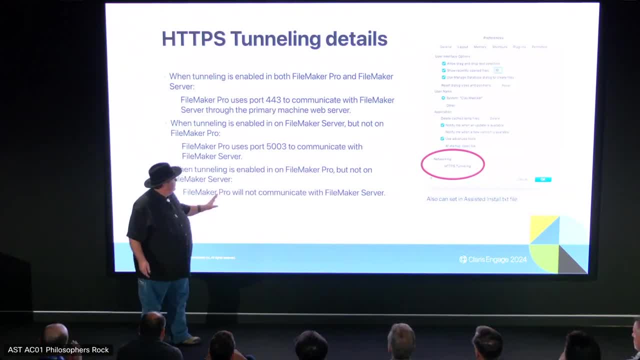 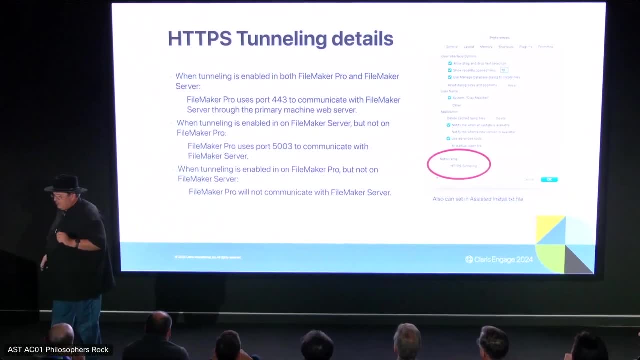 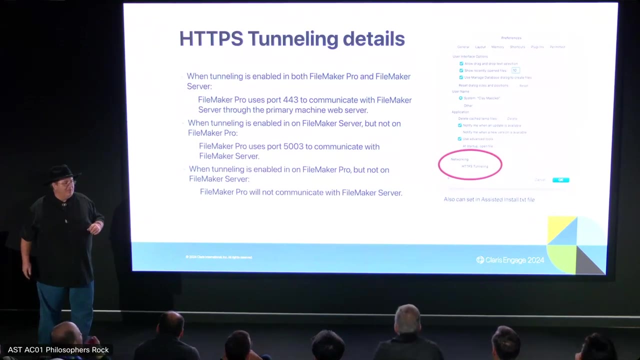 And telling is enabled on probe but not server Pro and not communicate with server. So One of the reasons for this is that the, The notification or the other negotiation process that goes on when kind is connecting to server, is pretty complex right now because 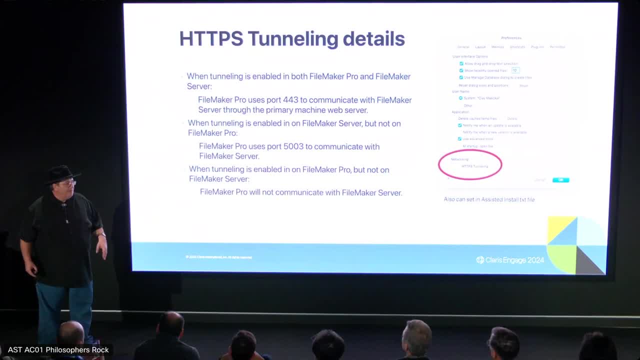 It has to see whether you can get an SSL encrypted tcp IP stream and then, if it's not there, then it tries doing without TC, without Encryption, and then has to negotiate whether whether the files read only or rewrite, and that's like a four step process if we have to start. 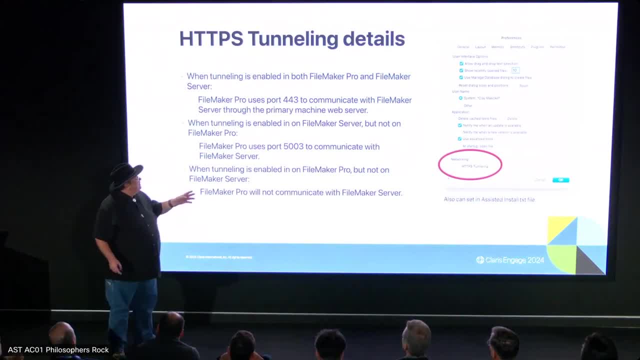 Peening to see: oh, can we, can we talk with going through HTTPS, or do we need to fall back? then that multiplies that by two. so then we're up to eight negotiations that have to go on during the connect process. So in filemaker. 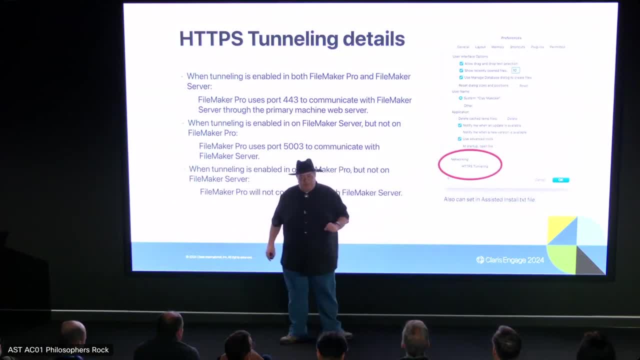 This circle is just showing where you enable it in the pro products and In the main app setting. Something that would help here Is we can cut down on these negotiations If we can like. stop peer to peer serving. I mean, we've been trying to kill peer to peer. 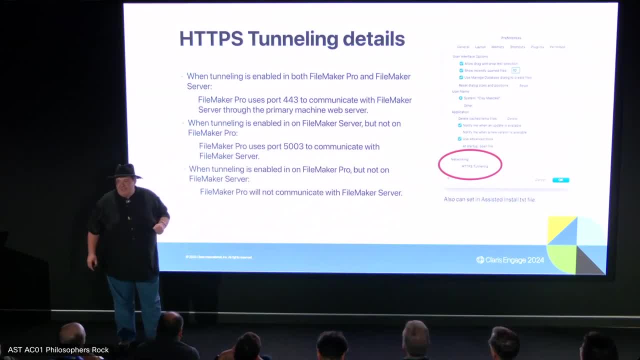 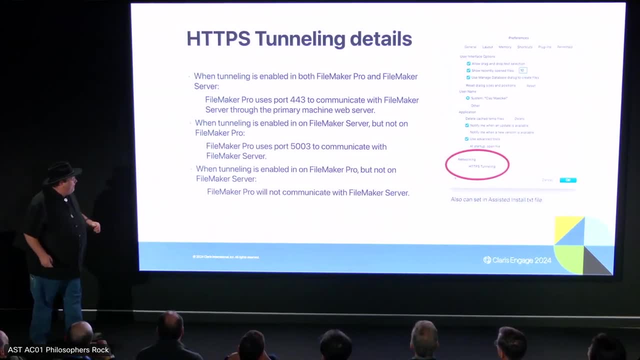 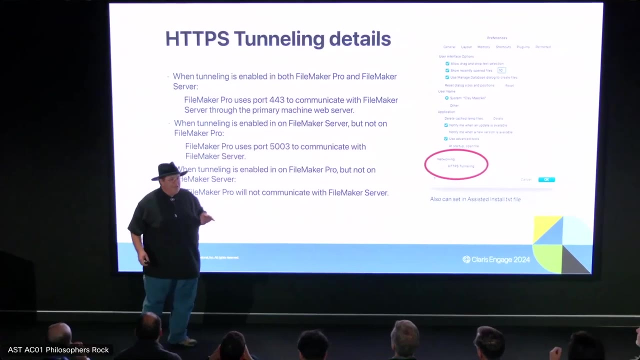 For a long time. There's people at screen when we try to kill it, but Maybe someday we'll just ignore them, I don't know. And also because because to do the HTTPS telling you actually have, you really have to have a web server. 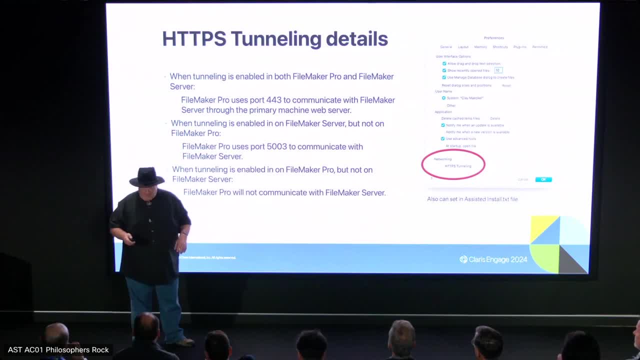 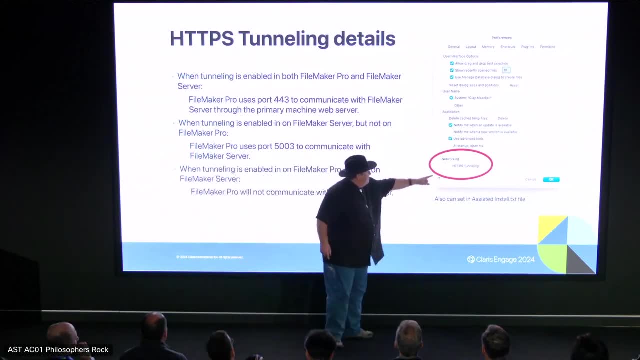 You can't do it without you to handle all that, to handle the negotiations and Do the proxy work and all that stuff properly. Oh, I keep forgetting about that little text. You can also put it on your in assisted install text file. so if you're doing a bulk installation and you know everyone is going to be using the HTTPS, you can do that and have it turned on by default at installation time. 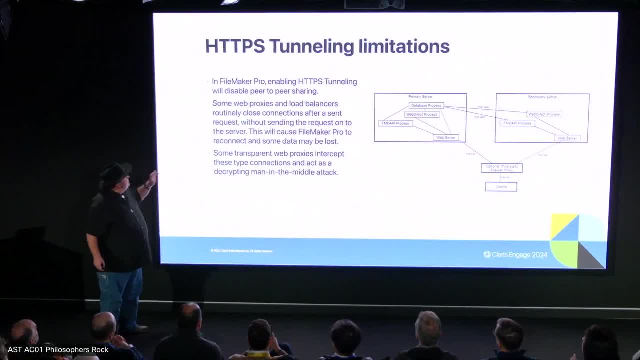 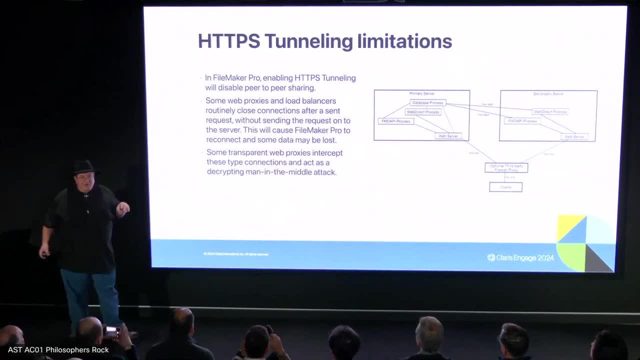 Limitations, that HTTPS telling, like I mentioned, you can't do peer to peer. Some bread proxies and load balancers out there Will only leave the proxy running for like maybe 30 minutes And then it just resets the connection completely. just I don't know why, but 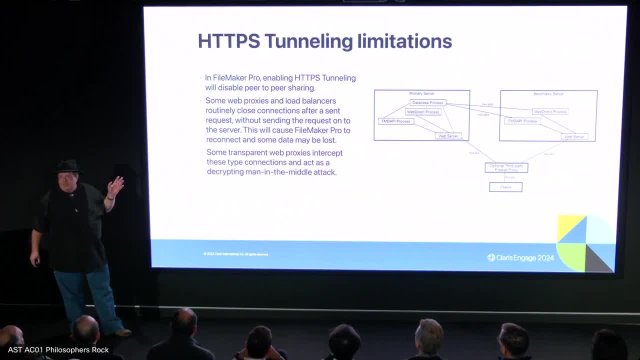 So this will make family, or do I reconnect? at that point you'll notice that oh, the connection went down, we need to re enable it And then the file maker will do that automatic reconnect, as if you got a disconnection because the cable got pulled out and push back in and stuff like that. but it's still not ideal. 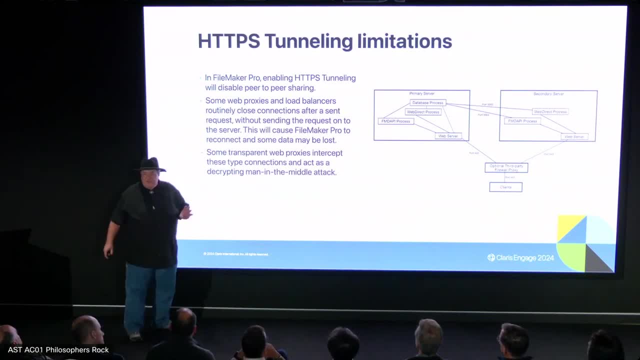 You want to check with you know your proxy vendors and your load balancers and make sure that they keep web socket connections up all the time while it's running. You don't want it Going through resetting it regularly. And since you're going through a proxy, you have to realize that that proxy can be looking at all the data going in and out of it. 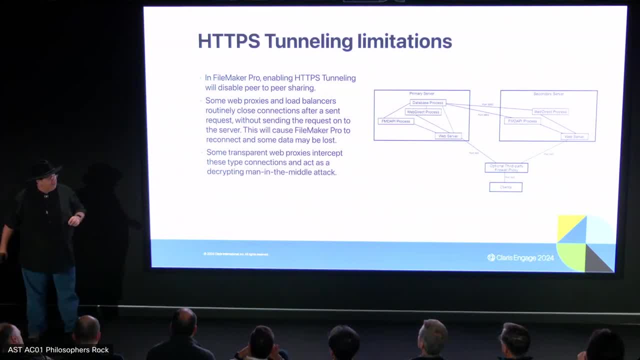 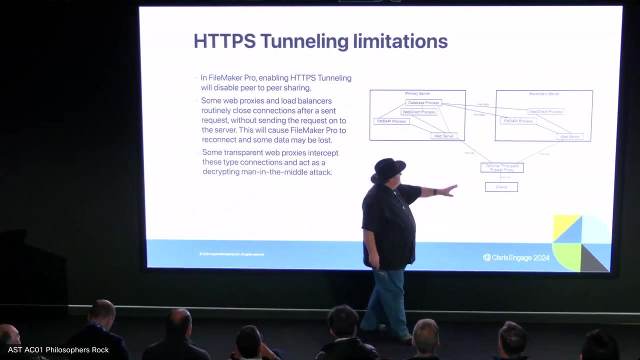 They can set up other security certificates on both sides. So hopefully you trust your web proxy vendor- or your IT department, I guess, here, which is the one that installed the web proxy server, And there's a little diagram over here. You see, the proxy is outside the servers. 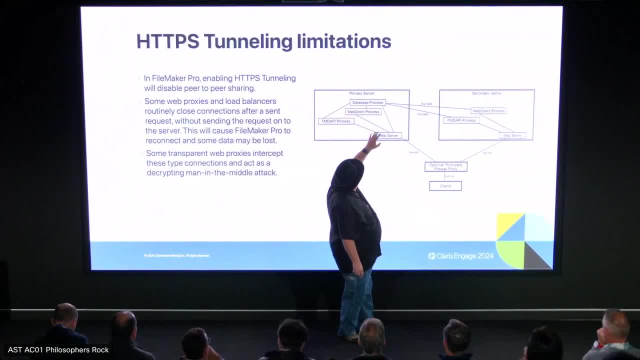 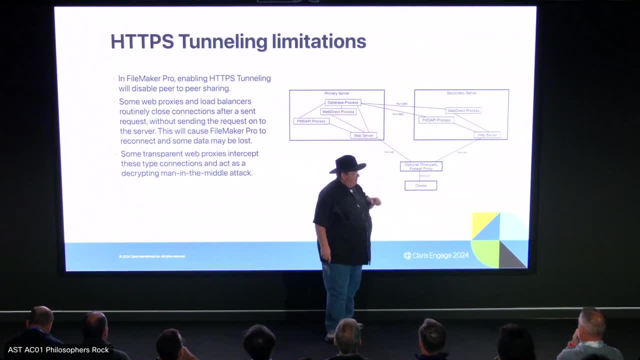 The kind sector that they use ports 443.. To talk to the secondary servers in the primary service, But file maker internally is still using port 5003 for all the processes behind the behind. there is faster, We don't have to go through the web browser. 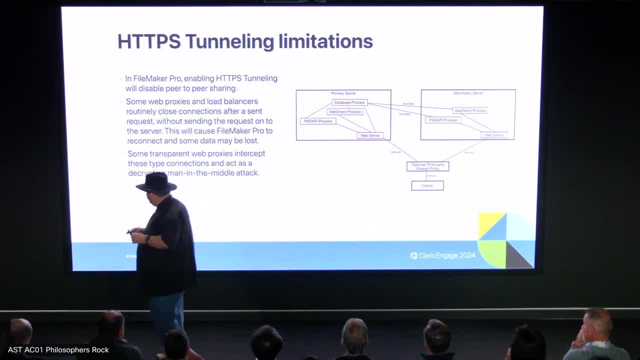 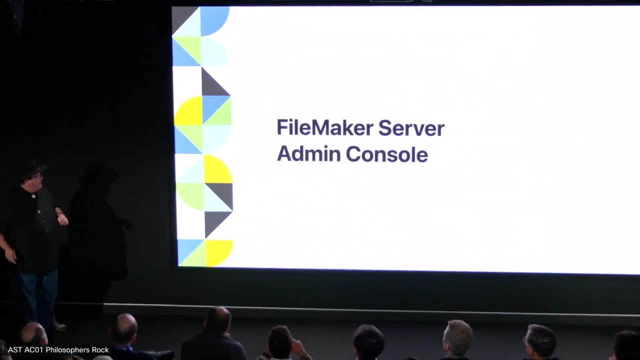 We can do process to process communications directly. Yeah, we're getting. we have some other time pressures coming up and I'll get to that at Q and A, So I'm going to go a little bit more quicker through this. the server admin council. 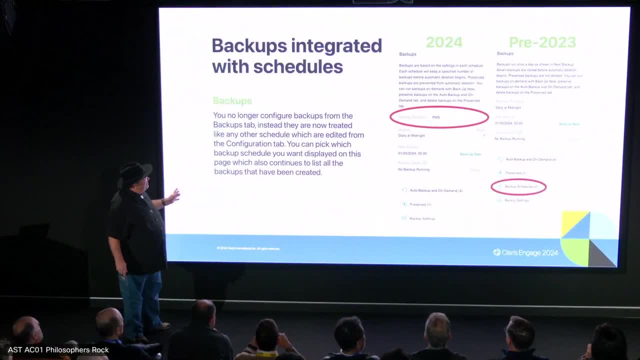 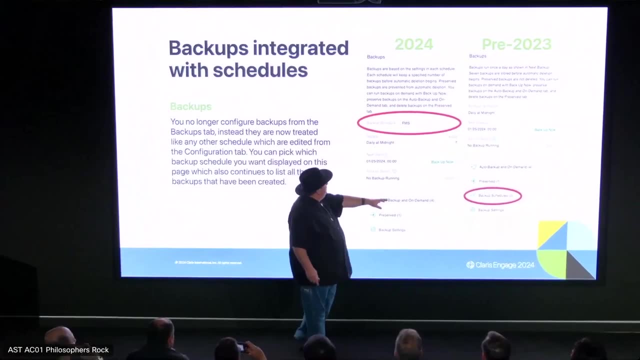 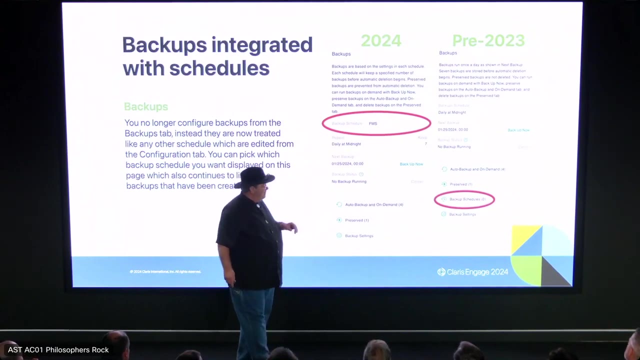 Backups are no longer a separate task: backups and now schedules. So you see what the new I look like before 2023 and now in the new version, You'll be able to see you pick the default schedule. You can see any specific, particular backup schedule in the UI here. 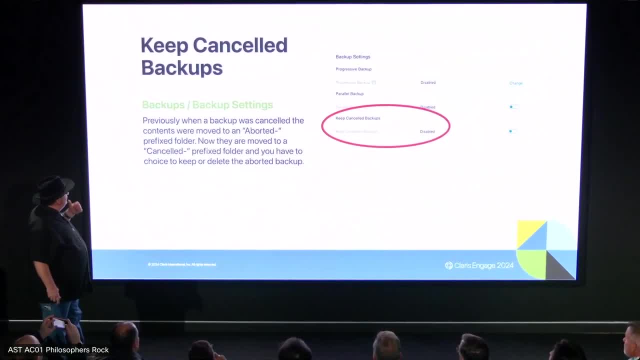 We're trying to hopefully won't change this anymore, But prior to nineteen point six, backups- where they were going, what they were named- seem to keep Changing all the time. You know they they were. when backups are canceled, They were put in a border folder and now they're put in a canceled folder. 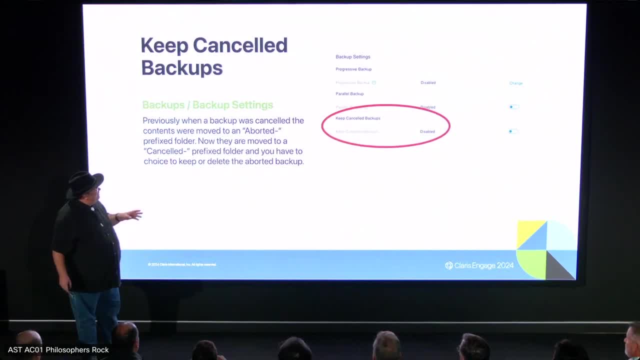 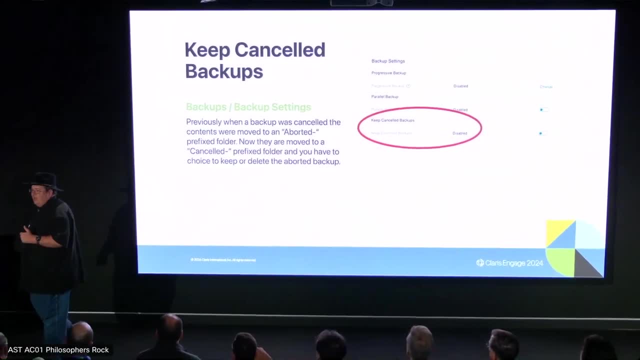 Some versions would delete the canceled backups, Other ones would leave them around, but now we give you a choice, So there may be a reason that you may want to keep a canceled backup, because, you know, maybe it's like a eight-hour backup, because you have. 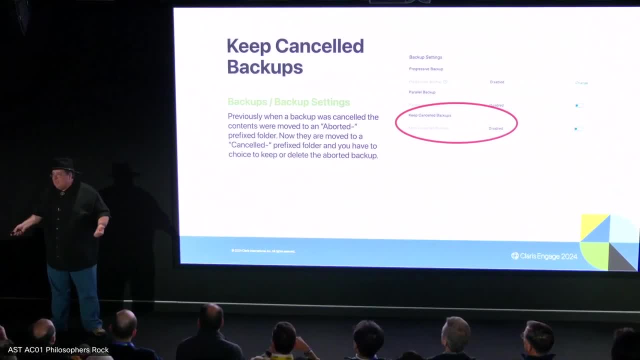 you know, terabytes of data You're backing up and maybe it succeeded with four of the files, but you just couldn't wait for the last file to be backed up and you may not want to dump Them all, because if there are some cassette catastrophe- 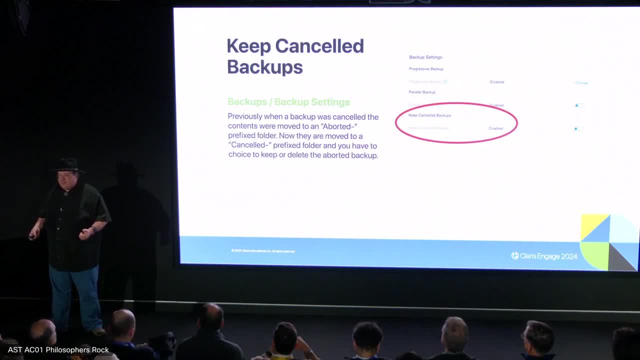 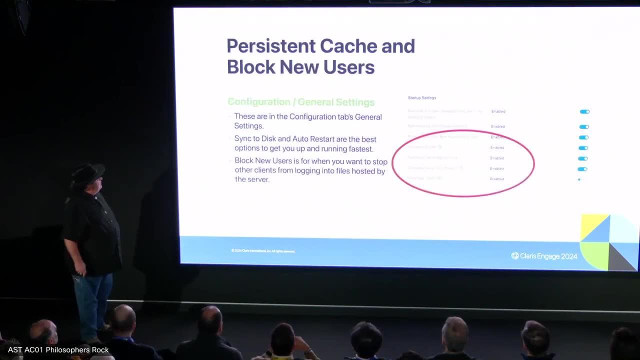 you, at least you know three quarters of your data will have. you'll have a nice clean backup of it. So it really depends on your use of you know how big and how much, how long you're waiting for this stuff. 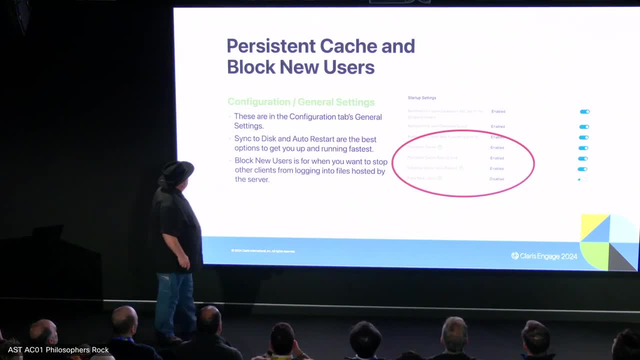 Configuration systems. So this is where persistent cache is turned on. We've been playing with it. We've been fixing some bug fixes since the twenty twenty three. We're a lot happier for how this is. Basically, what the persistent cache is doing is that we're using 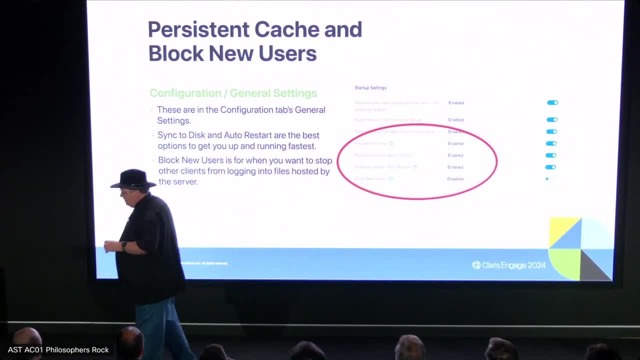 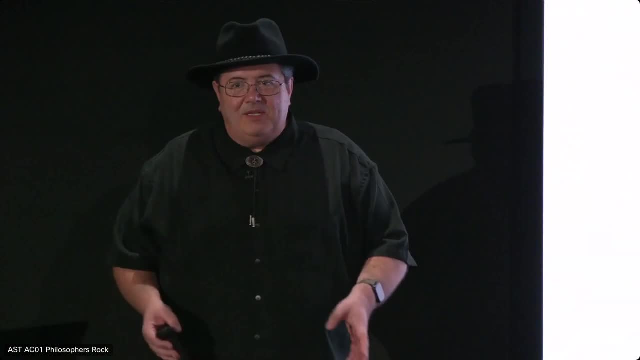 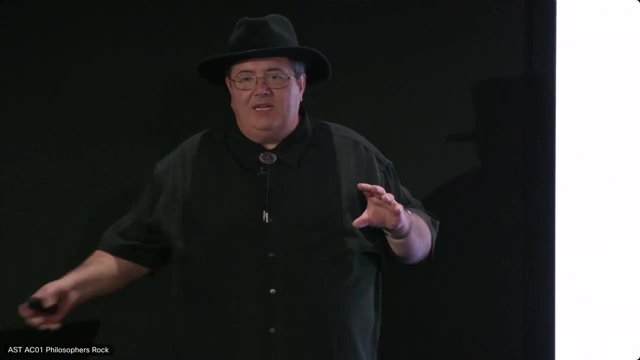 memory mapped file, backed memory allocation. So we allocate a block of memory and then we tell the operating system map this to this file. So the operating system is basically, as we make rights to the our cache blocks internally, it in the backside is doing and writing it to disk immediately. 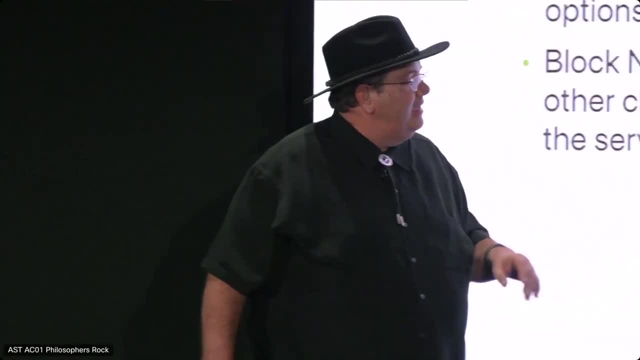 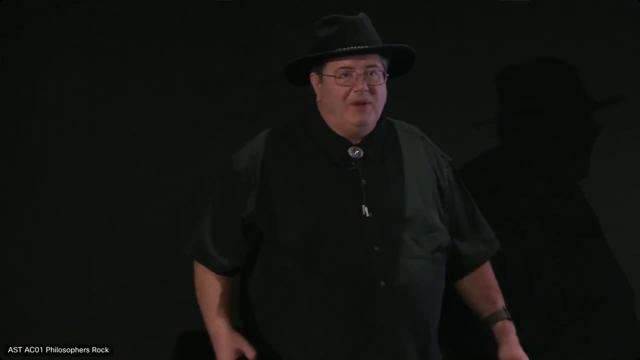 And when you turn on the sync to disk, that we tell the operating system that we want to register the disk almost immediately Whenever there's any change, whenever the virtual memory manager detects that a block change, that will then do IO and write it out immediately. 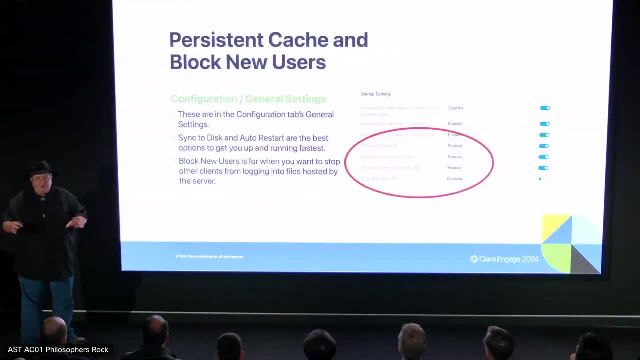 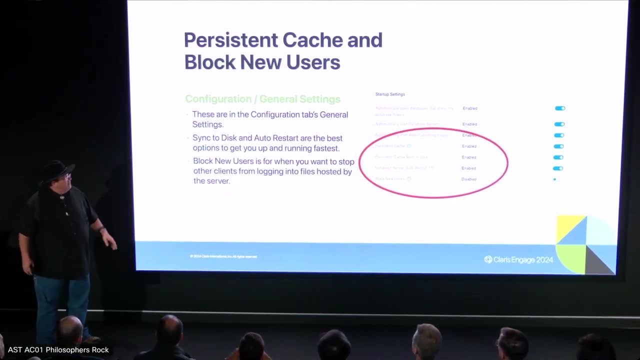 And the auto restart is saying that: well, that's so the reason we're doing that. So we're writing all the in memory cache structures that we have inside server to disk. So if the server process gets killed or crashes- which we shouldn't anymore- 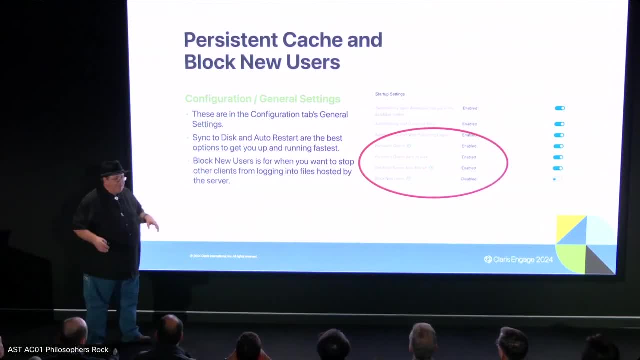 or you know, or you know someone does a server shutdown that you know forces OS to. you know want to shut everything down quickly, So then it just goes through and does a bulk kill of all processes. The what was in memory will be on disk. 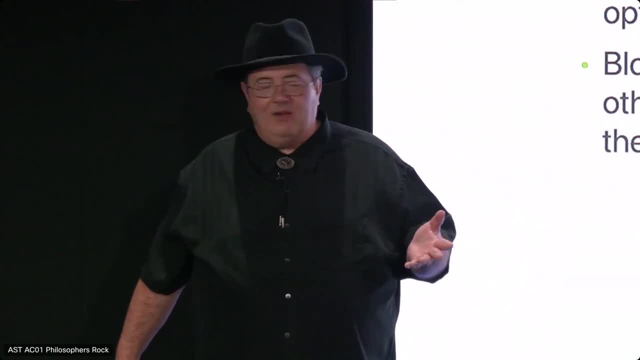 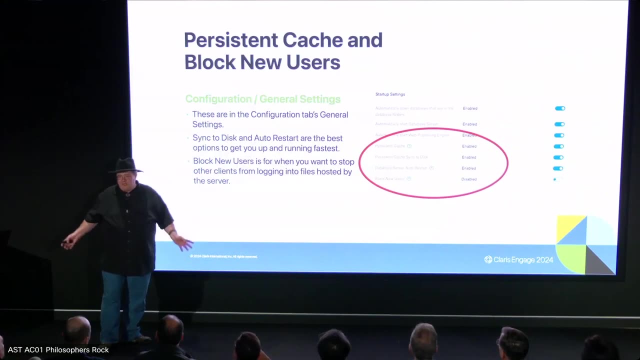 And when the server restarts it'll look for these files to see if they're setting there And if the auto restart is on, it'll use that to reconstruct the cache and then basically continue at that point Finish flushing things out to the files properly to get nice clean files at that point. 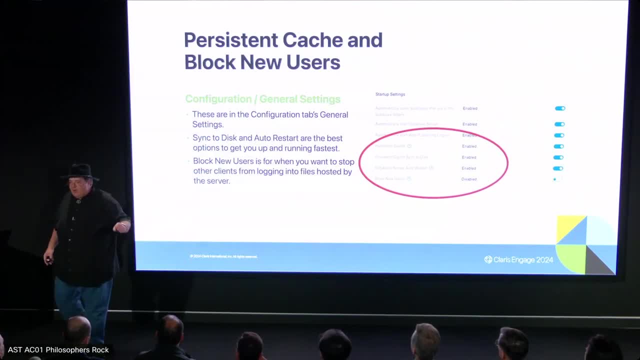 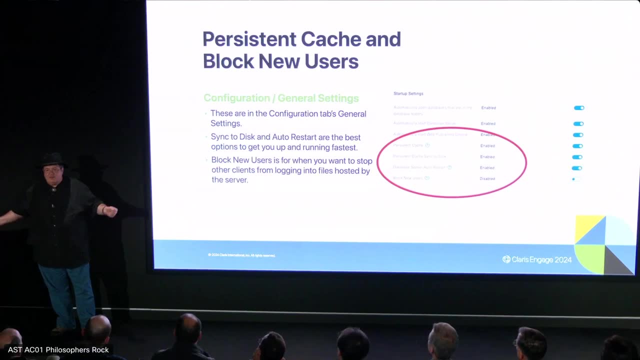 This does not help in the case where you pull the cord out of the wall because we're depending on the, the operating system, to get it to the disk And there's nothing we can do if it's in process of going to the disk. 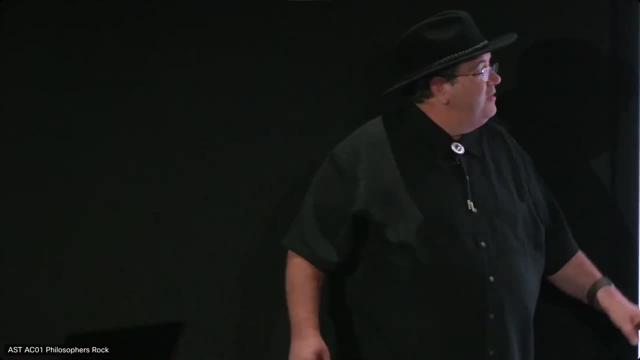 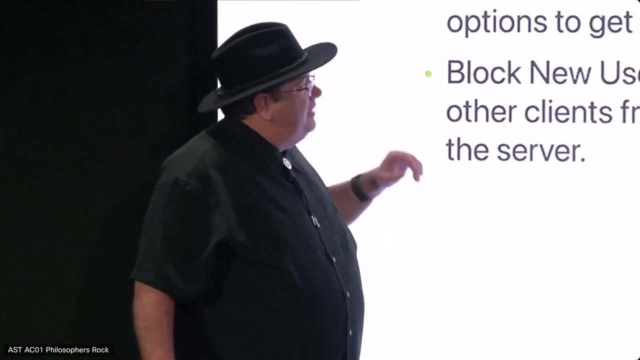 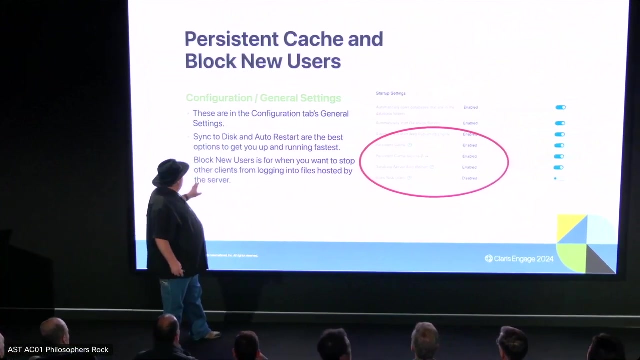 and then, like, the disk blows up or the power disappears. So this is really for, like software style errors, And syncing to disk immediately is a little bit slower. but we're I think we're going to start recommending that you turn that on. 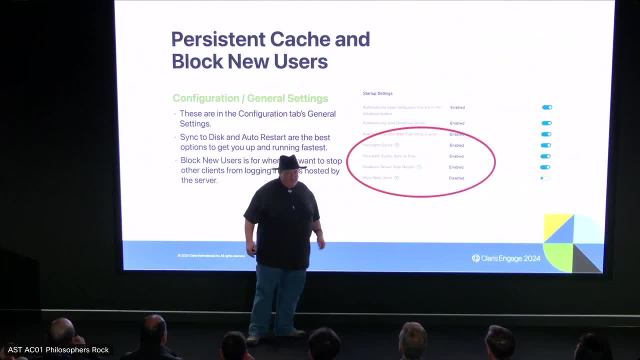 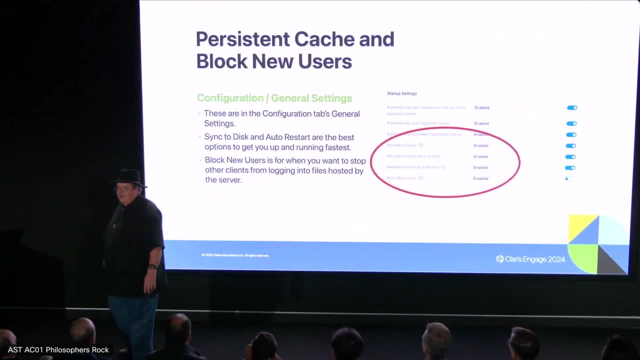 Another new feature is block new users. This is good for people doing maintenance, So you may want to log in. you kick off users that you don't want on there anymore because you want to scan something, You want to make a well. 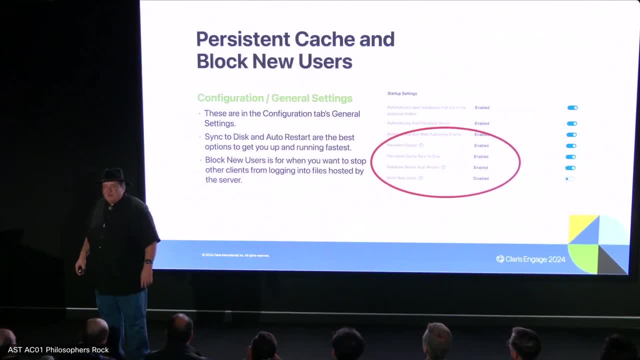 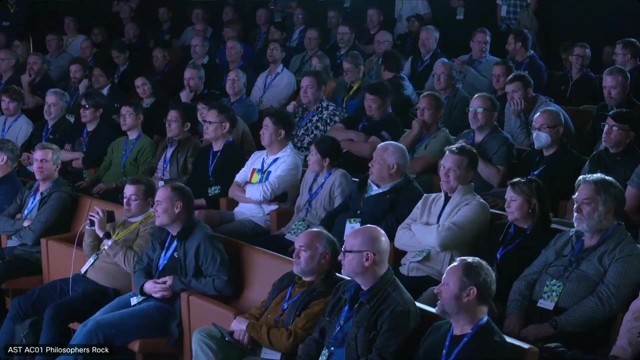 you want to do a live update where you don't want people logged in at that moment, So now you can turn that on So no people can log in while you're doing your your stuff because you don't want to use it. You probably really should be using the migration tool and do the whole dev staging and 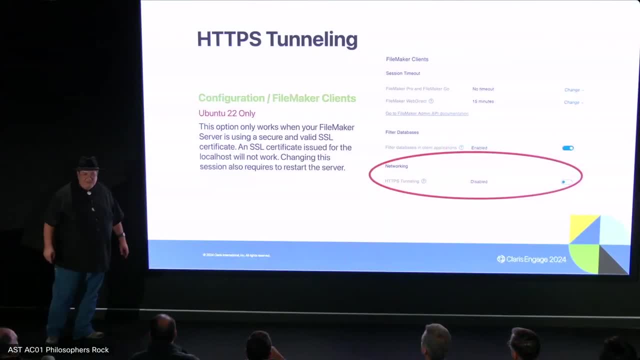 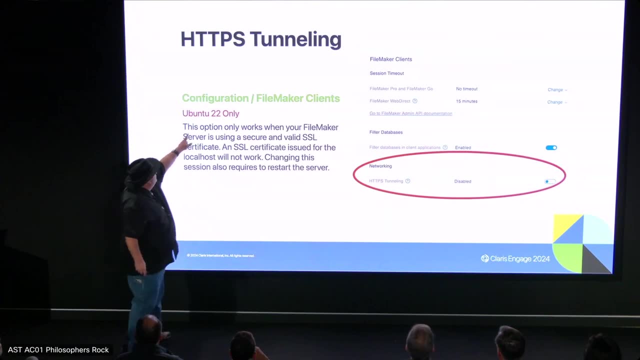 but you know you have to do hot fixes sometime. You know you, your customer just won't wait. HTTPS telling: this is where you turn it on in the server UI. Remember it's Ubuntu 22 only. Note that we're really starting to use Ubuntu as the main server development world. 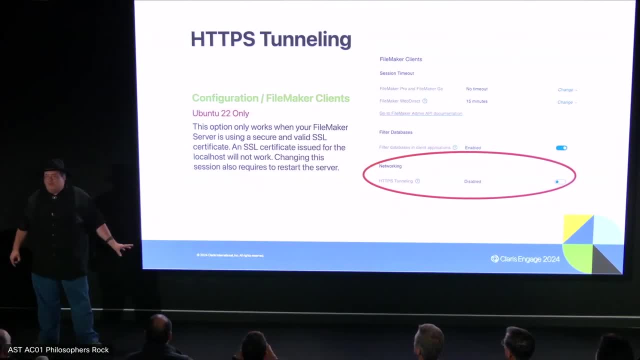 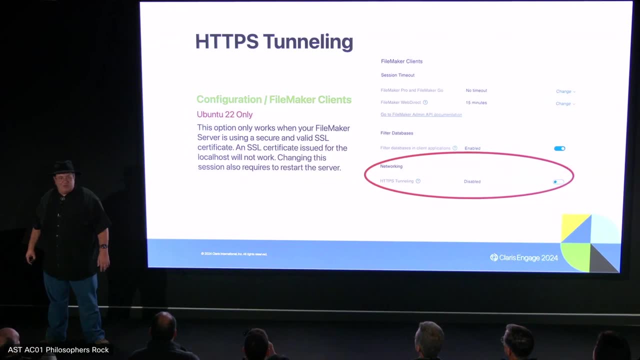 Where new features that come out will be Ubuntu 22 first. You'll probably be the most tested. We really want you guys to move to Linux servers. I know there's some Microsoft only houses that won't let you run any Linux, and you know. 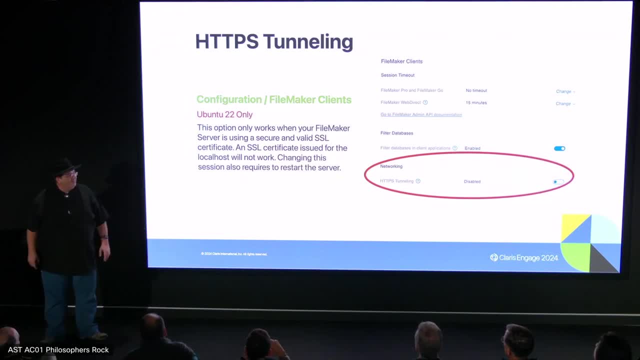 that's an evil word to them, The Mac OS. we try to kill it. but then, you know, Apple says: why are you, why are you dropping our support? And then I asked him: when's the last time you sold a server software and server hardware and stuff like that? 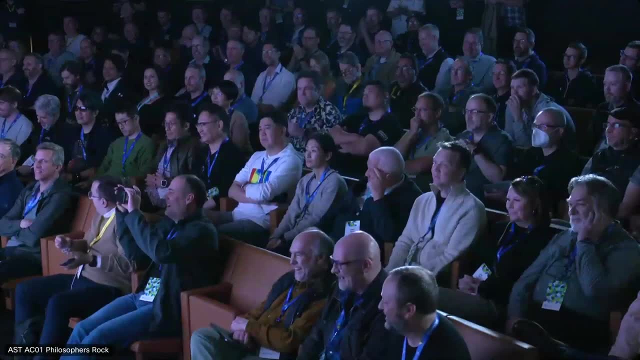 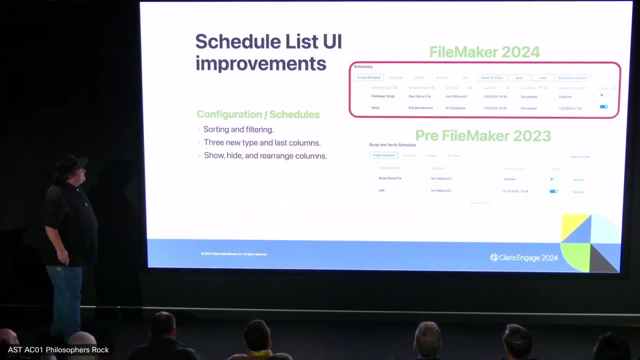 but a Mac Mini is not a server. We're doing scheduling improvements. You know, pre FileMaker Pro you only had four columns and some options here, So now you get a lot more columns. I mean, there's more. there's three more fields in there. 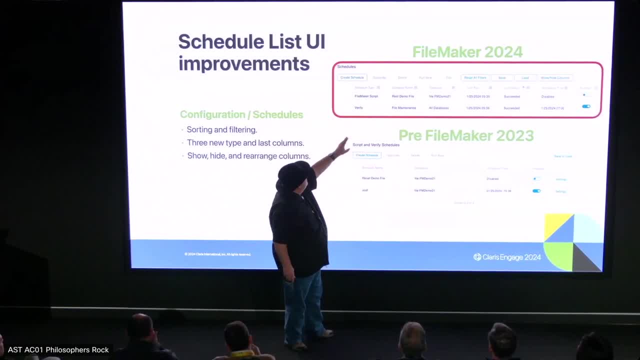 You can now rearrange the columns. You can show hide columns, show columns, sort them, filter them. You have, if I know, some, some of you guys out there have like hundreds of schedules and stuff like that, So it's now a lot easier to manage them. 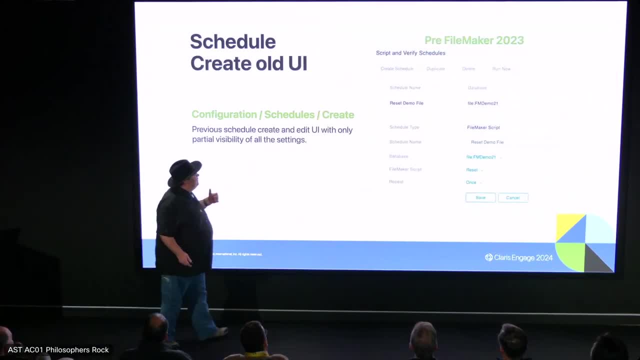 So prior to 2023, when you created a new schedule. it's kind of limited. It's kind of like how FileMaker work: You had to drill down into multiple dialogues to go through and set Things. The new version: 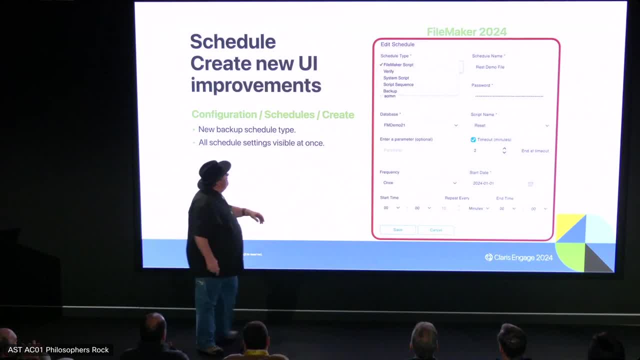 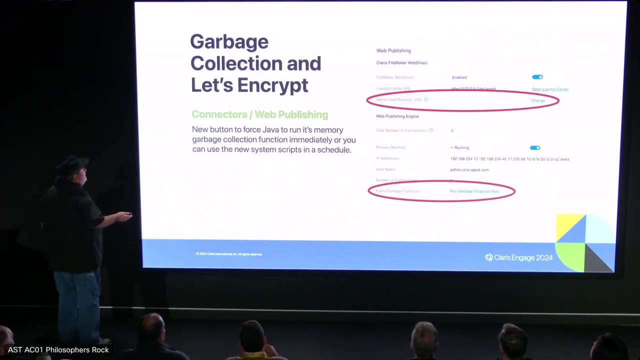 everything is in like one panel And you can see backup. now is a new schedule type, So backup is not in another area. It's now all built into this schedule. So you, it's just schedules for one thing, Garbage correction and let's encrypt. 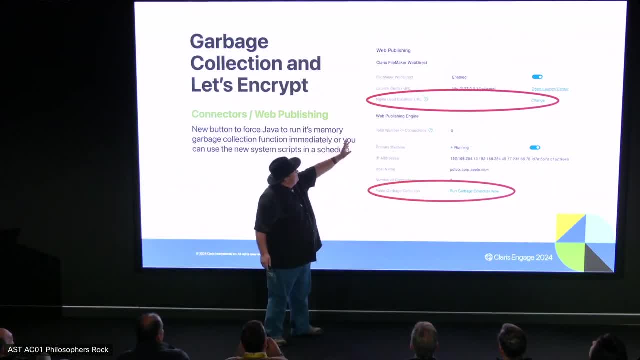 Oh, actually, for you know. you know, NGINX? this is where you set where the load balancer is actually located that you wanted me to use. Here you can force garbage collection. I don't know how often people will use this, because I'll show on the next panel what you probably will really want to do instead. But if for some reason you want to toggle the garbage collector to run, you can do that there. So here in the system scripts- we now have like three new system scripts- You'll be able to run the garbage collector immediately. force the garbage collector to run on secondary servers. 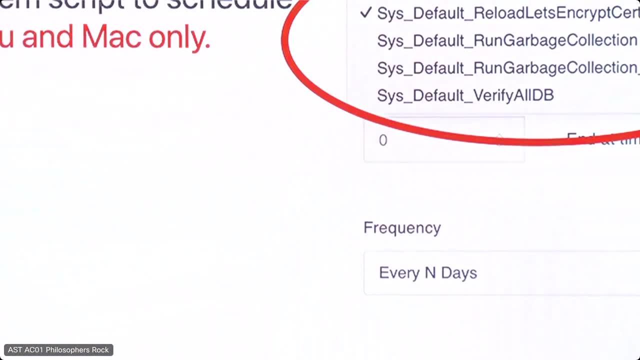 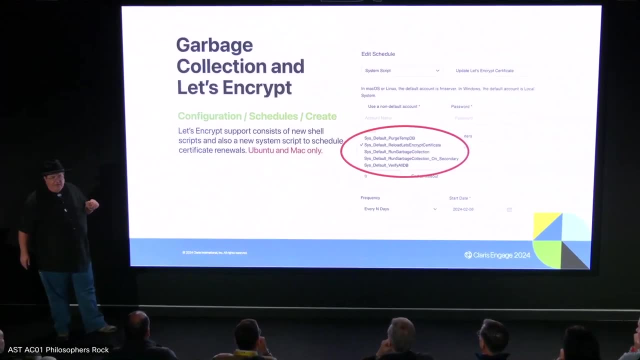 And we're bringing- let's encrypt the certificate support to the server product. Now it's only going to be on Ubuntu and Mac first. There's really not that much UI other than that in the server. We're supplying you the scripts that you need to run and instructions of all these other services that you have to download and install. 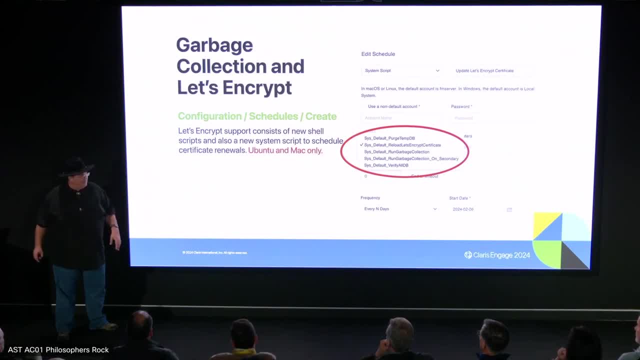 Basically Unix, Unix style services to actually get the certificate And to install the certificate. the plan is to eventually maybe roll this all more into the UI so you don't actually have to run shell scripts to set it up initially, But what you'll be wanting to do, since, let's encrypt, certificates always expire after 90 days. 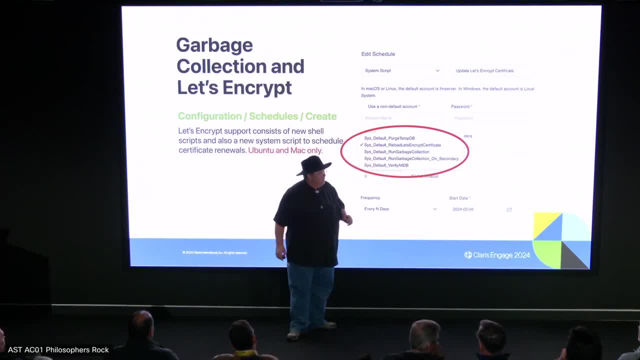 you'll probably want to have your default reload certificate script run basically at 80 days and stuff like that, Because you can't update the certificate. I think under you have to wait at least 60 days or something like that before you can update it. 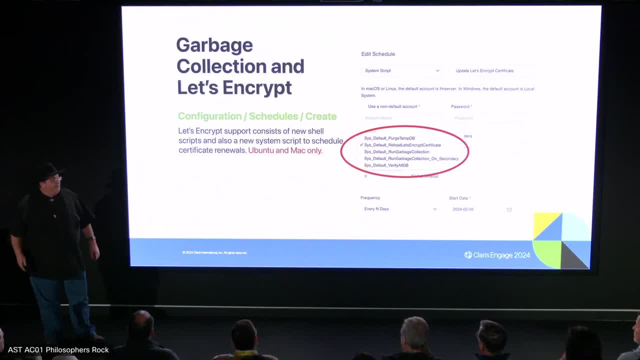 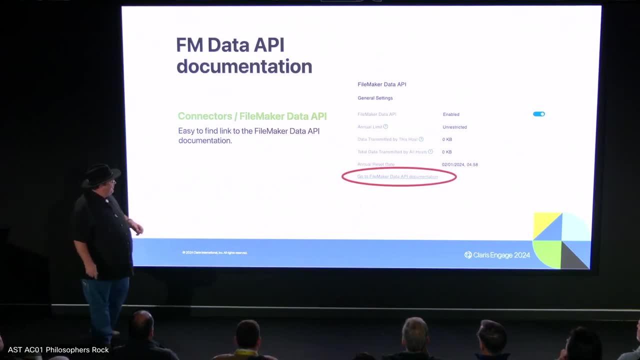 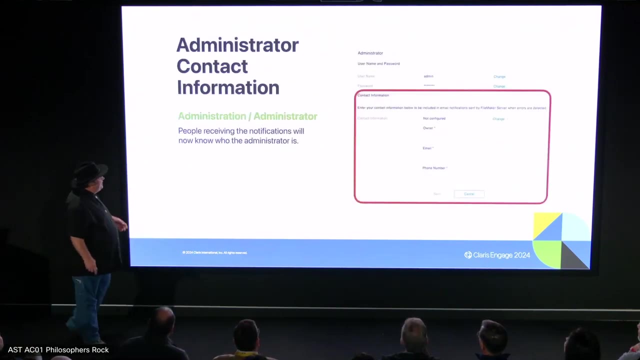 There's a window where you can do the updates. I may have the numbers off, but that works like that. I like this because I can never remember the URL to get to the file maker data. I also don't like any notifications from the server. 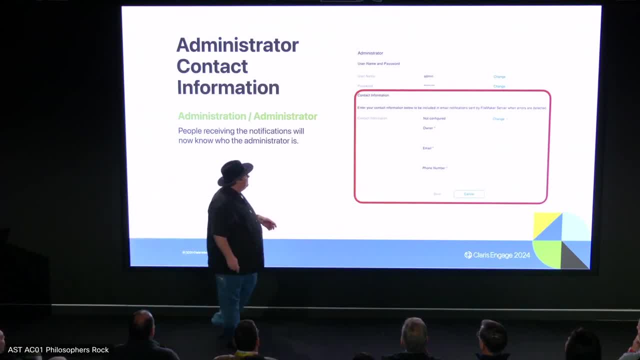 and I don't know who actually I need to call and yell at saying that it's down and not running. So now, when notifications go out, you can set who the owner is and who. you know who who needs to be there. 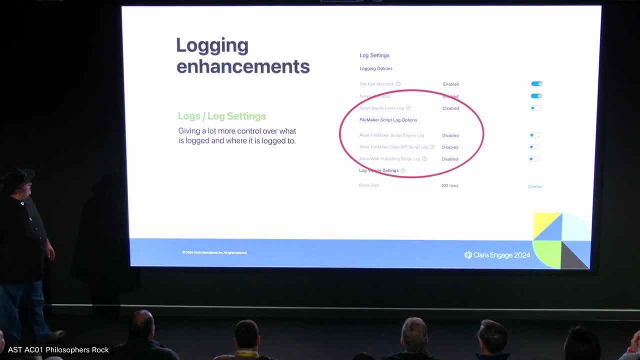 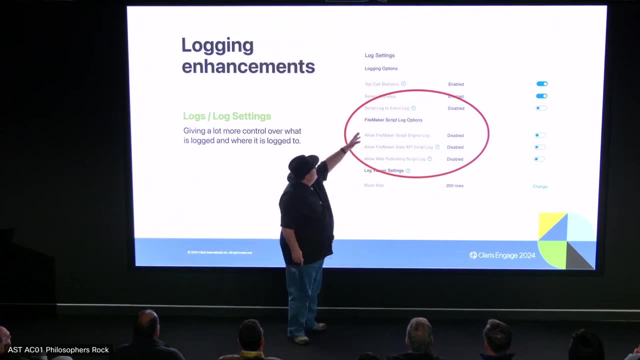 Yeah, Logging enhancements. Lucy was mentioning how you know, scripting is split out. If you really want the scripting log to go into the main event log, you can still turn that on. And this is where you turn on the logging for the SASE. 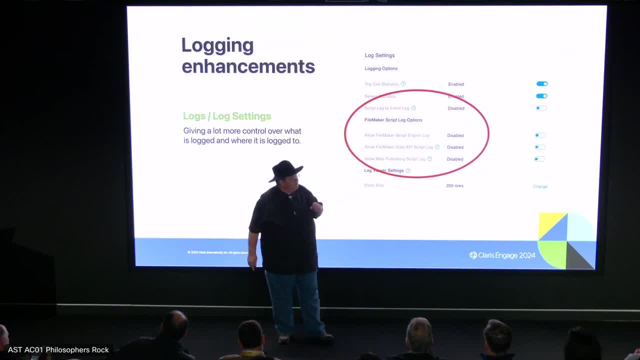 for the data API and in the web publishing script logs. Those three files you can either turn on or off. You have to turn them on here for the script. step inside FileMaker to start logging and stop logging to work. If you don't have these on and you have that script, step in your script. 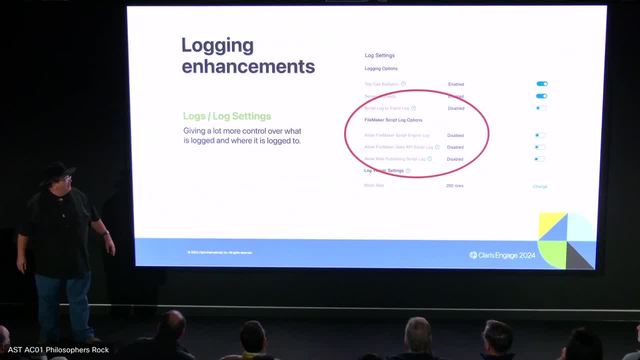 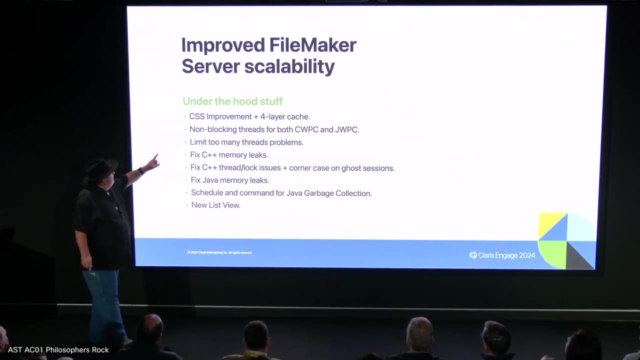 and it runs on. you know one of these other platforms, the web publishing, or you know web director, the SASE. it won't force it to turn on, It won't turn this option on. So other FileMaker improvements: 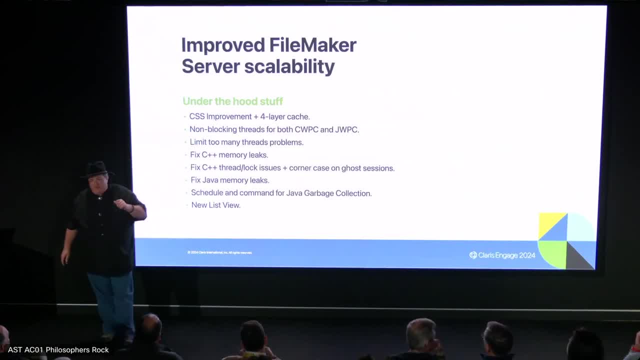 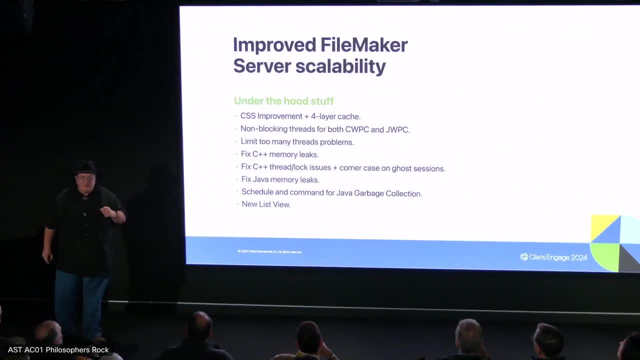 We're improving the caching. Caching is hard Um, uh and a lot of the improvements inside web direct to be able to support more users into uh in. the one process is to do to do a smarter level We have with this four layer cache. 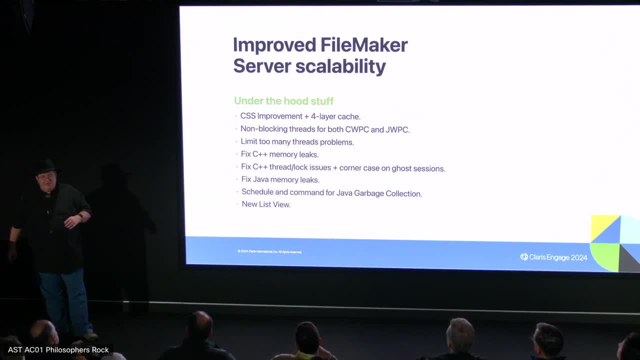 Um, there's this whole big blog internally that I read some of it up and saying, well, okay, it's, but basically, basically, um, at different layers you can cache more things and not cache things. Uh, some layers of the cache you can share between multiple clients because they don't change base. 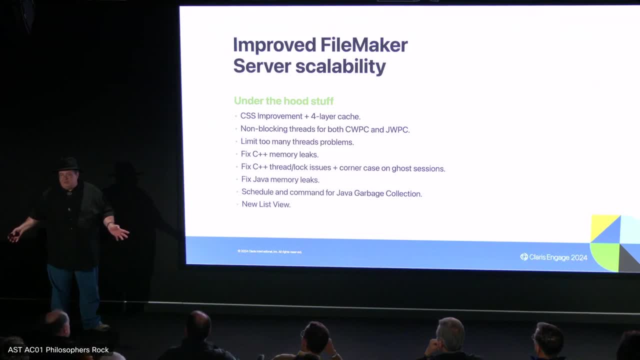 You know why, If you have a hundred and fifty clients talking to this web process, before we were creating a hundred and fifty different caches of this object, but now we're smarter, We're only. you will only have a cached once, because it rarely changes and it's less memory to use, less stuff to allocate. 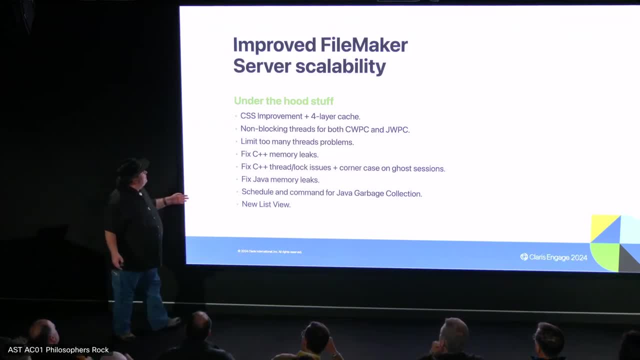 deallocate and handle things to easier, non blocking threads. We're going through watching using these advanced debugging tools and Lucy was mentioning before Some of them. tells you where your hotspots are, What you know, what mutex is People are. all these processes are hanging on. 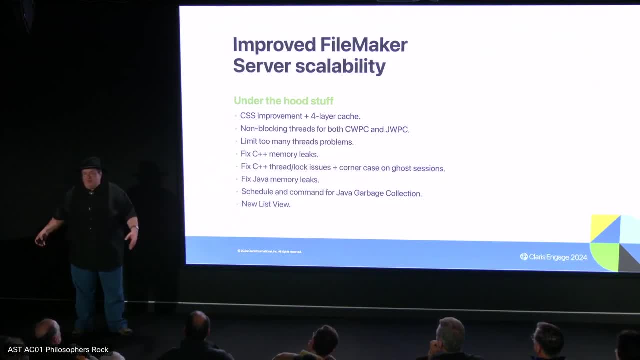 So we look at the hotspots and saying, oh, why do you know why are all hundred and forty nine other users waiting for this mutex? You know why, why? why do all these clients actually have to wait for this one resource? 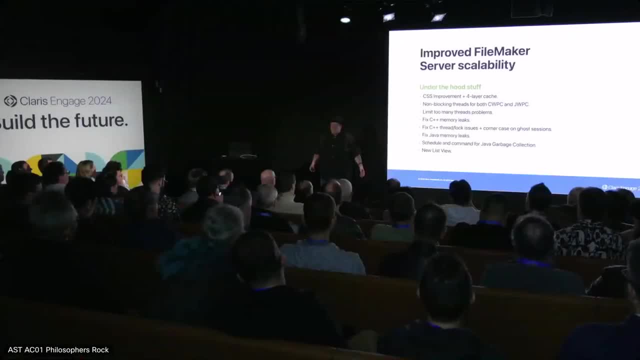 And sometimes it's just um. you know, someone was a little bit paranoid and decided: well, let's make sure it's safe, So we'll throw in a mutex. So you know, that's one reason when you don't understand what's going on. 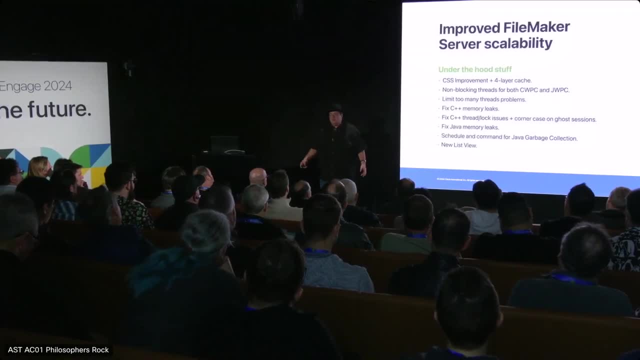 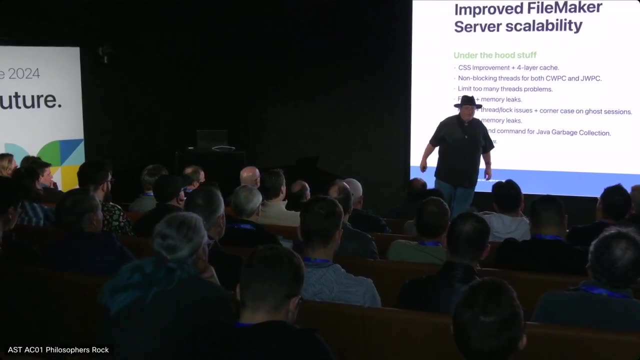 not just throwing a mutex, and you know, your guarantee that will work won't necessarily be the fastest, though, And then you kind of have an opposite. problem is that some developers are saying, well, let's just throw it on another thread because 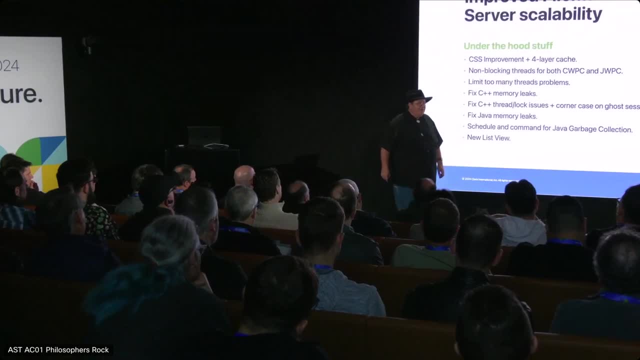 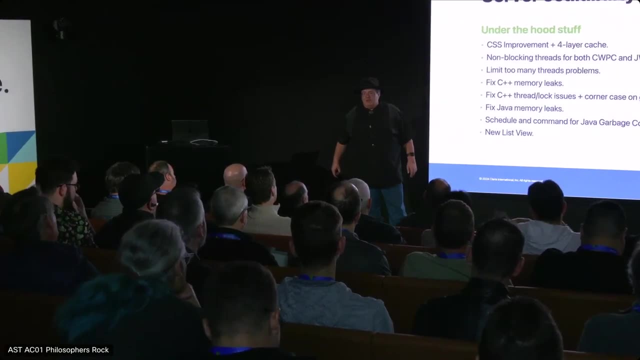 yeah, you know. but you know ten threads are nice, but you know one thousand five hundred is not good, It just basically kills. you know your processor If you're trying to run that many things at the same time. 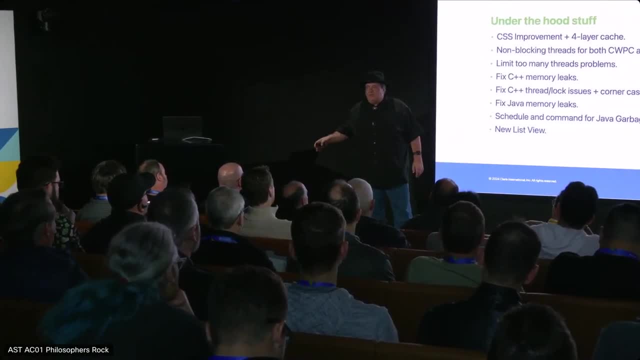 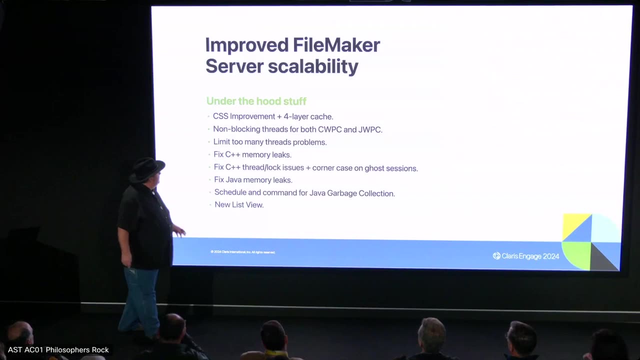 sometimes there's a lot faster. just to you know, don't don't even spin up the thread, Just wait for the process for some threads to come back. This is thread pooling, That's. it's a very standard pattern with using these tools. 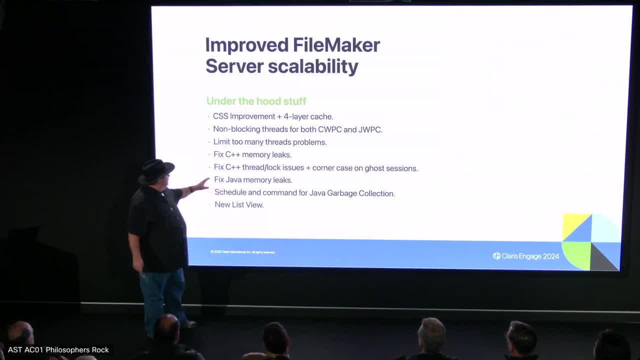 We've been finding in C++ memory leaks, Um thread locking issues. So this is a sand that's been finding these things, This is tea sand that's been doing this. He sends pretty nice and that it'll tell you when two different threads are accessing the same memory. 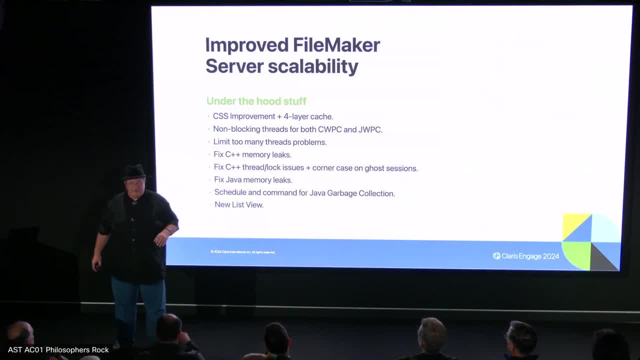 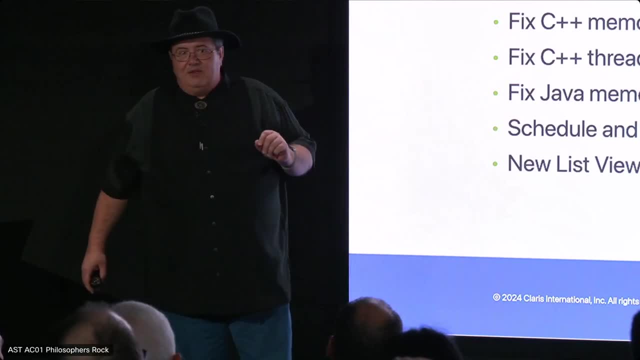 and there wasn't any type of synchronization event between those accesses. Now, when you run these tools, it really slows down server So well. sometimes we'll give a customer a specific ASAN version if there's something that we can't reproduce internally. 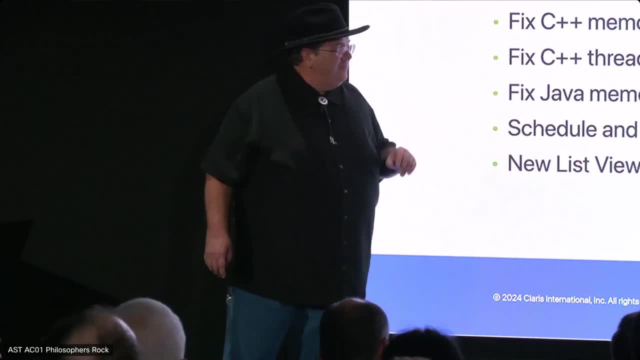 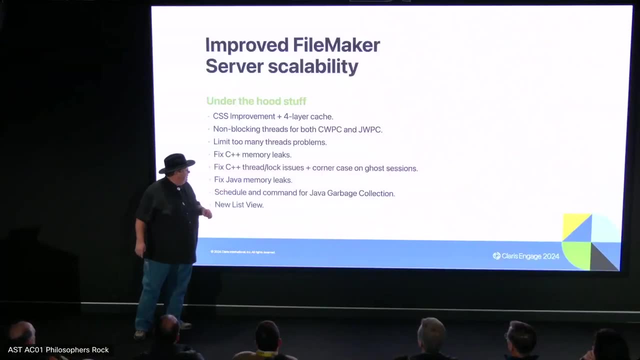 But these bills with these tools turned on are really very specific and only useful in certain situations. But we've been fixing the memory Java leaks that were occurring. So, in addition, actually I really hate garbage collection operating systems. I really want more control. 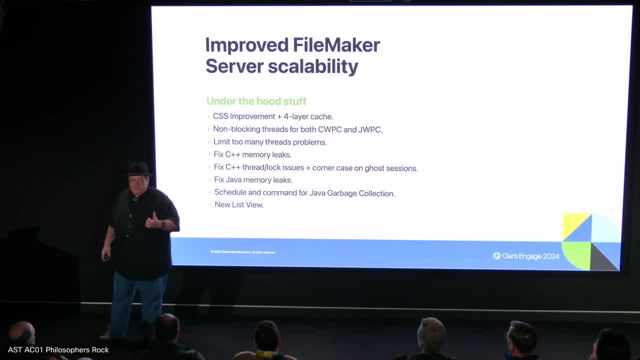 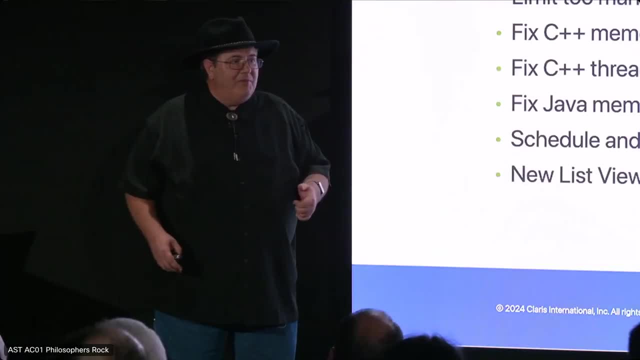 And you can even see that with Apple with a objective- See the first version- you had to do memory management yourself. You have to grab and release the second version. They say, oh, we want to make it easier, So don't worry about it. 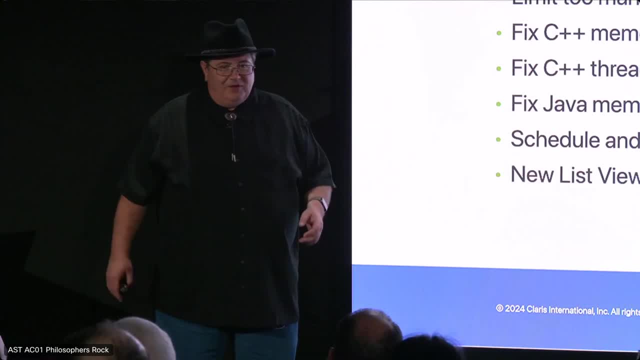 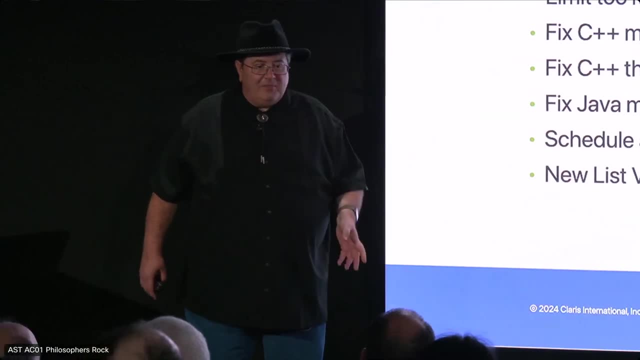 We'll do garbage collection. You know we'll clean up memory when it's no longer use. That didn't work very out. work out very well. So they went through and then they did something, which is actually pretty smart. Is that during compilation time? 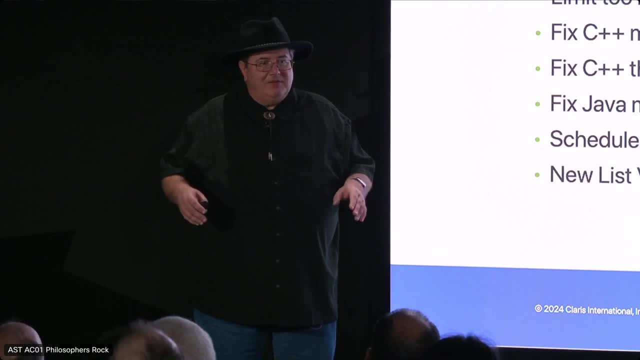 it knows the code flow and how things are working and it basically does what the first process was. It does the grabs and releases, but you don't have to figure out, figure that out. It knows how the code can flow through your system and as those things magically behind the scenes. 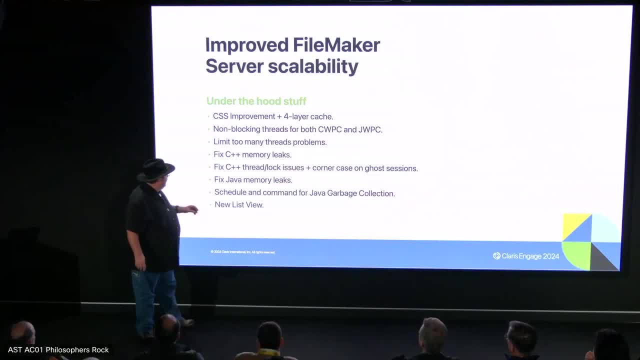 So I wish Java would do something like that, but maybe fixing Memory leaks, and we've given you these abilities to force the garbage collector to run more often. I mean, Java is supposed to run that stuff when it needs to, but I've never been happy with it. 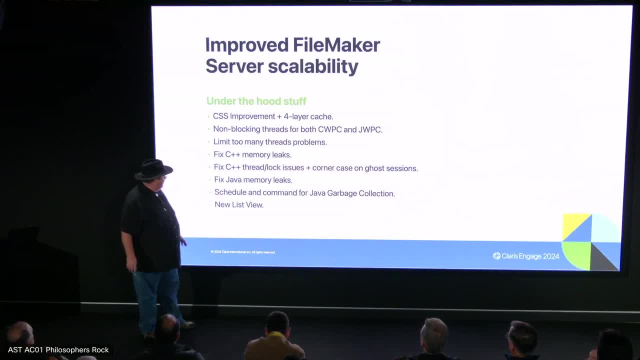 So the workaround is to schedule that Also. the other thing- you'll see the other thing in web direct- that we did that to improve things- is that the list view is now almost a complete new implementation of it. It doesn't flash all the time. 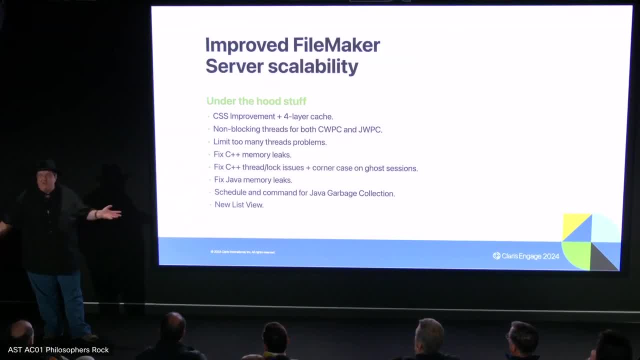 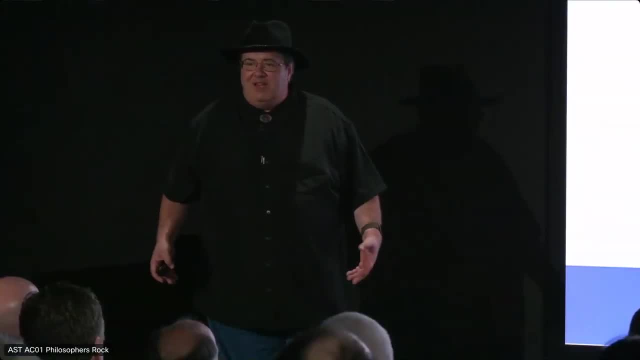 Every time a new record comes in, it is actually usable now? Well, it's usable If you were the only person on the system, but so it looked good for a demo, but the minute you have, like you know, other people doing work at the same time, 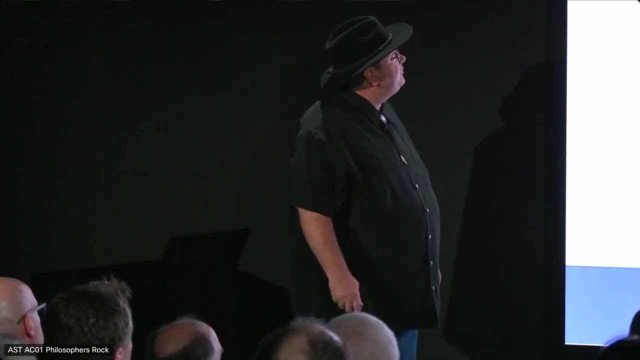 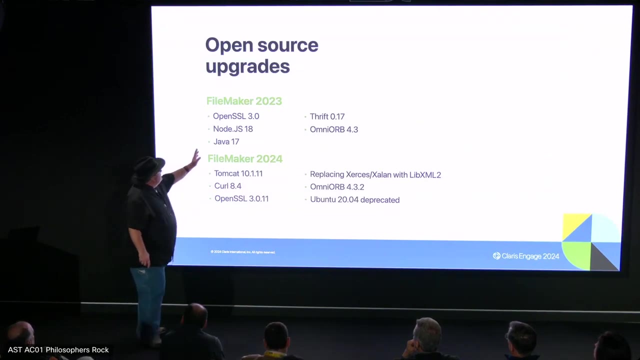 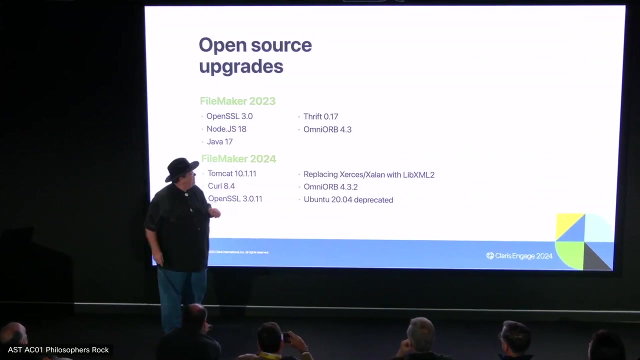 it. yeah, it failed pretty quickly. And lastly here, open source upgrades. She mentioned these things that we've been upgrading. The Java version is kind of pretty much tied to the VADN version we're using, So we want to make sure that they're compatible with which versions I'm your. 4.3 is. 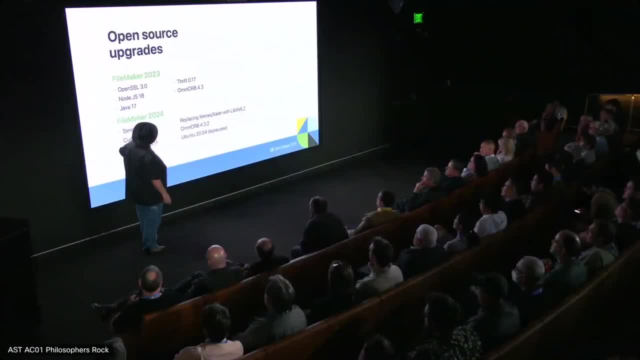 uh, gave us the ability to use web sockets. We're doing the communications Interesting thing. Open SSL 3,, you know, killed a bunch of cryptography, things like MD 5, and we use MD 5 hashes internally inside FileMaker. So we actually had to write our own implementation of MD 5.. 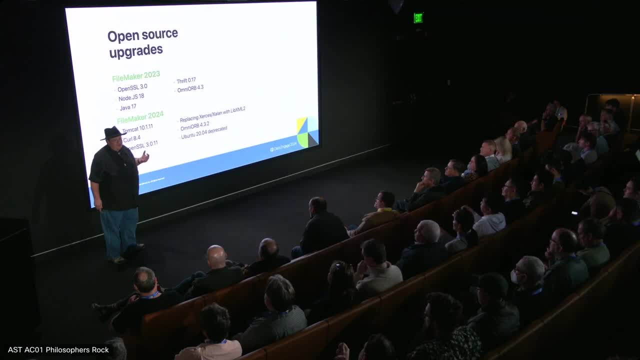 This is not a security issue because you can't ever get access to that hash. You know you can't twiggle, twiddle some bits and communications going back and forth to you know fake out something. So it's safe as long as you don't give access to the MD 5s. 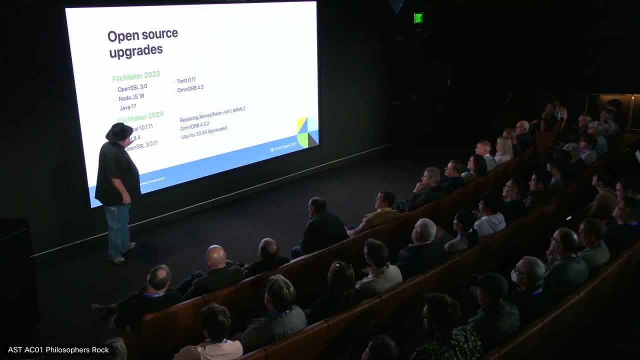 It's actually faster than some of these other ones too, but if I'm like a 24 and 24 will be updating Tom hat curl latest version of that. There's always a newer version of open SSL. I think 12 is coming out soon too. now. 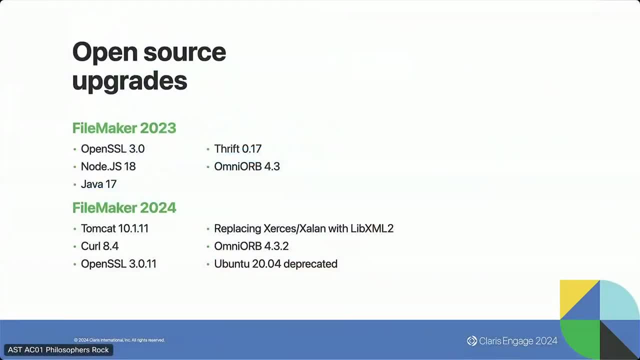 so it may be that a big thing here Replacing Xerces and Zalon with live XML, They're seeing Zalon has not been supported and has not had an update like in 10 years, I think, And we've been getting bugs of how I can't handle modern Unicode characters and a bunch of different issues there. 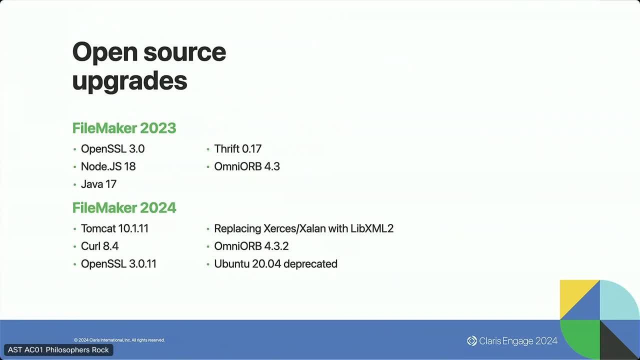 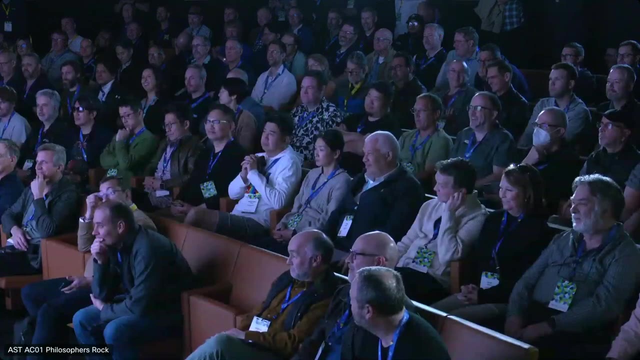 And so we're now moving to a XML library that's supported open source. Apple uses it internally or Apple installs actually on the OS, And this gives Beverly Voth another chance to write a new book, The other thing of Bantu 2004.. 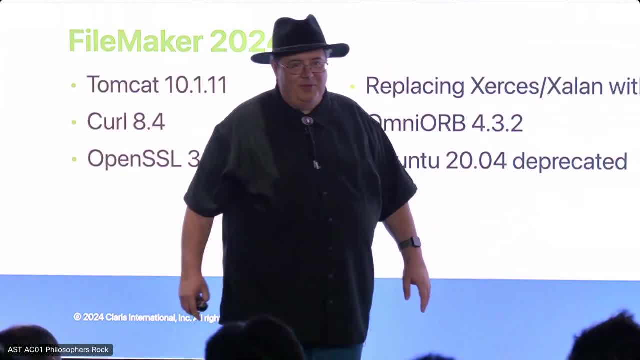 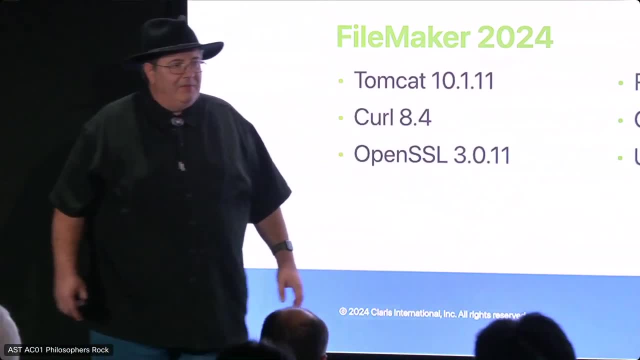 I know where we announced this, but I'm telling you it's coming up. We were going to be dropping support for that. We can't support three versions of a Bantu because you know Bantu 24 is coming out and I'll be the new version. 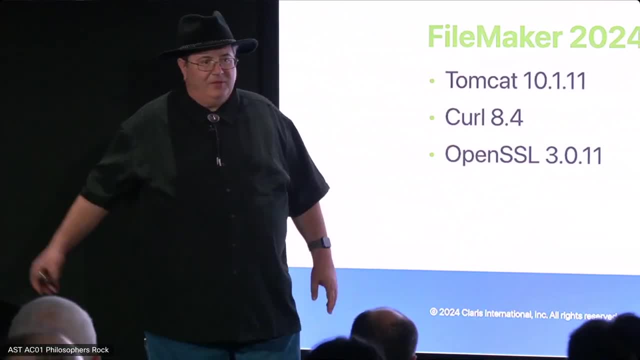 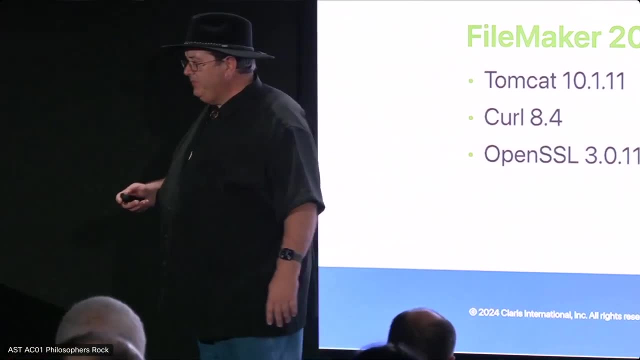 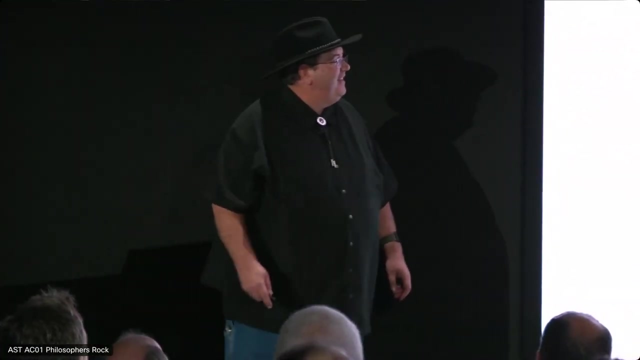 So it will be moving to supporting 22 and 24.. And I think the LTE stuff is dropping off soon on 20.. So this is the best time to be a file maker, developer. So what is next, The next steps for us? 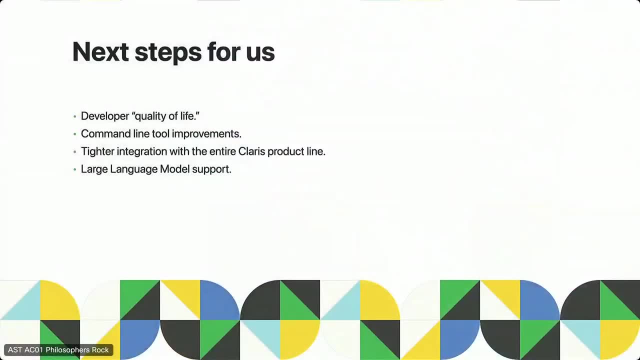 we have a team working on quality of life, things like doing. you know, you have the search light in the macro. you just type in something and they'll find something and open it. So we'll have a window. I think we're going to use command K. 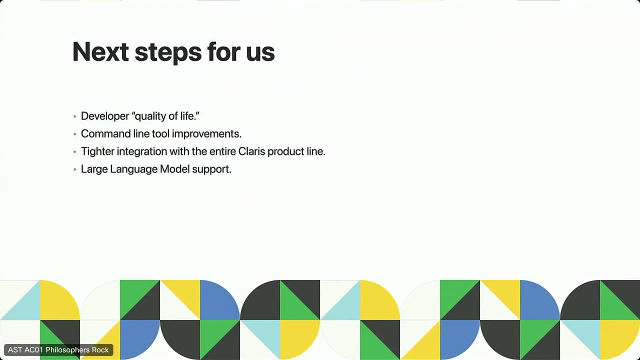 You hit that. you can type in a layout name, a file name, a script name, any type of name, and then it'll pop up a list. You pick one. it'll jump right there for that, Giving you more options for. 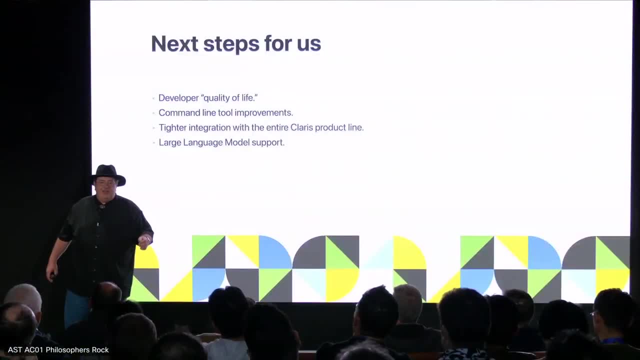 when you're in layout mode or scripting, like when you add a go to next record script step, maybe you want that checkbox saying, oh, exit in loop if not found on by default. So some of these things are tiny things, but when you add a whole bunch of them together, 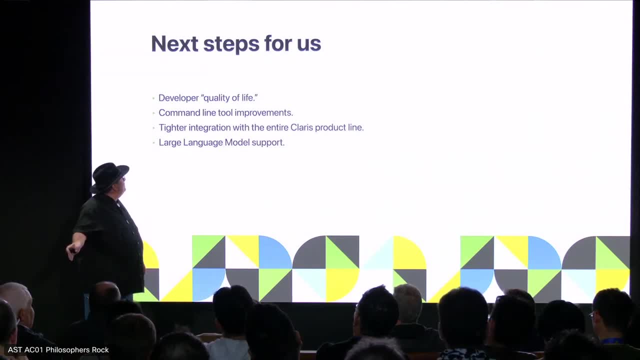 we call this the quality of life features. So we have a team working on that. We're going to be doing tighter integration with the entire Claris product line. There's a lot more work on connect to do Claris Studio. we're kind of waiting on them to supply us APIs. 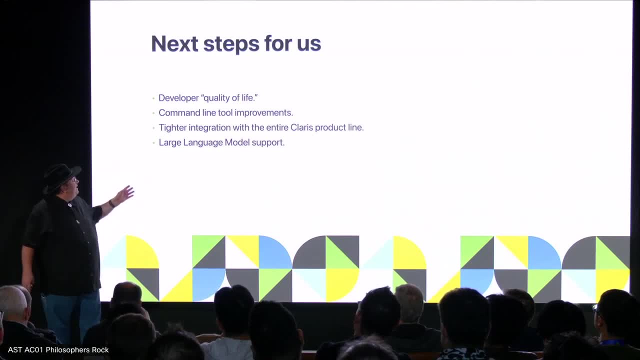 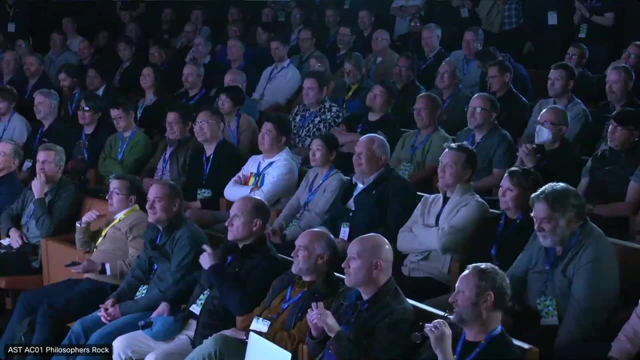 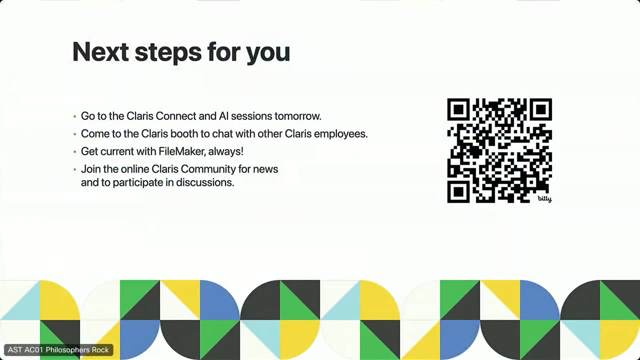 The minute we get them, we'll implement them, And everyone else has been talking about large language models, so I won't. The next steps for you, though: go to the Claris Connect and AI sessions tomorrow, so you can learn about LLM and what's going on there, and learn more about Connect. 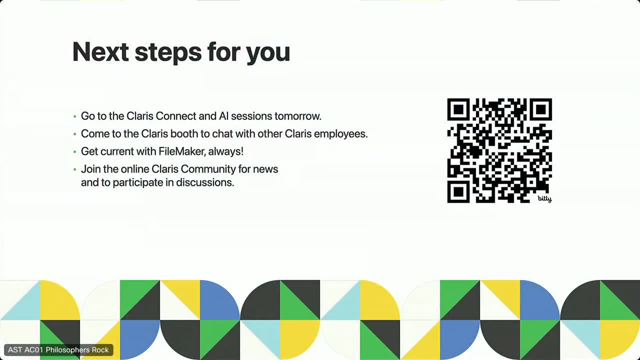 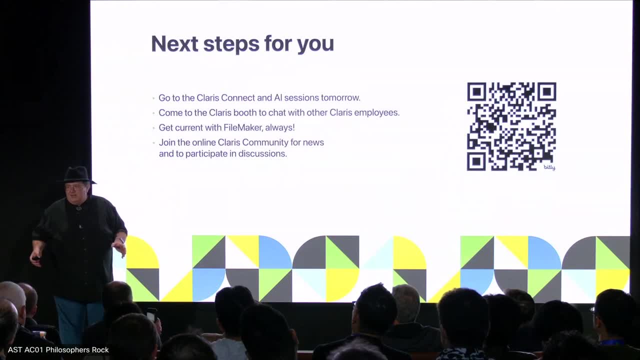 Connect is. we should have done this a little bit earlier, but I think this is going to be very, very strong future for gluing things together, gluing studio I mean. I think they even announced it that you know a studio and connector can basically get merged. 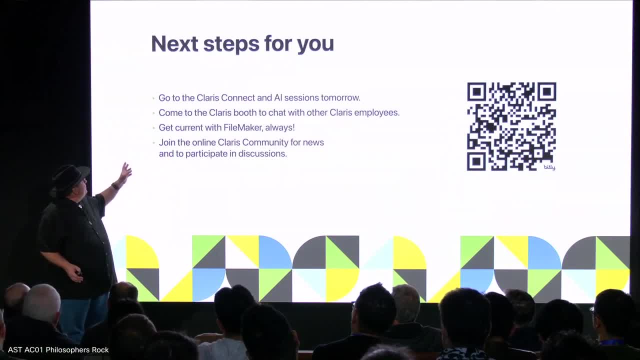 and it's going to have a lot tighter integration with FileMaker in the future too. Come to the Claris booth to chat with Connor. I guess Wade is there right now, so you'll miss him today, but I may drop by there when I have a chance. 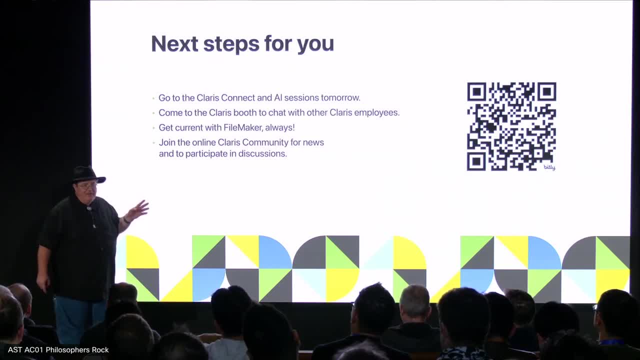 Get current with FileMaker and always do it. I mean, if you don't upgrade to FileMaker, then why am I here? You know, and join the online Claris community for news and to participation discussions, and that's what that QR code will take you to. 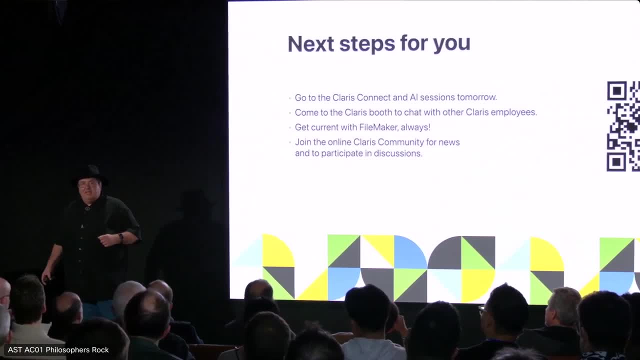 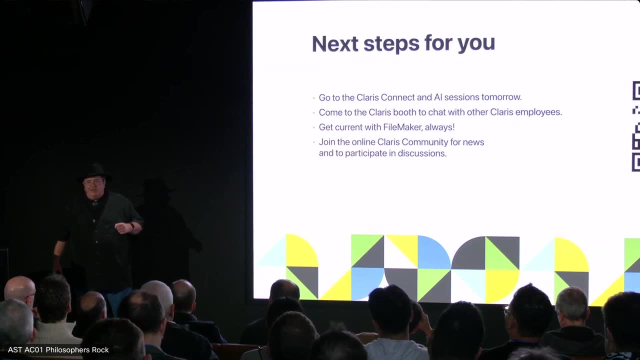 Also, I guess we're inviting more people to join the ETS program and if you want to do that, send an email to ETS at Claris dot com, If you really want to get in and live on the bleeding edge and maybe destroy a bunch of FileMaker files that we told you that you shouldn't open. 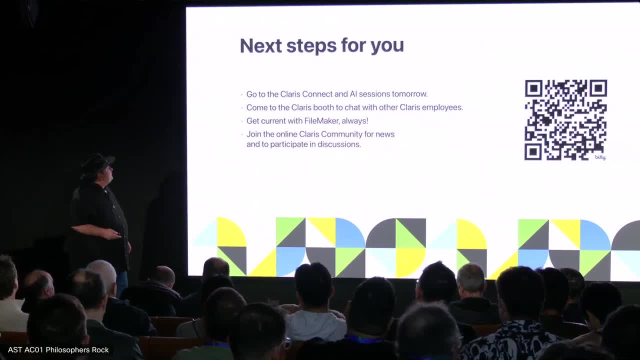 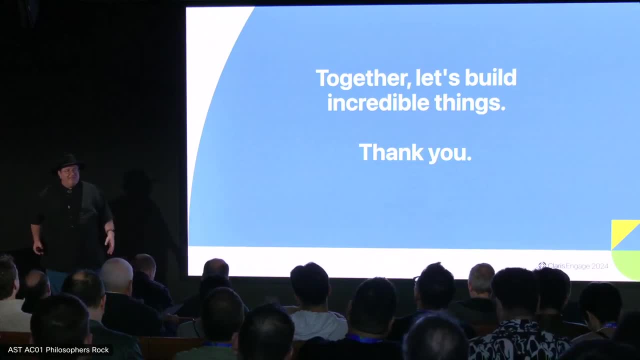 unless you really have a backup. So that's yeah. so you know, with the power of your organic brains and our technology that we're giving you guys, we can build a. we can do incredible things. So thank you. 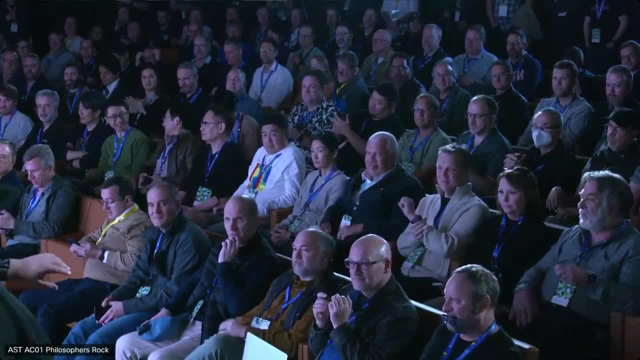 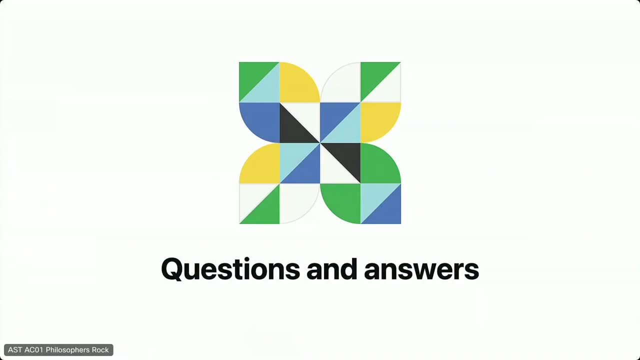 Now the first question is: is there chocolate? And yes, there is going to be chocolate at 4: 30. So just go upstairs Real quick. So start of restoration is a nasty history. So now we have the persistent cache. 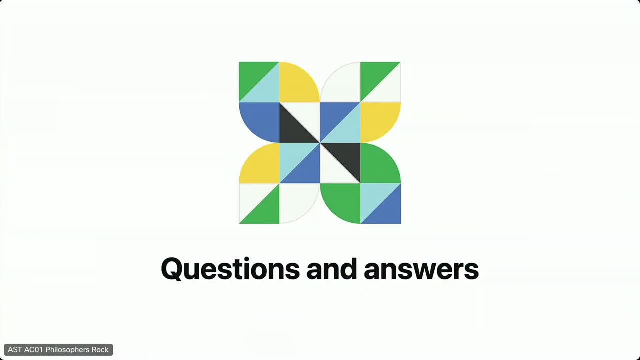 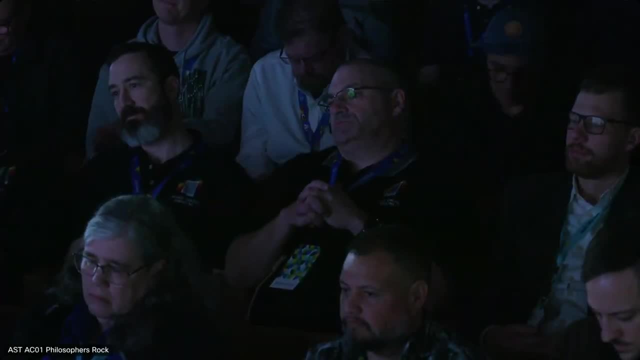 What is your confidence in persistent cache? Can we really trust it? Yeah, I mean, it's been out there for a year already, in 2023.. There's been a few minor bug fixes that were more like edge conditions that we've updated. 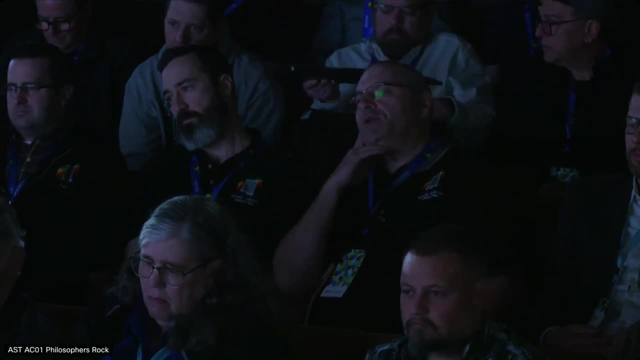 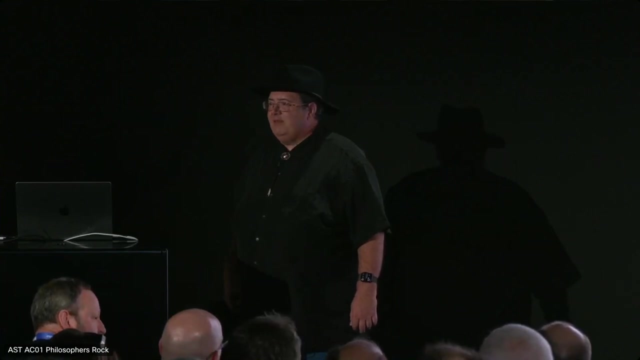 So yeah, yeah, no, we're messing with the structure and we don't want our customers yelling at us. So, yeah, it's not nearly as invasive as the previous restore is. Yeah, start of restoration was a little bit more invasive inside the Draco engine. 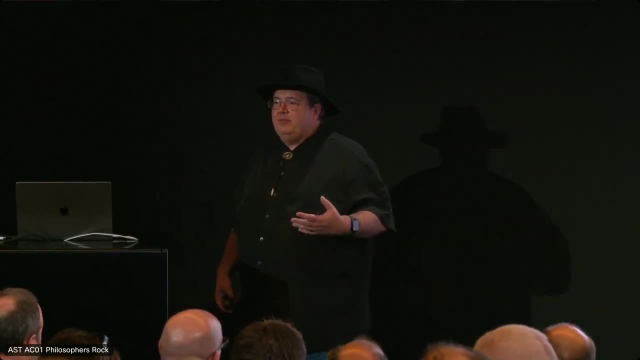 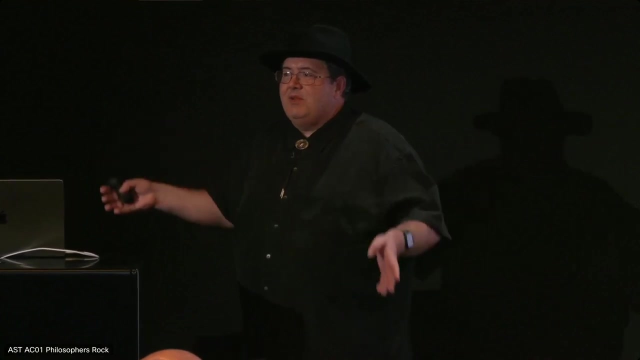 This thing is basically just turning on an operating system feature saying that, oh, we put this cache in this memory, write this memory to disk when you have a chance and then, if there's a failure, then that's when we look. So. 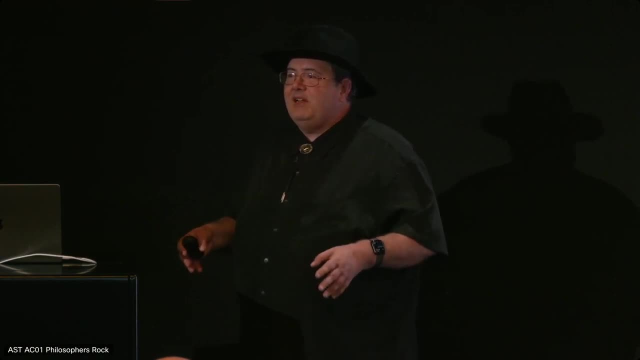 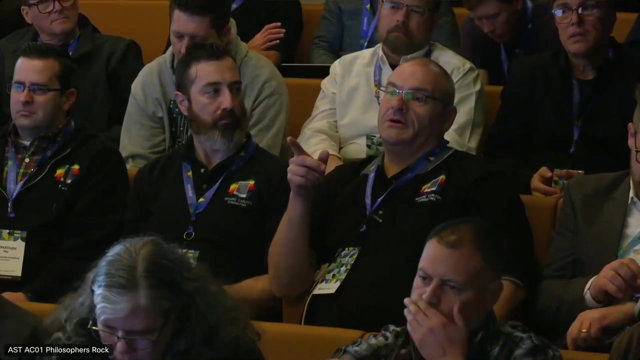 when there's a failure is when all the real work does. So if there is a failure, it will be a failure in bringing it back up, but it shouldn't affect, you know, operations Not on a power plug pull or. 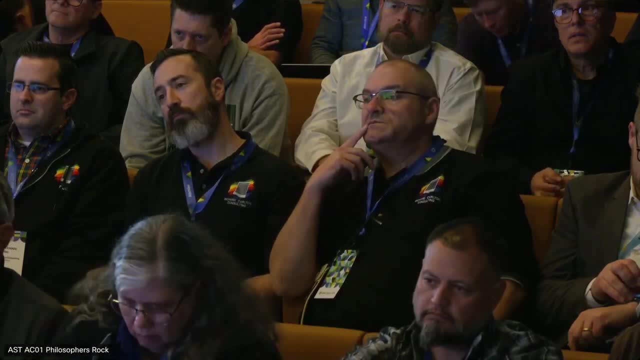 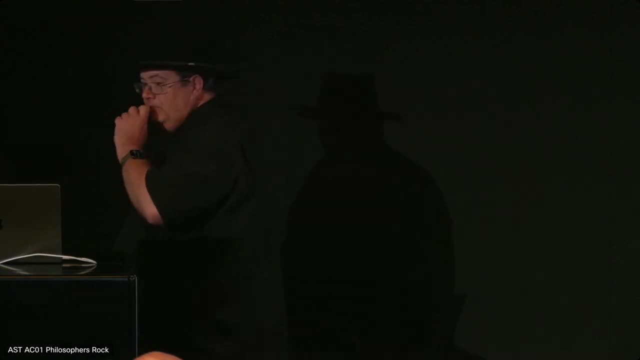 Not on a power plug. yeah, you can't. you can't save a hard drive, just stopping. Actually, I want to add to that There were two settings that you all saw: persistent cache and then sync to disk. The sync to disk setting is for pulling the plug. 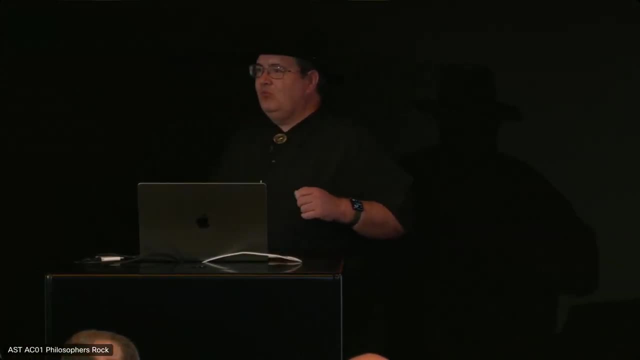 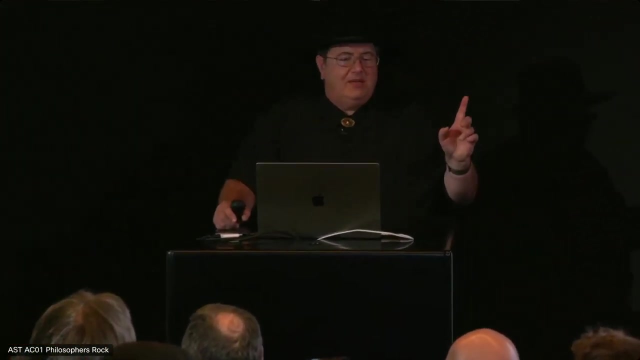 So I've pulled the plug. so Really Mm-hmm. And it didn't corrupt files, so yeah, Okay, Let me mention something for the people in in Zickler Park is that they're going to be shutting down that room in five minutes. 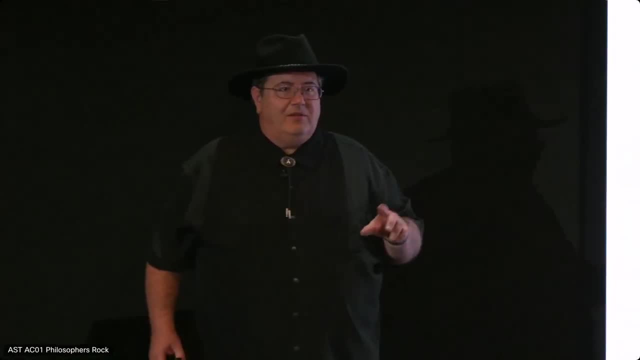 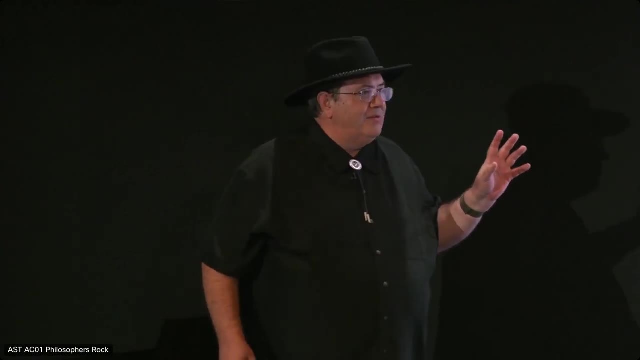 So if you have a question, you may want to come over here. They, the partners, are going to have an event in that room, so they're going to be kicking you out soon. So sorry about that, but But we'll continue. Q and A here. 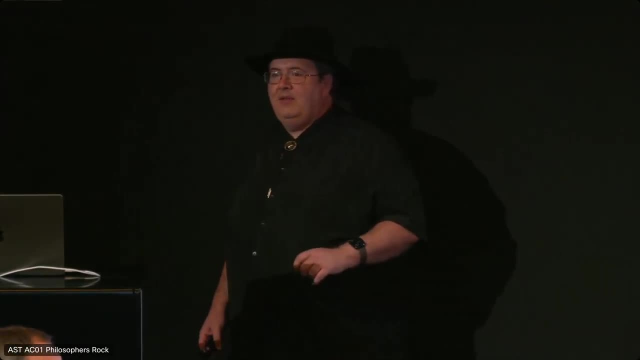 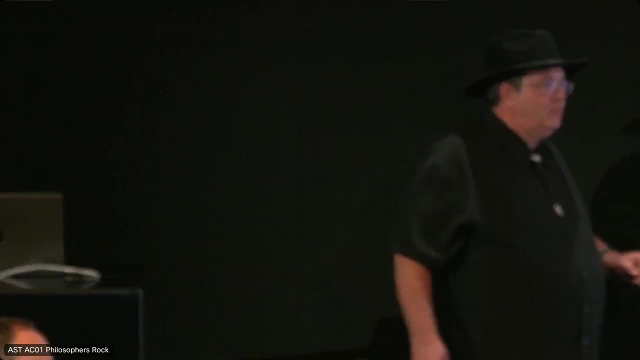 Yeah, we'll continue Q and A here, so So a quick ask: having seen bottom right saying, hey, we're going to drop support for 20.04 Ubuntu, Mm-hmm, A lot of us moved into Ubuntu world to kind of. 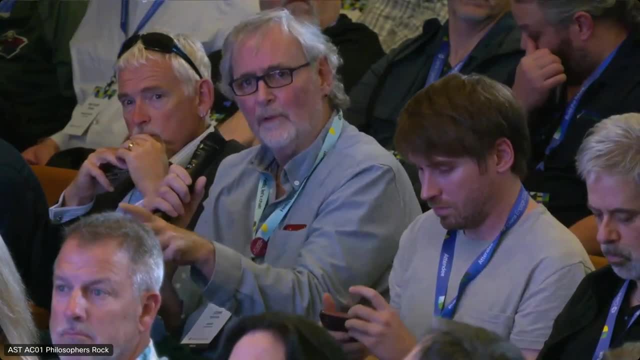 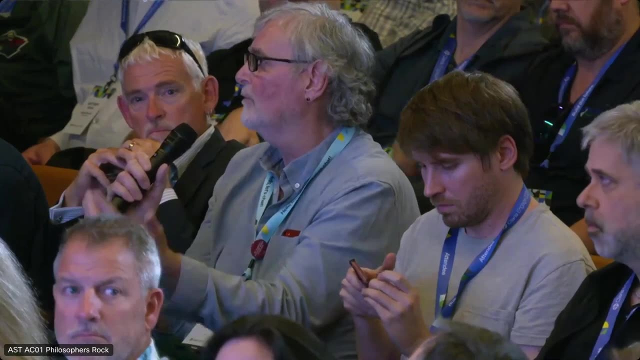 to make it work and it's brilliant, but we're not Ubuntu experts, so we've got to go from 20 to 22.. Can you write some documentation to help people through the process of doing that, Because there are multiple use cases for that? 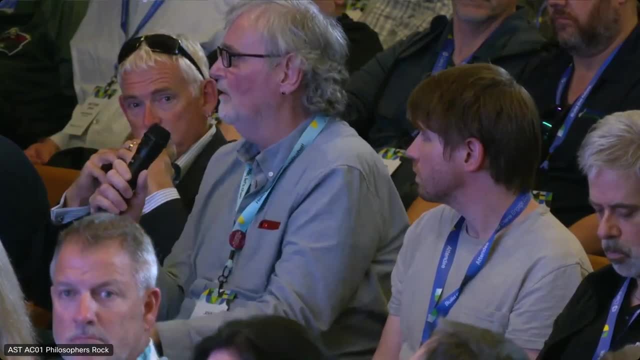 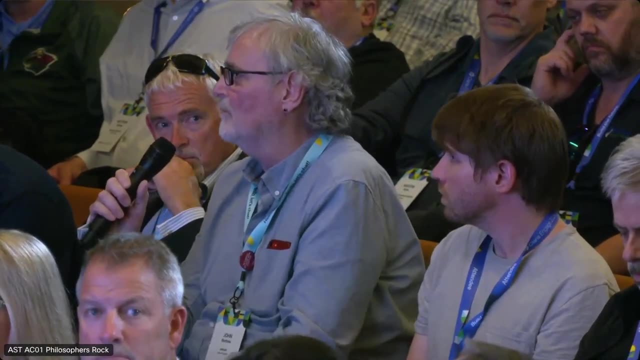 We're on high rented in VPSs You can't just do an update, because you lose all your files, but also the in-process update may throw up some errors. So could you give us some help with some additional documentation? We'll note that. 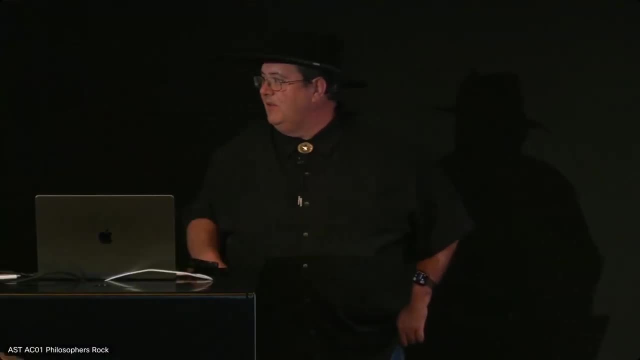 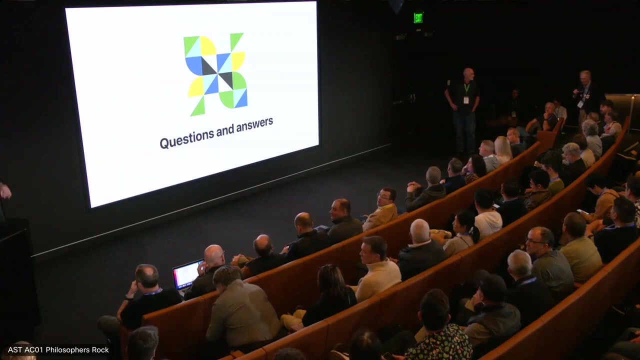 We'll note that. yeah, We'll take it back. All right, Yes, sir, Let's go over here and then, Oh, you have the mic. Oh, Okay, You, you all knew, Oh Know, that I was going to do it. 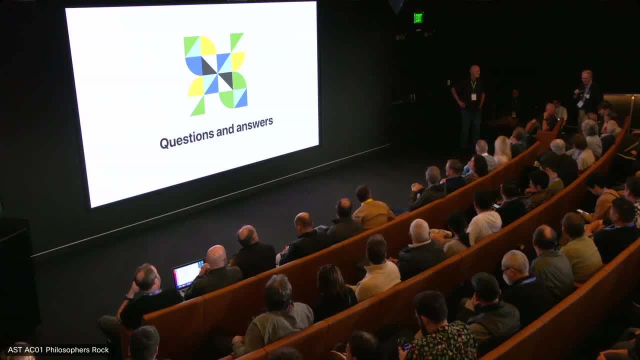 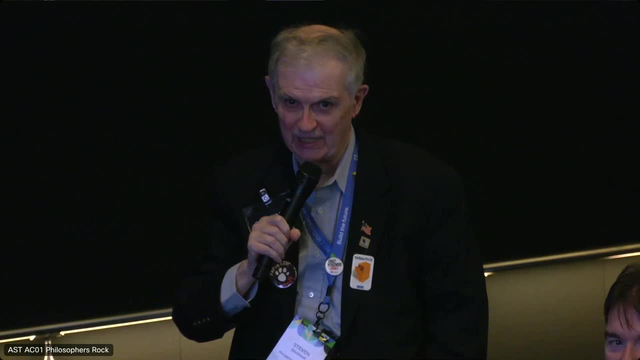 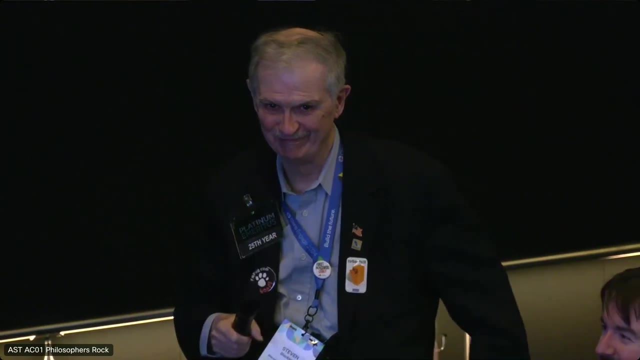 Okay, In your, in your future plans, let's take a look at passwordless, at bound and unbound keys, and let passwords die a decent death. No, Yeah, No, it's, And I'll see you at RSA. 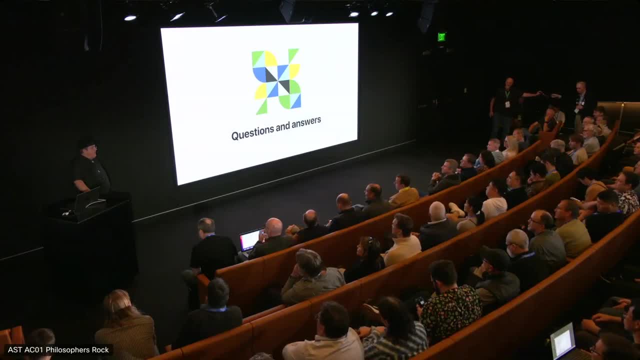 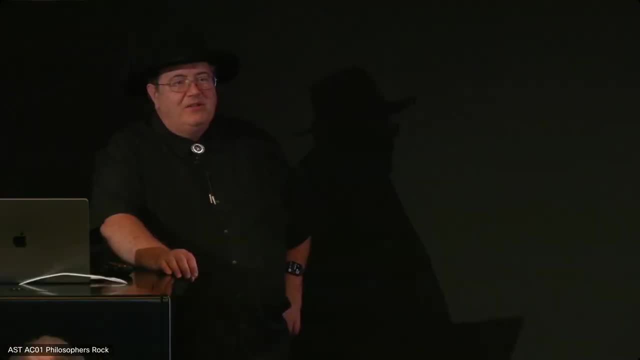 Right, yeah, yeah, Well, Apple is really. so Apple, I guess, has noticed us So, which is sometimes a good thing and sometimes a bad thing. So their, their security department has been. you know, they have active white hat hackers, you know. 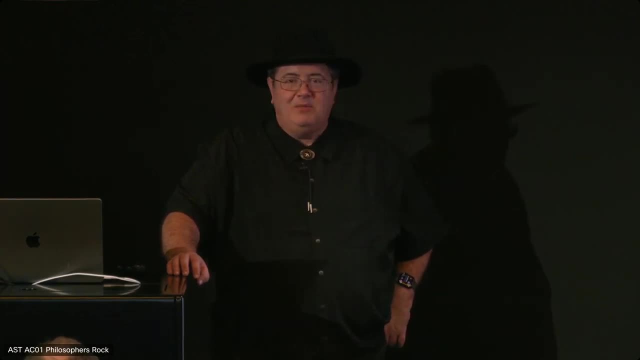 trying to break into FileMaker. They're trying to find holes and stuff like that, And they did find a small hole that were there's going to be new versions of 19.6 and 20.3, I think, Yeah, coming out of of server to to handle these things. 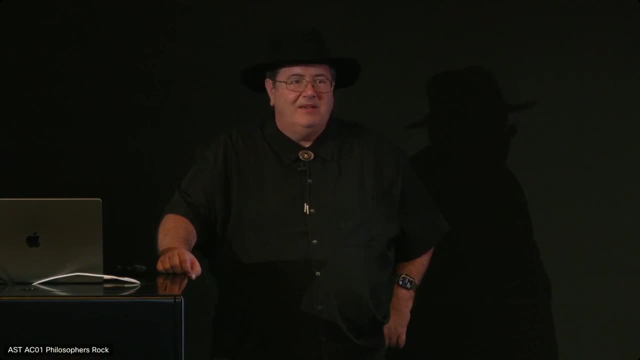 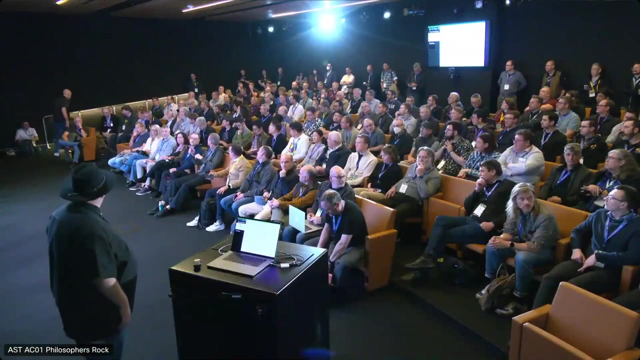 It. it's kind of complex to how to you know, to get that to happen, But any hole is a hole, So we're we'll. there'll be new releases coming out to to fix that. Send the white hats to me. 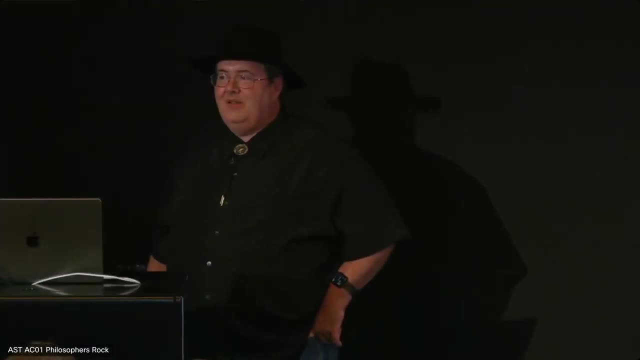 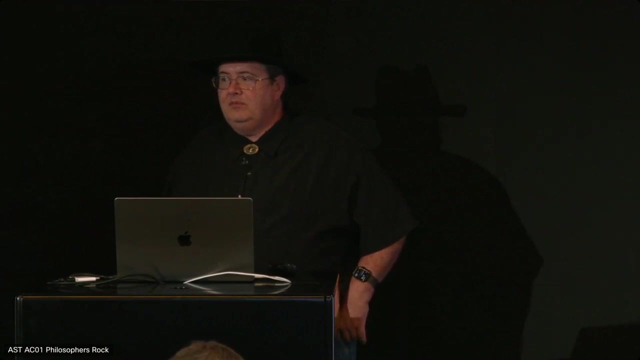 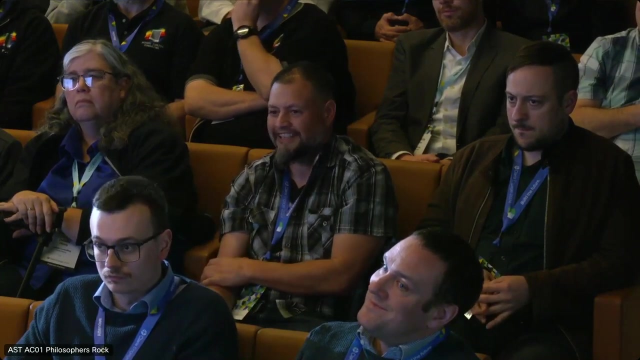 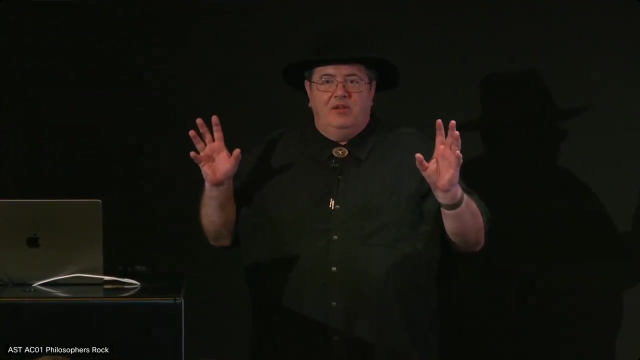 Oh, send the white hats to you. Okay, Rick, we have a question here With Claris Studio mentioning MongoDB background. is there any plan to have FileMaker be able to use MongoDB As the, the SQL engine? No, You know one thing: 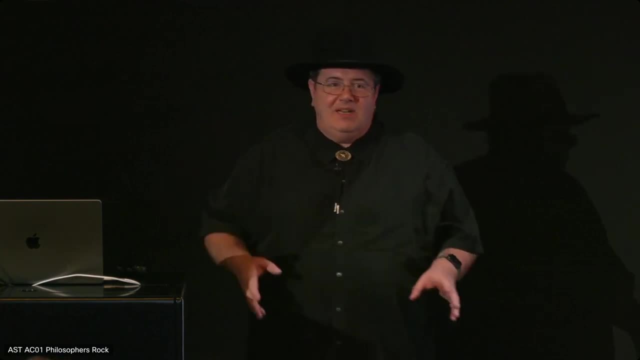 FileMaker, you know, is the pessimistic locking. There's so many rules that that FileMaker does. That really makes it, you know well, it makes it FileMaker and everything that you know. But it does not make it an easy thing to expand, to handle. 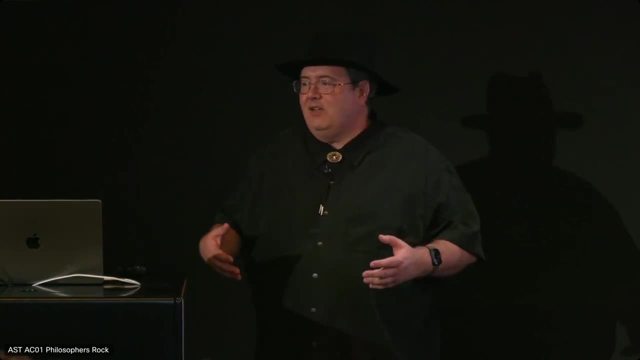 you know thousands of customers and stuff. So you really can't do pessimistic locking. You have to do optimistic locking. You have to have a a different model in the backend. And there's no way and and you can't- and I was talking- 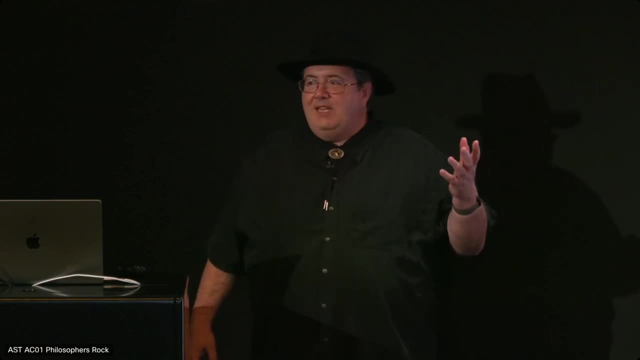 about context for how the you know scripting system works. You really can't have server backends remembering the context of you know 20,000 customers trying to hit your server and stuff like that. So the whole FileMaker model really is not scalable to. 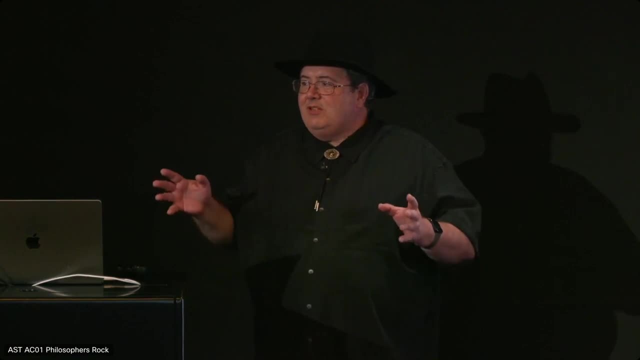 those numbers. So we see just a much tighter integration of being able to move data back and forth between the two being able to access data from there. Studio wants to be able to access data from FileMaker directly too. There, you'll have to talk to them when. 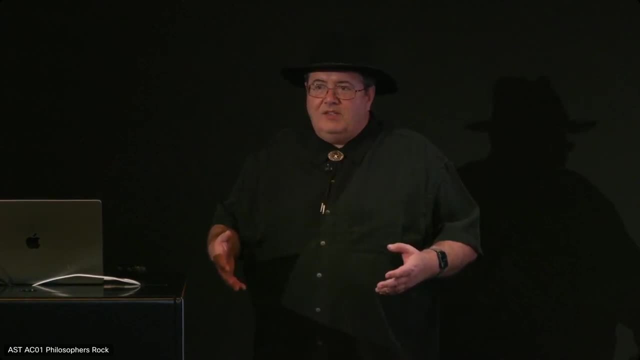 what their plans for that is. So I really see it as two separate stacks. It also another divider between it is that something inside FileMaker that was always fighting us is that, oh, we have to be the database for new users that know nothing. 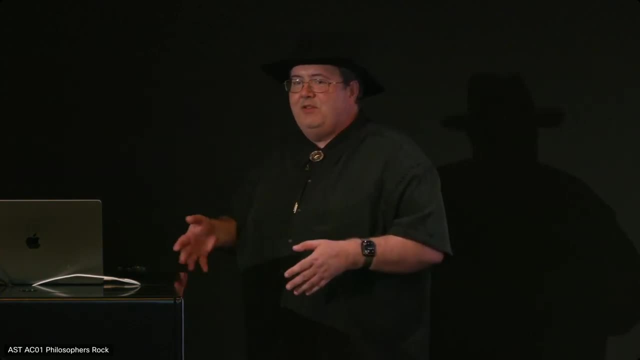 about databases and stuff like that And be the database for you developers out there. So there was always a fight going back and forth And you'd complain when we make things to make it easier. We don't want to go through all these wizards and panels and 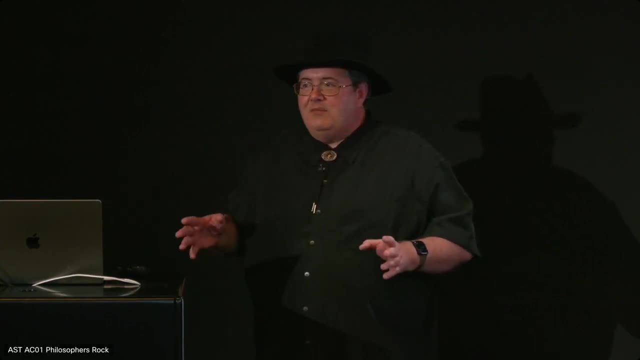 stuff like that. So I see the FileMaker direction sticking with the developer customers and Studio being the new user customers, The people. that's the first try. We get them hooked on that first and then say, well, we need to go further. 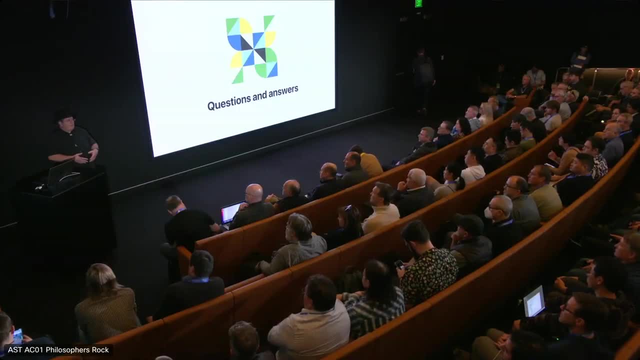 Here we can look at FileMaker. If you don't know how to use FileMaker, there's a whole community of developers out here that we can send you to. So that's kind of the basic strategy of how we want to go in the future. 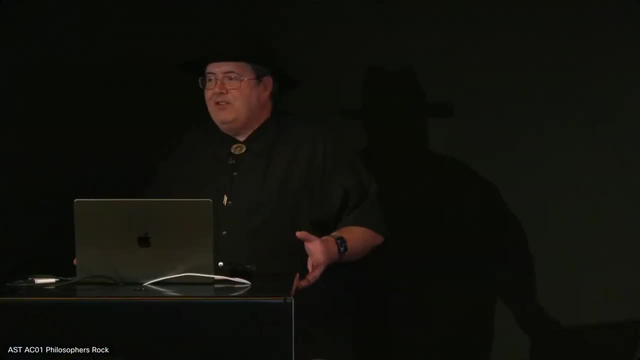 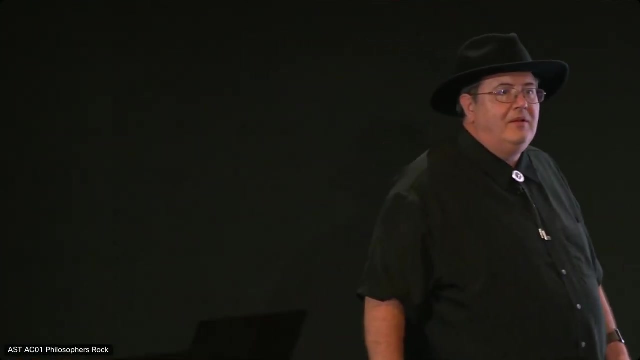 So that's, and yeah, just the Draco engine knows how to handle FileMaker style stuff. And then Mongo is the back end for the masses. You talked about developer quality of life, with some cool new features coming. What about a co-pilot? 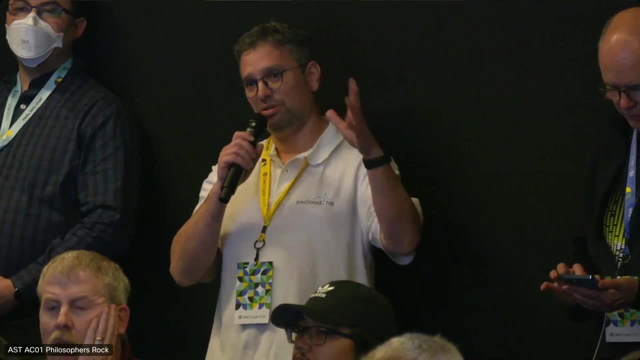 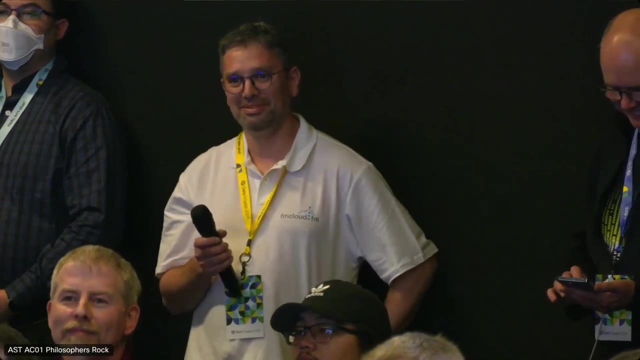 What a compiler. Yeah, like GitHub co-pilot, you know, code generation Co-pilot, Oh, co-pilot. Now that's all in the AI discussion stuff. I've been trying to ignore all the AI stuff myself. 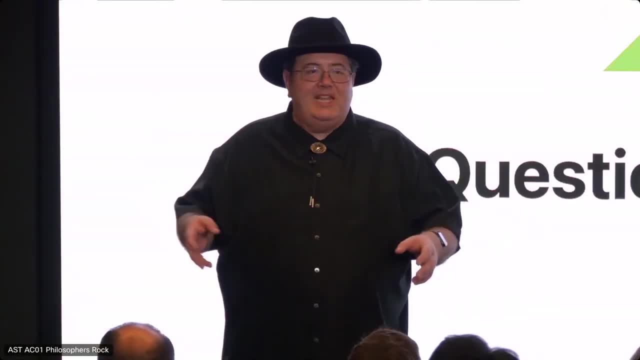 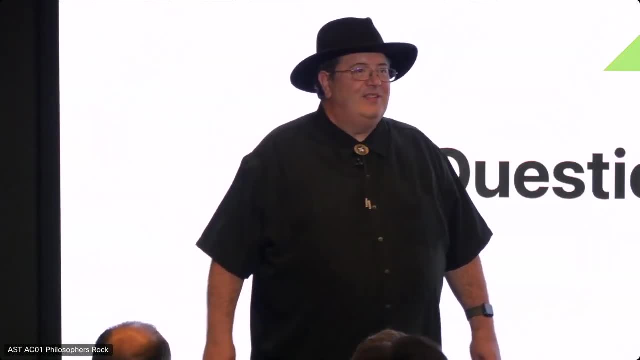 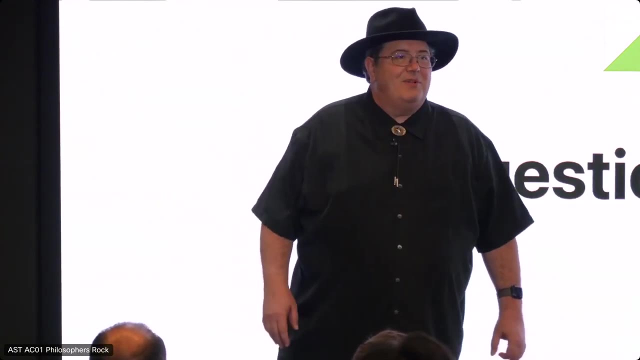 So I haven't been. I see these people saying things and typing stuff in and all of a sudden like a calculation pops out and say that's amazing. I don't want to think about that, so sorry, Ask Ronnie or ask Wade about those type questions. 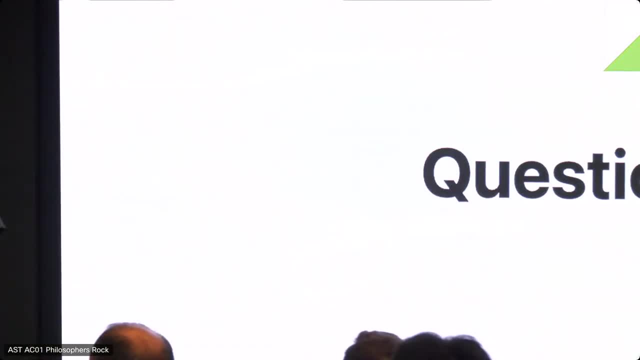 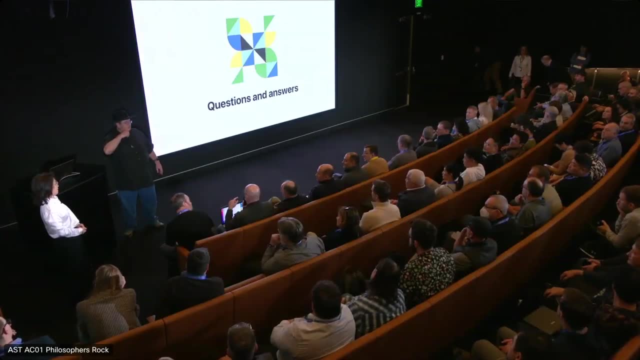 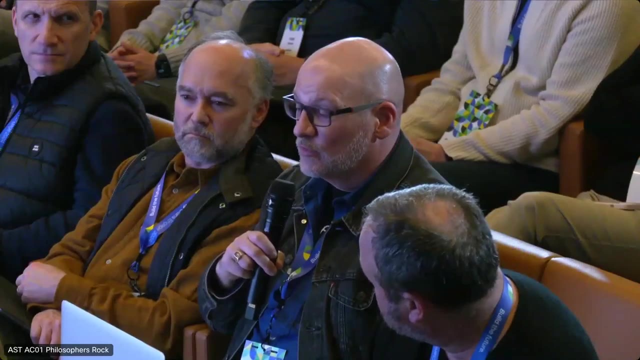 You mentioned- Let me get this one over here. Yeah, You mentioned in your in your presentation, assisted install files right here. I was having a conversation this morning with another developer about that. Would it be possible in some future version to have the set? 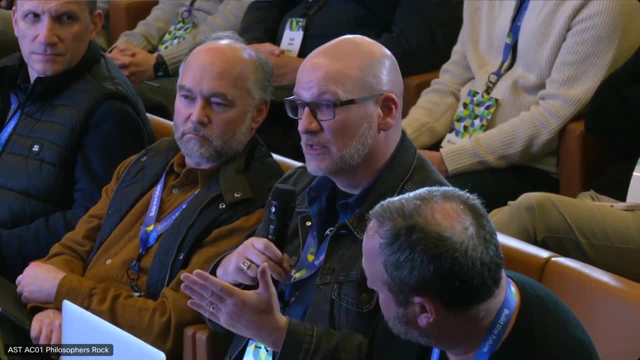 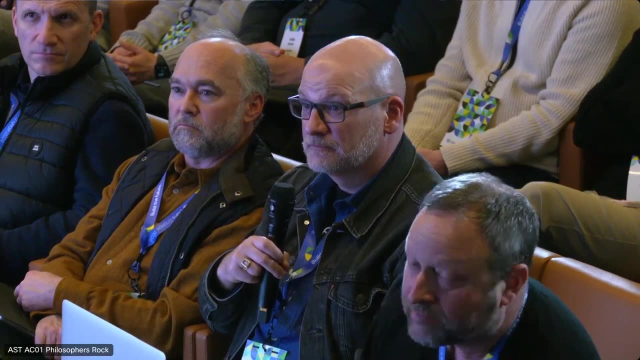 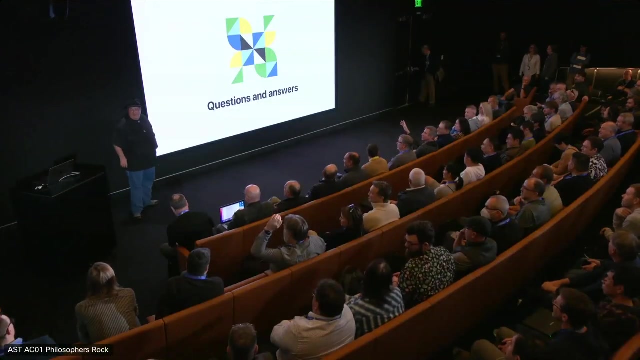 file cache size included as an option in the assisted install file, Please, Yeah, yeah, we yeah. that shouldn't be too hard to do. Yeah, Will the? will the Let's Encrypt refresh process require disconnecting users or restarting the database server? 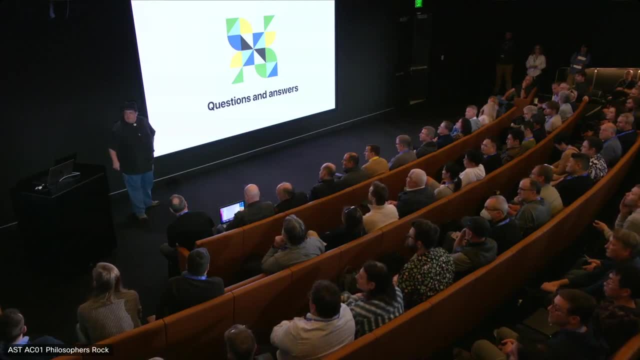 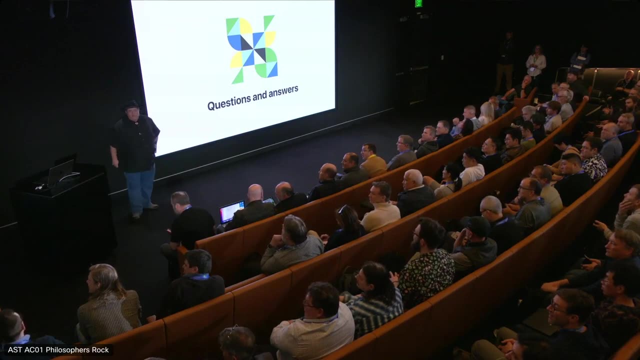 I believe it does at this point. Yeah, this first version will. As far as writing down that feature idea, could you repeat the question? Oh, whether Let's Encrypt when you refresh the certificate. when that script runs, it's gonna have to disconnect everyone and 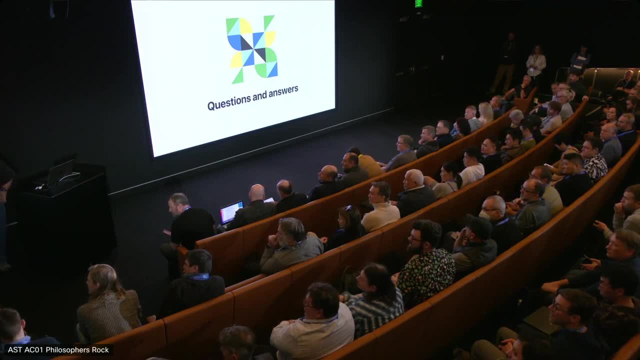 bring up the server again, right, Yeah, yeah. So we, we would love to find a way to maybe do a reload At this point. it's just a. it's just a restart. The thing is that we have to talk to the OmniOrb libraries. 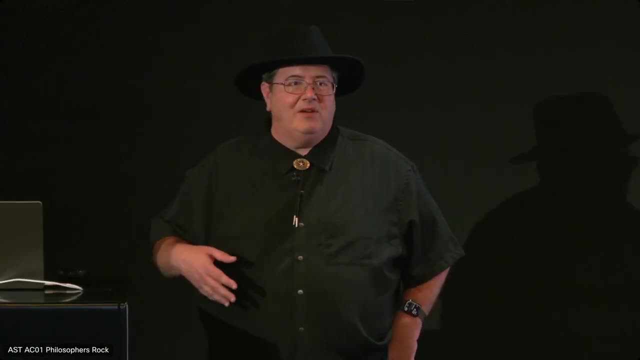 and stuff like that. We have some requests out to Duncan, the people that are updating They're working, or Asper saw, or the people that OmniOrb is an open source product that we have a yearly contract with to do updates and 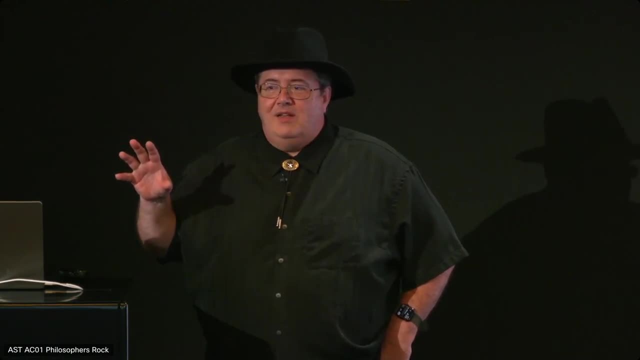 fixes and feature requests and stuff like that. Actually, when we started doing the HTTPS work, we were finding a lot of bugs that his other customers weren't Cuz we were hammering it a lot harder than a lot of his other customers. 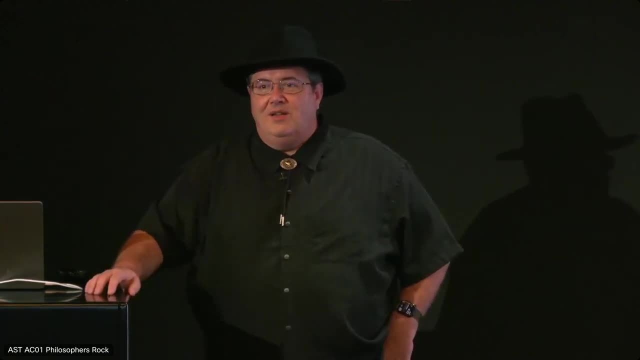 But he's very responsive to that And now that we have this new feature and now that we've stopped pestering him with HTTPS tunneling bugs that we can probably work on, have a mechanism to have their OmniOrb library restart. 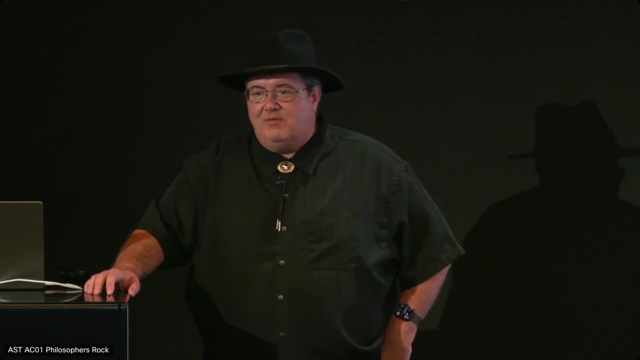 Or we start using a new certificate instead of having to force that stack to completely restart. I don't know. he may tell us that that's way too complex. I can't do that because there's too many threads running. I don't know, but we haven't had that full discussion with him. 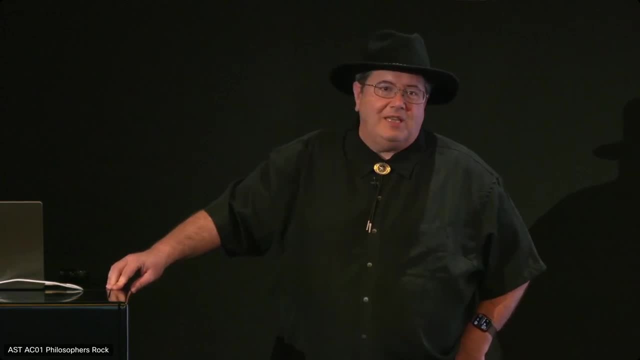 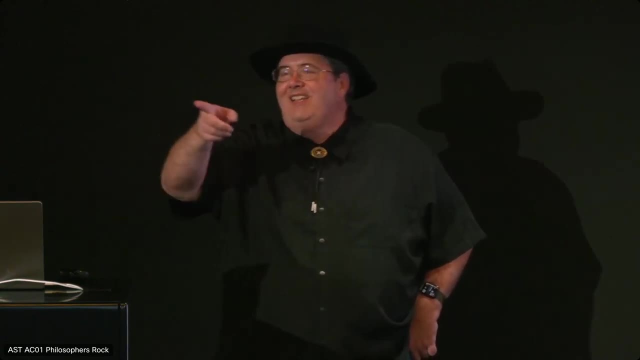 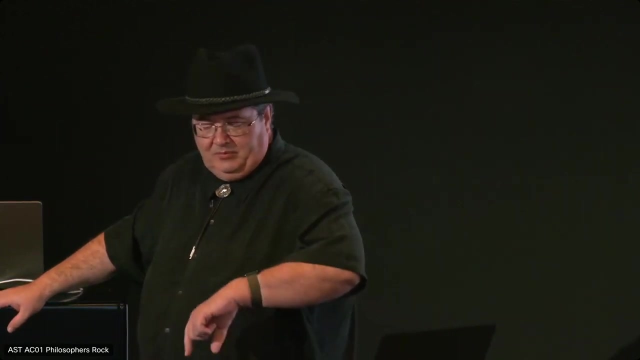 yet, But that'll be the work we have to do to get that to work, to upgrade the certificate without having to restart the server. We'll do you next after this. Thanks for sharing all the updates. Wondering if you can speak to roadmap for speed improvements. 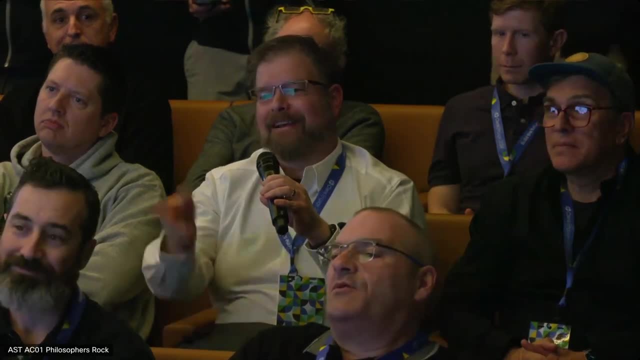 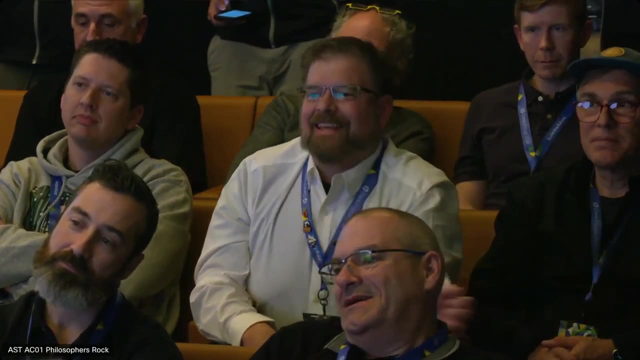 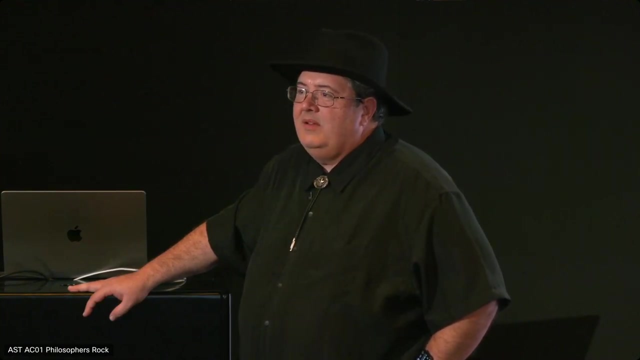 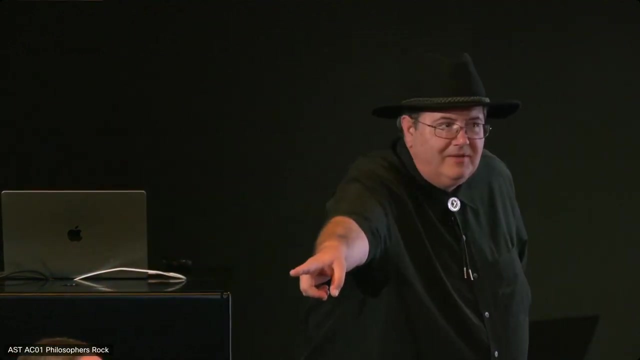 for the calc engine. Yeah, The L and M work is so. I think one of the things they've been talking about is doing this large vector math, And we were trying to do it with text first And over here, over here. 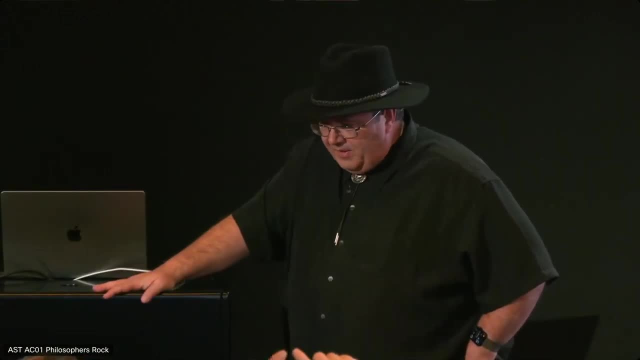 Yeah, And then we realized that, oh well, we need to really store a binary representation of that instead of the text representation, Because to do the math on that, you know converting it back and forth And that's kind of like the same problem with the JSON too. 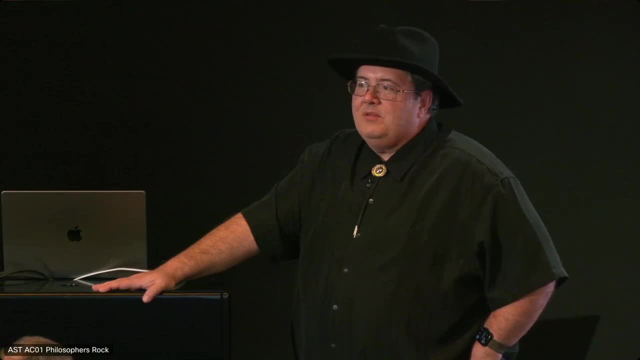 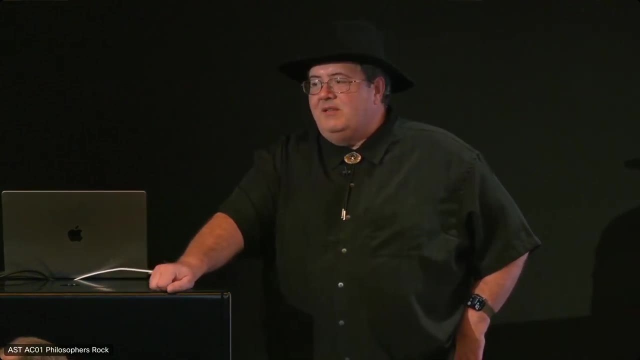 is that JSON is already stored as text And as it goes through the processing and stuff like that, it's getting converted to a binary form and back and forth all the time. So what they're playing with is basically putting the vector into a container field as binary data. 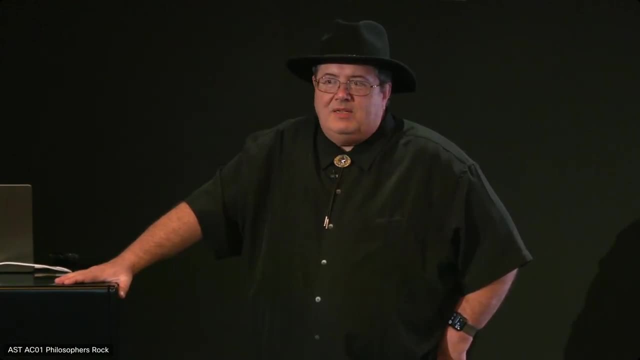 Ideally we would just add new data types. But to add new data types requires us really to have a file format. So how many of you guys would be really peeved if we did a file format change in the next three or four years? 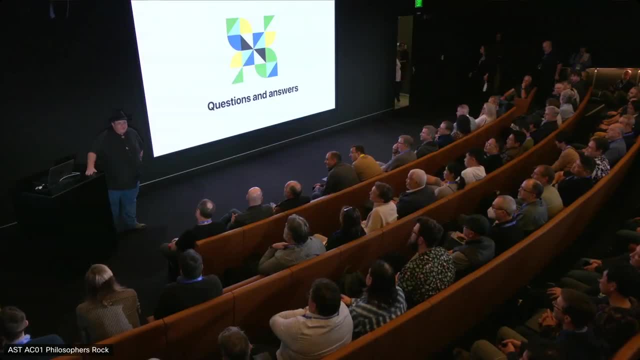 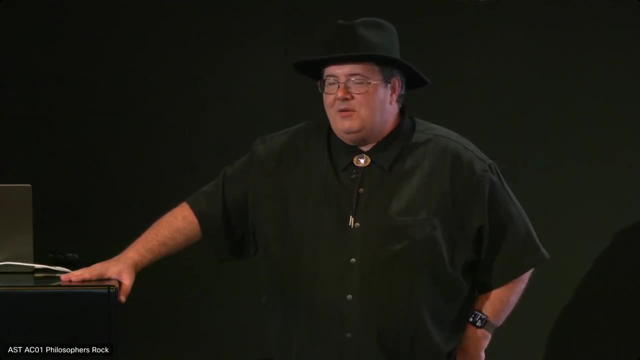 But- and that's one of the things that holds back some of these optimizations- It would really be nice to give some new data types internally that get pushed all the way through, But we're trying this out with the vector stuff using a container field. 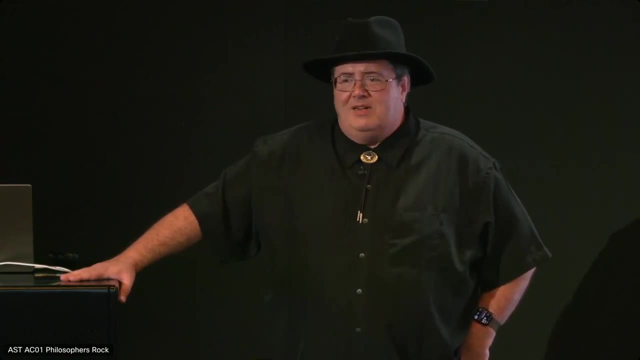 So it will be interesting. You'll be doing math in a container field saying that: oh, you know what's the cosine coefficient, What's the cosine coefficient of these two container fields, And then it will return you the value of how close the items in. 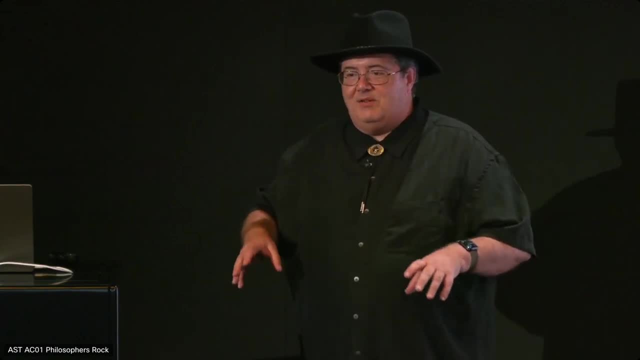 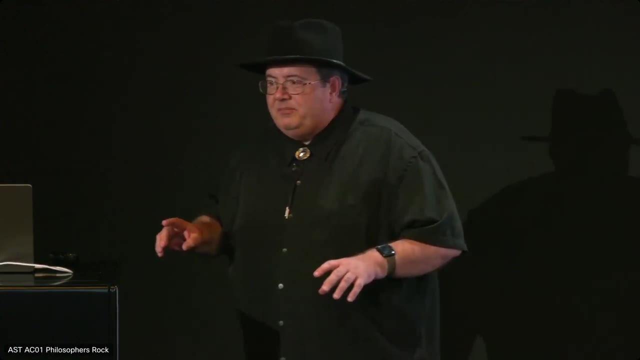 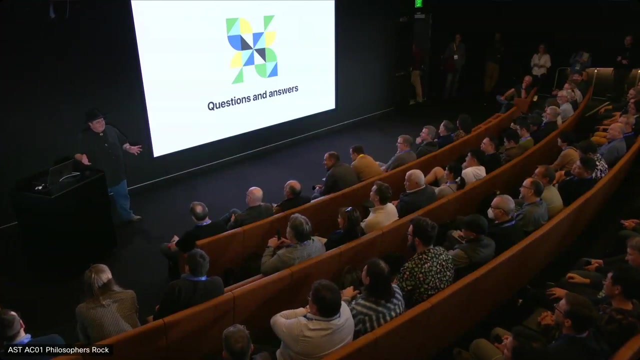 there are, whether they're related, whether they're exactly opposite or they're actually equal. You'll hear, okay, I have been listening a little bit about the L and M. Math is interesting, But yeah, they are doing work in there that we're kind of.